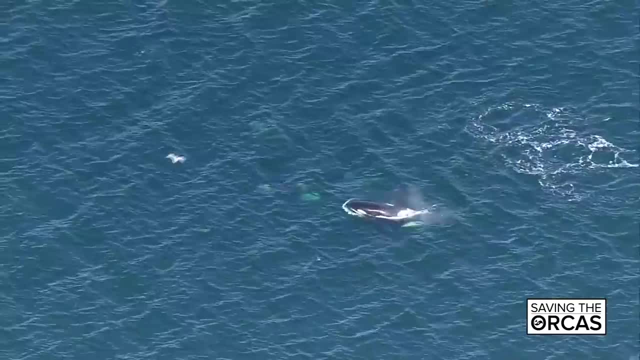 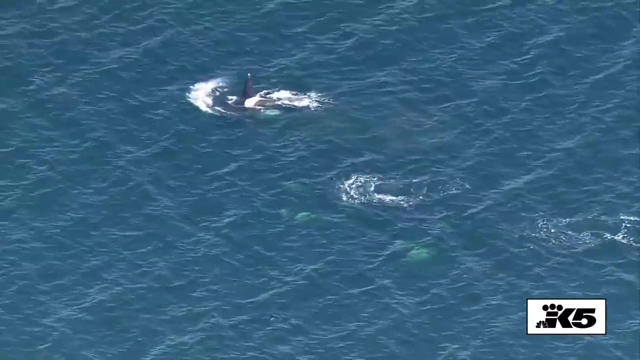 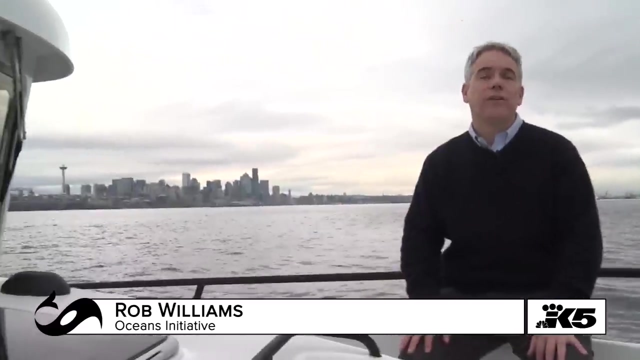 noise makes it hard for them to hunt. Killer whales, echo, locate their prey using sonar to find fish and capture it, as well as communicate with each other, and any loud noise can interrupt those signals. And what we're finding is that Harrow Strait and the Salish Sea is is noisy enough that whales are losing 62. 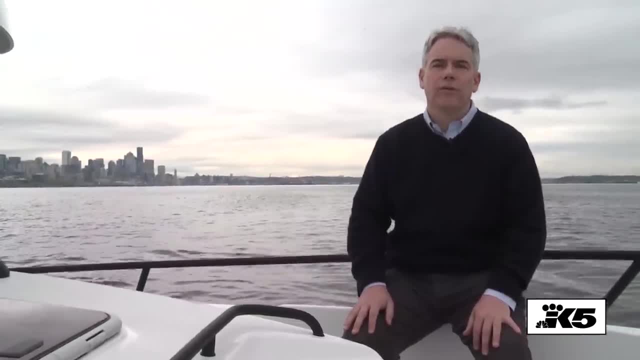 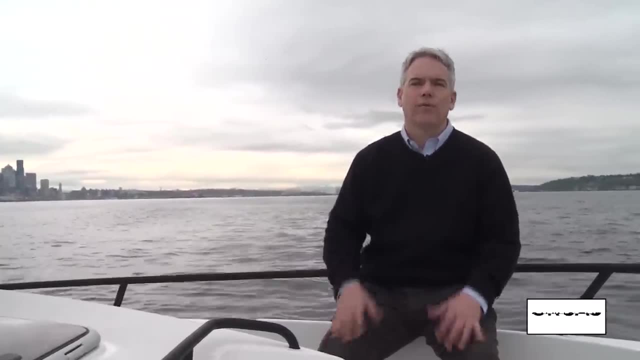 percent of their opportunities to communicate over the background noise on a typical day, and on a really busy day, they can actually lose up to 97 percent of their opportunities to communicate over meaningful ranges. Rob Williams founded Oceans Initiative and he's been studying the southern. 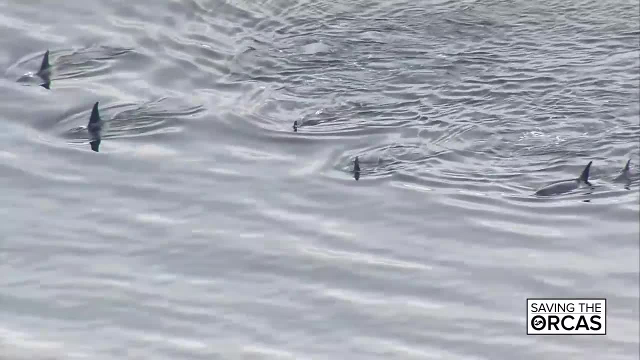 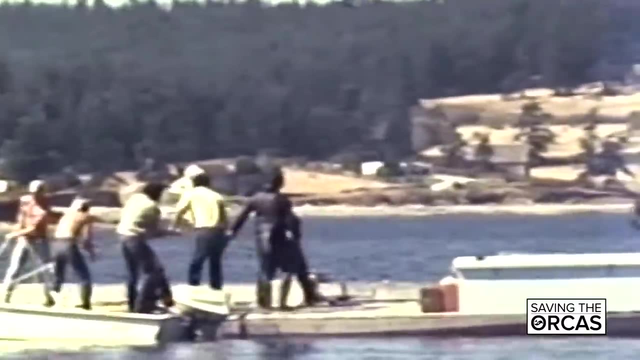 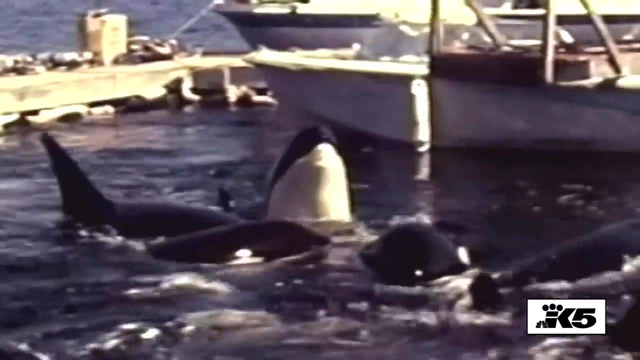 resident killer whale since 2003.. He says there's no easy fix. The problem started decades ago when captures for theme parks removed whales that could have reproduced and hurt the whales social dynamics. But since the captures stopped decades ago, the whales still aren't recovering the way they should. Williams. 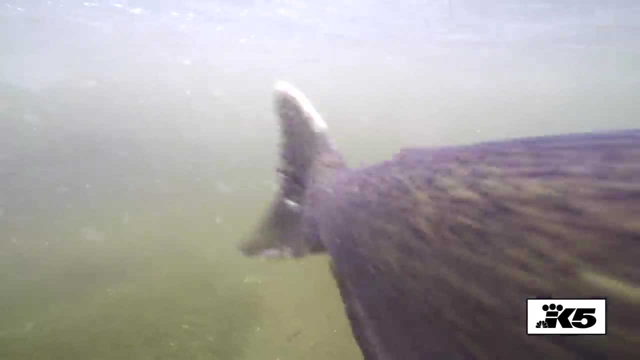 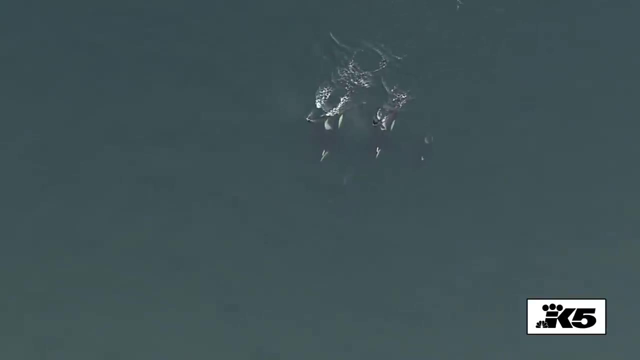 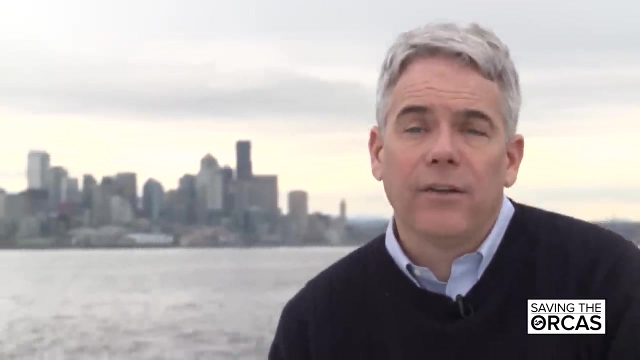 and other experts say that's because of polluted water, a lack of prey and boat noise. Williams says when boats are around, the whales can lose at least a quarter of their hunting opportunity. But we must not lose sight of the bigger picture, which is that noise can only bias and bias the whales. some time while we 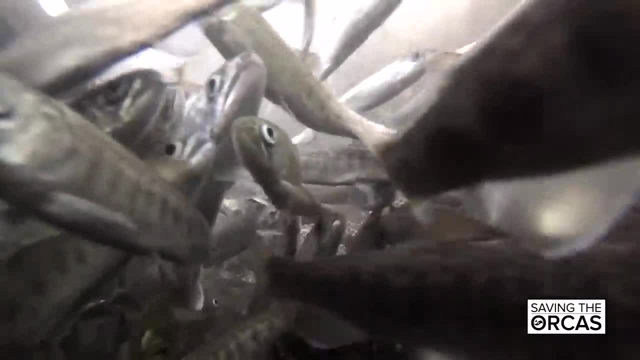 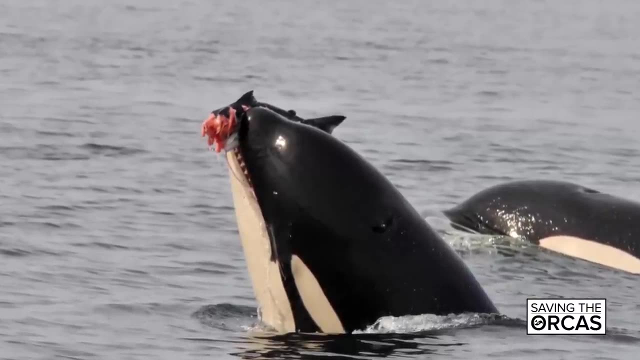 recover Chinook salmon stocks. Williams says that scientists estimate the whales need about a 30 percent increase in Chinook salmon numbers that haven't been seen since the 1980s. We've seen a lot of political will over the last few years to protect this population. 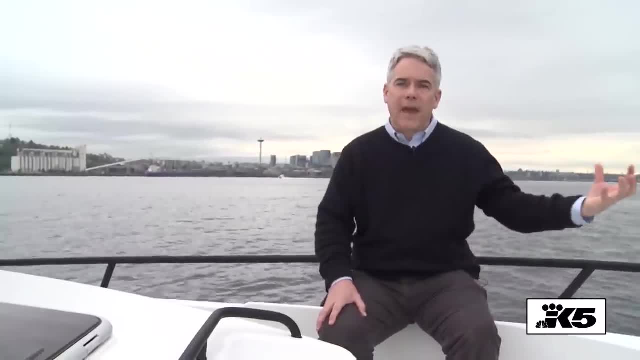 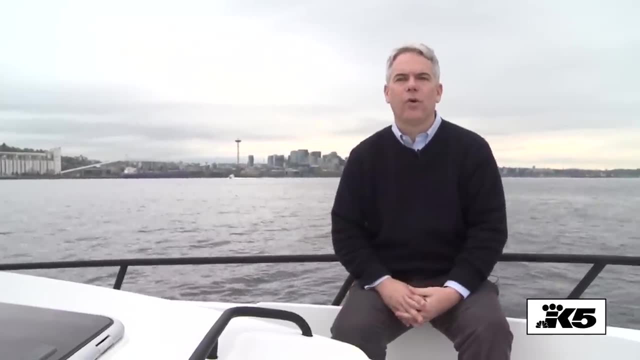 but we've also seen a lot of finger pointing: It's the salmon, it's this one dam, It's this one industry or this one source of noise and in fact, what our science is showing is that it's all of it and in fact we cannot get to the 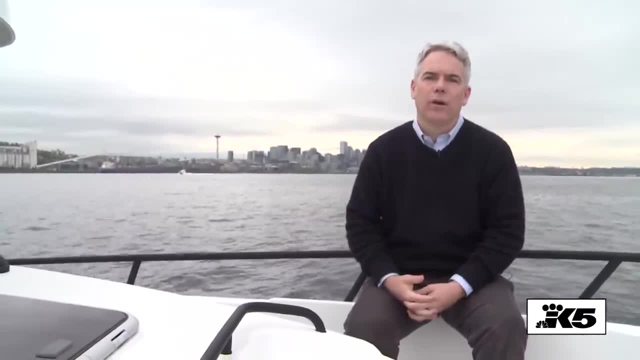 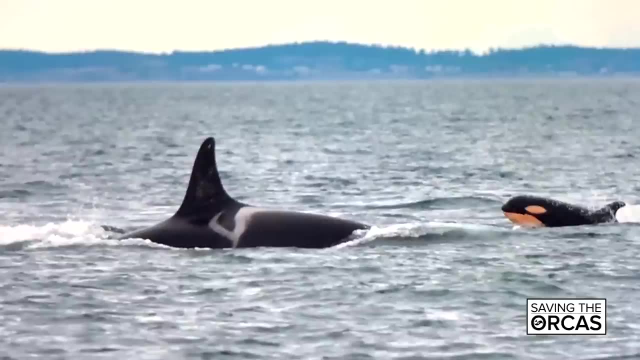 recovery target without mitigating all the threats all at once. One goal for recovery is helping the orcas birth at least one new calf each year for the next 10 years. but those calves also have to survive and the majority recently have died. These whales are: 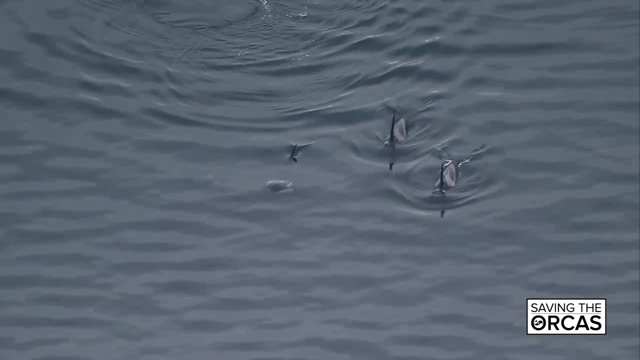 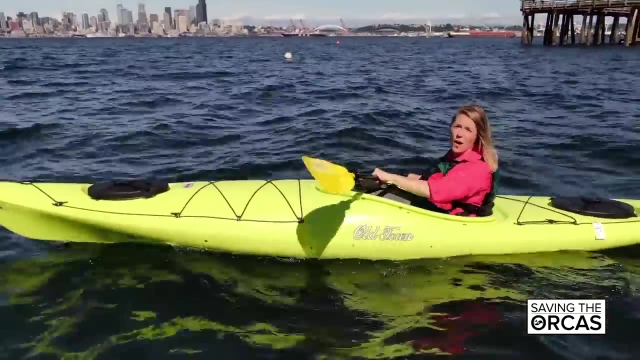 resilient and they're clever and if you give them a fighting chance they can recover. but we don't have a minute to waste. a lot of attention has been focused on the whale watch industry. in fact, the governor's task force to recover the southern resident killer whales proposed a ban on whale. 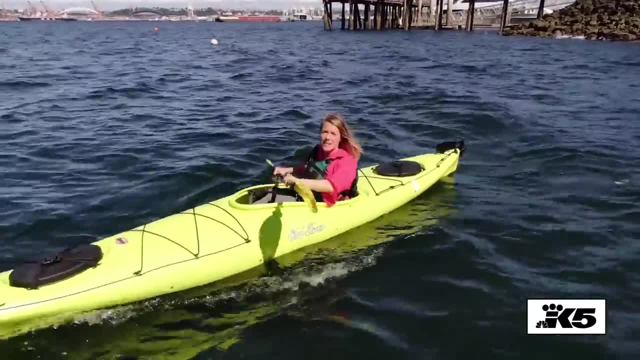 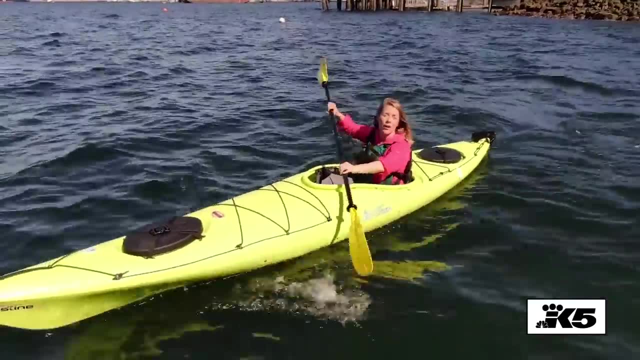 watching of these orcas, but legislators never passed it. some say that the whale watch boats add a considerable amount of stress to the orcas, while others say the whale watch industry is unfairly blamed. this group of high school students is in david bain's favorite kind of classroom. 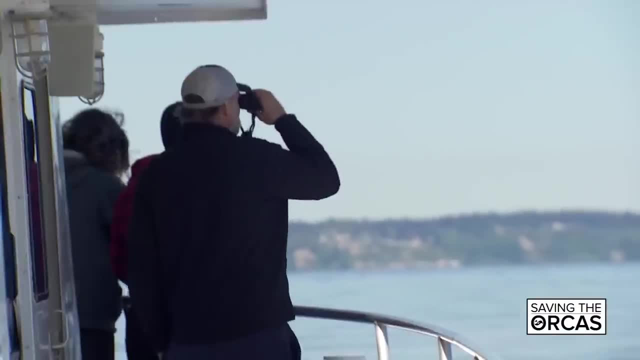 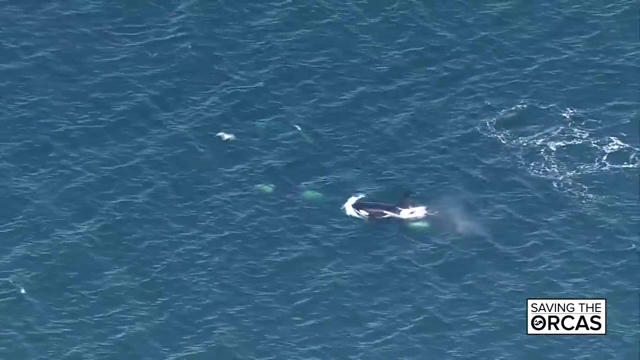 there's only so much you can get out of reading books. bain is an acoustic scientist who was once considered an adversary of whale watching boats like the one he's on. he studied the southern resident killer whales and his research prompted changes in the industry. the boats stay farther. 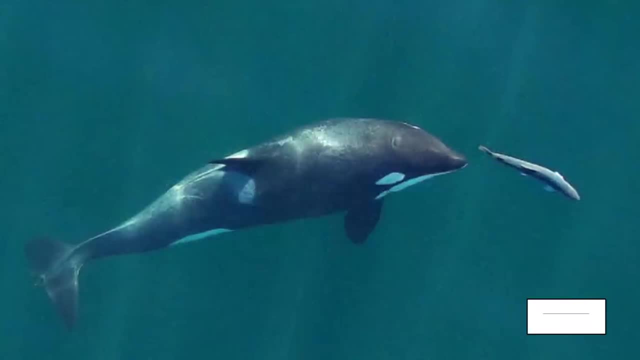 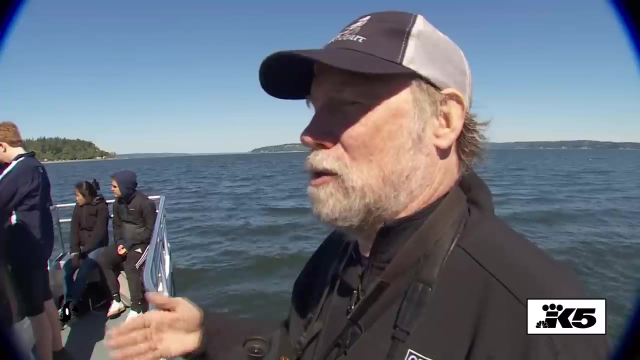 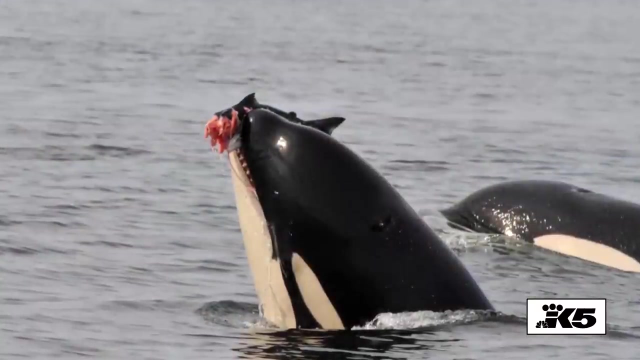 away and go slower so the whales can find their food. killer whales put out a click and they hear the echo coming back off the fish. as you can imagine, that echo coming back is very faint, so if there's too much noise they can't hear the echo. bain says scientists have found that when it's really loud the whales just give. 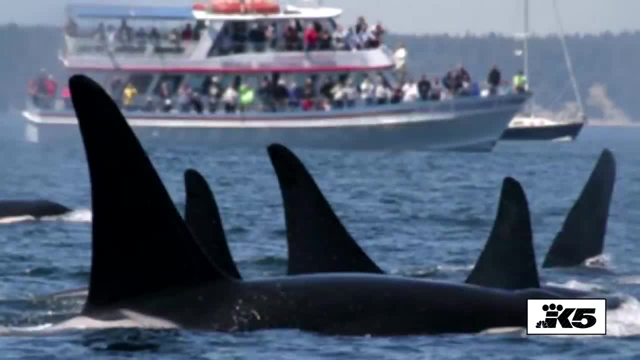 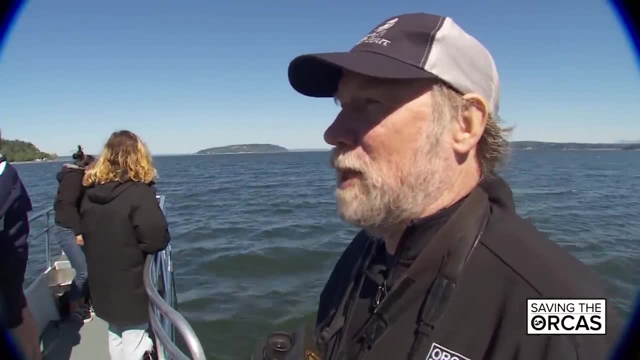 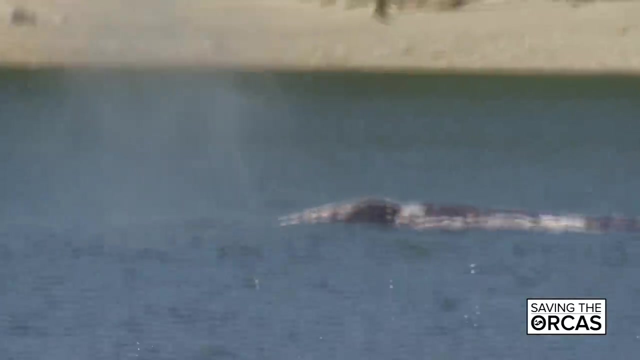 up looking for fish. but nowadays whale watch boats are not his biggest concern. the one i worry about most are small boats that are going fast and, you know, they may not even be aware the whales are there. boats like this one, which the whale watch boat tried to warn of the gray whales nearby we. 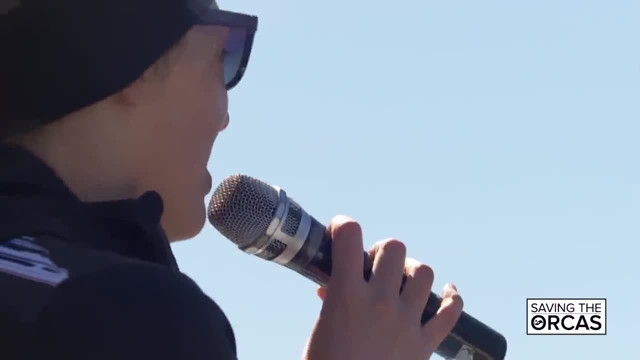 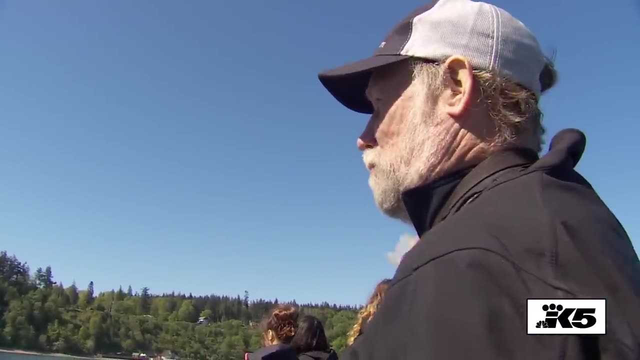 can see that the whale watch boat tried to warn of the gray whales, but it's clear that something was going on and he did not slow down at all and you can see his wake is right over there, near where those whales are feeding. even though that boat's off in the distance, it's still probably louder. 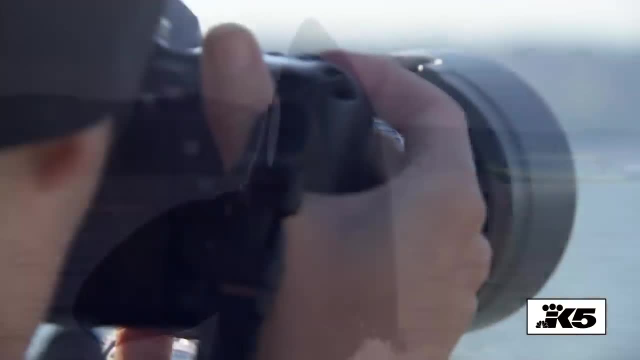 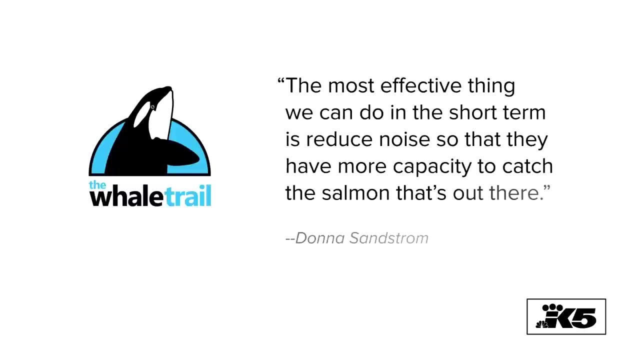 where the gray whales are than this boat is. but critics say that instead of warning smaller boats, the whale watch boats draw more attention to the whales by attracting other boats with people hoping to catch a sight of them. most effective thing we can do in the short term is reduce noise. 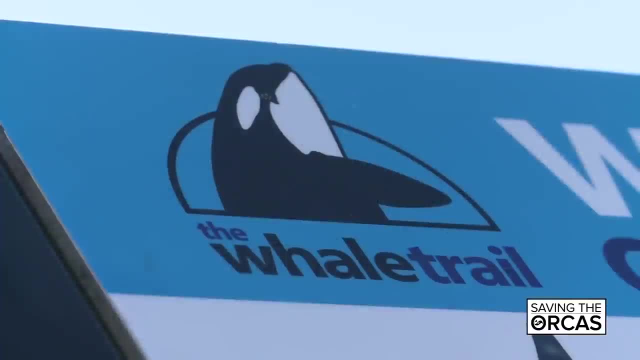 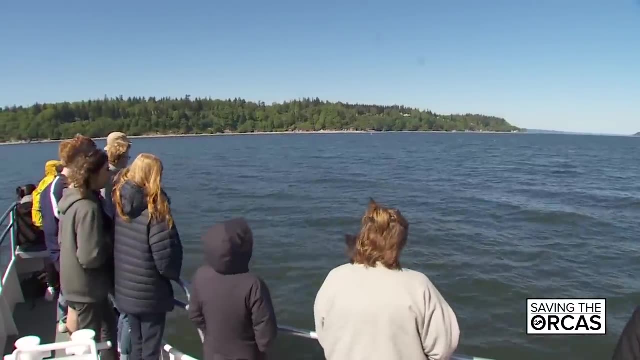 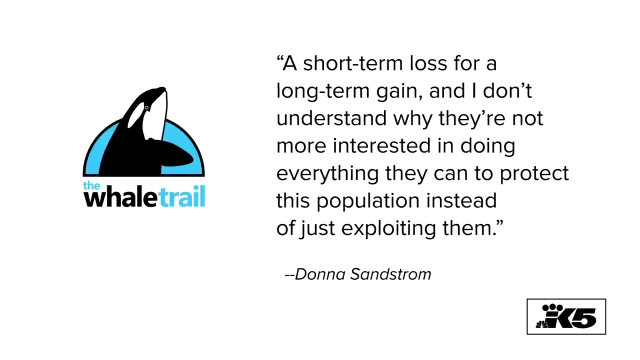 that's out there. donna sandstrom is founder of the whale trail, a land-based viewing option for whale watching. sandstrom was part of a movement to try to ban whale watch boats from following the southern resident killer whales. a short-term loss for a long-term gain and i i don't understand why. 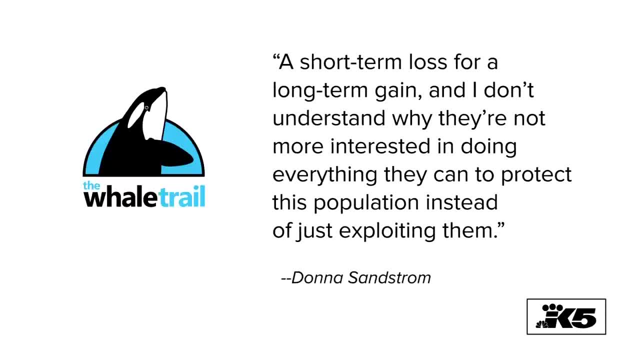 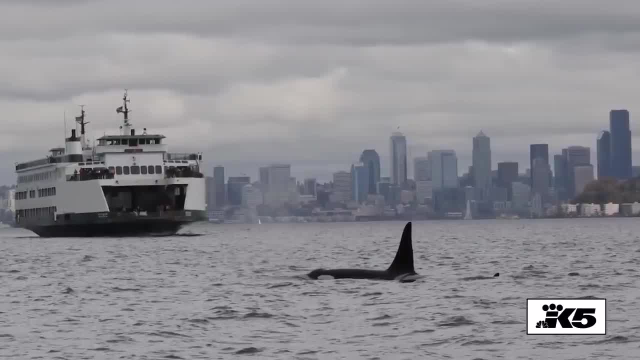 they're not more interested in doing everything they can to protect this population instead of just exploiting them? with all the different kinds of boat noise in the sailor sea. the whale watch boat is a boat that was originally singled out. can't argue the fact that we are out here on a 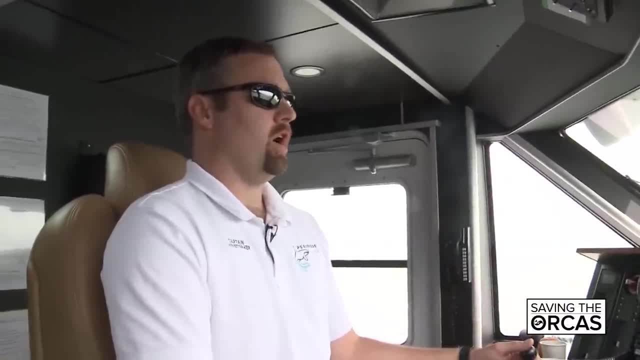 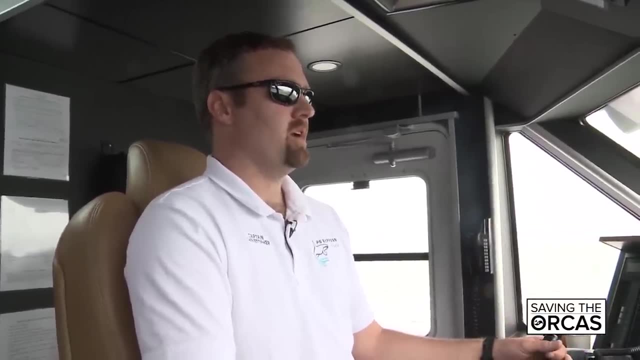 vessel. we are, you know, going through the water, creating noise. um, you know, i would argue our presence is mitigated by, you know, the education that we do. we, we're, in essence, the front line between the public and orca whales, and we're creating almost a relationship where people get 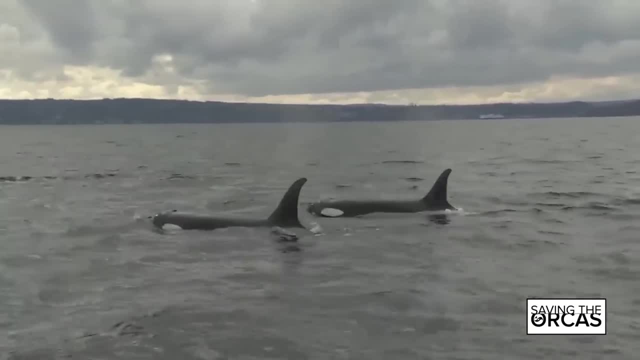 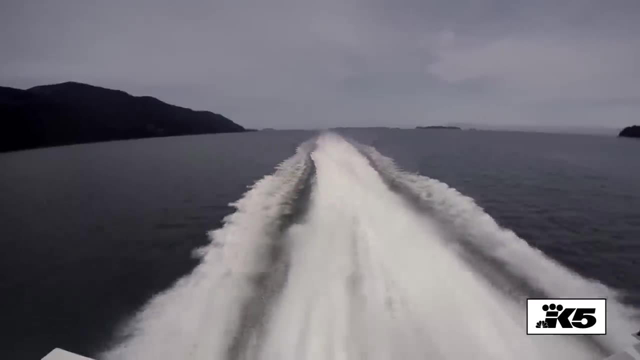 to go out and experience orcas and learn about the whales and the wildlife, and and you know ways they can help the whales. christopher hanky's family owns puget sound express and this boat has a technology that makes it one of the fastest but also one of the quietest in the pacific whale. 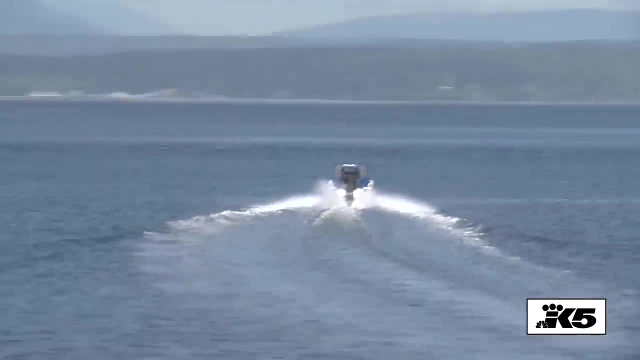 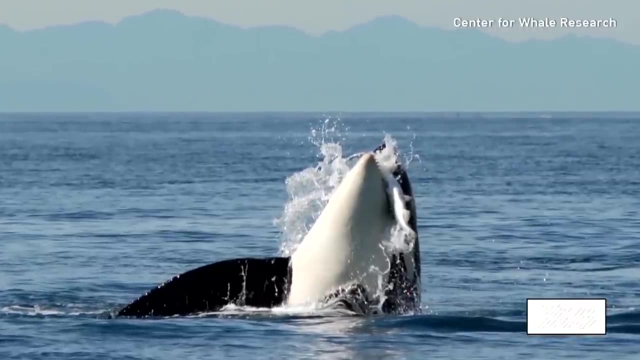 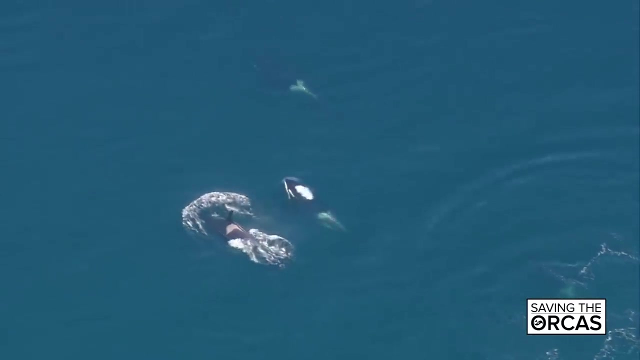 watch association. like many others, he says noise is an issue because there are so few salmon for the southern resident killer whales to locate. i think the orca whales are part of the salmon story and i think the biggest hope for everybody is that we can restore salmon habitat and maintain you. 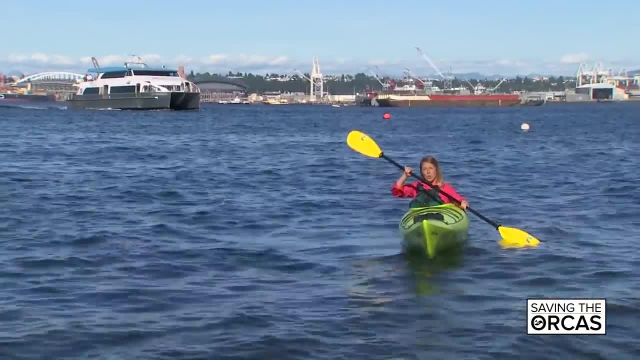 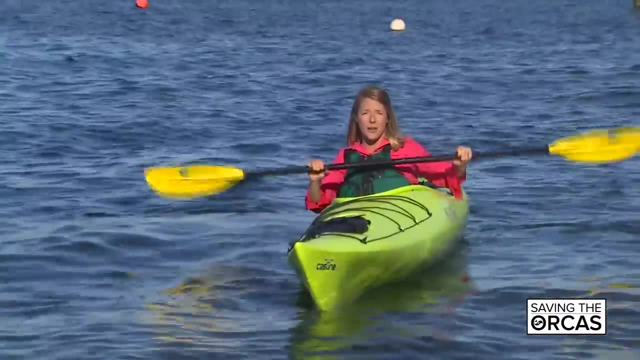 know our native salmon species. boaters should expect to see more law enforcement on the water this summer, especially off the coast of the mont island, which is one of the favorite places the southern resident killer whales look for food. the rules for voters have changed this year, and wildlife police officers will be out enforcing them. 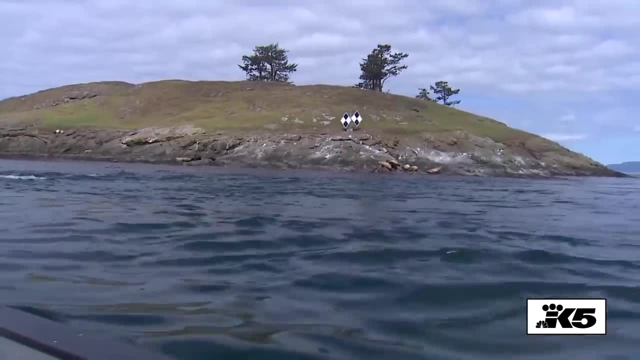 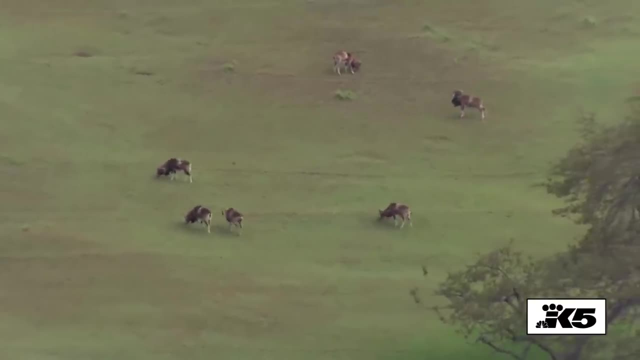 we never really know what we're going to see out here on a given day. some days we'll see stellar sea lions, some days we'll see different birds, deer and and such on the islands, but most of the time we're looking for marine mammals. like the southern residents, life is about to get busier. 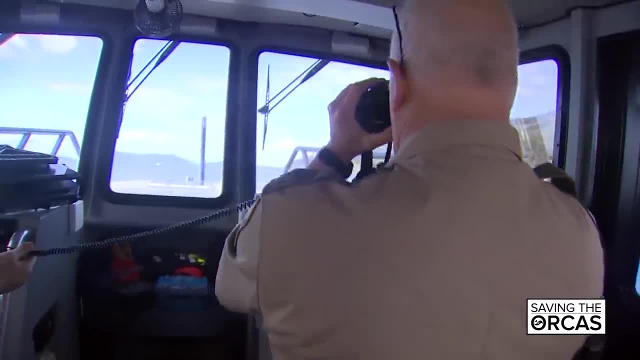 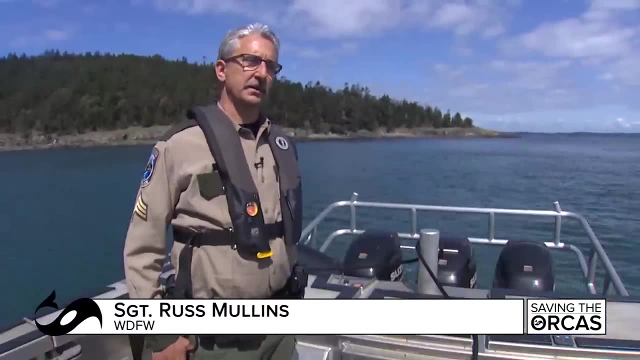 with the state wildlife police team. looks like a tadbit as there looks like a tour boat. as the weather gets nicer and more people are out on the water, they plan to be there as well. having vessels get too close to the killer whale has been a problem for quite some time. 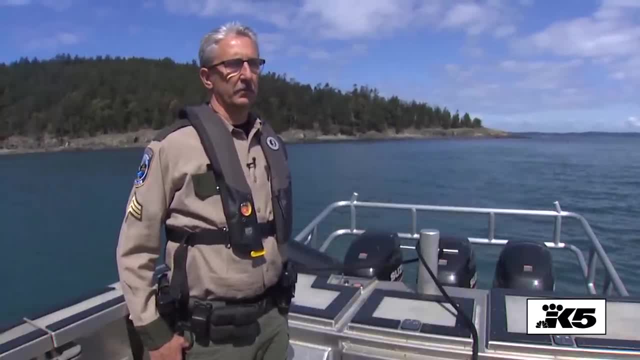 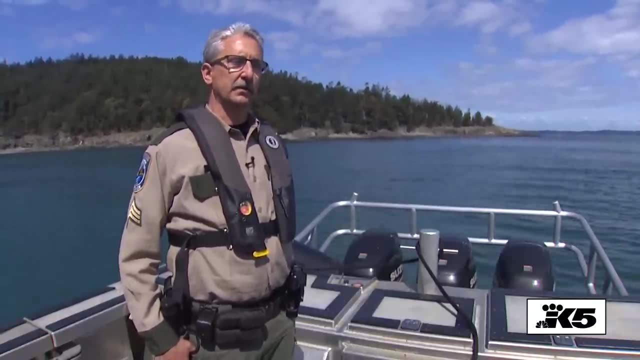 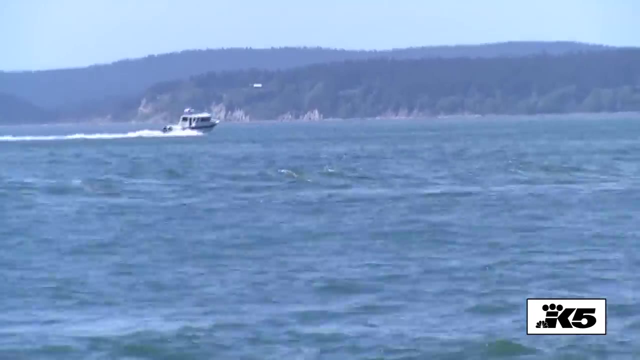 we worry about, in a worse case scenario, prop strikes, which haven't been known to happen, but we always worry about it, and also the cumulative noise of vessels being in close proximity to the whales. sergeant russ mullen says officers with the washington department of fish and are mostly focused on operators of recreational boats and fishing boats. 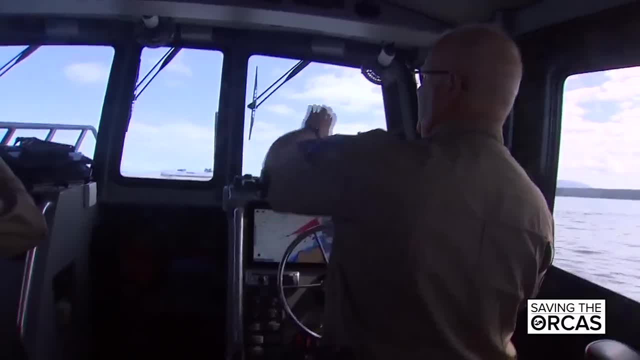 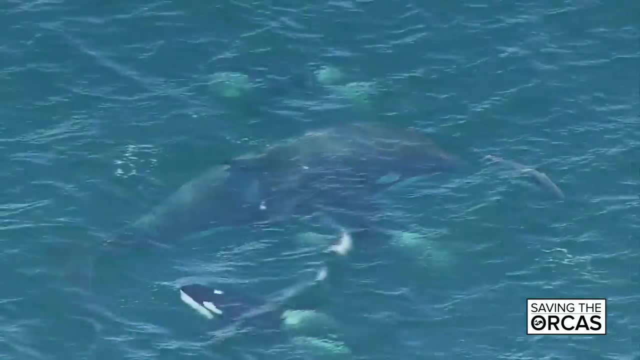 who may not be aware, there are whales around them. It looks like they're looking off the port bow. Boat noise hurts the orcas' ability to hunt because they use echolocation to find fish and that echo is drowned out by boats. Quiet is so important for the endangered orcas. 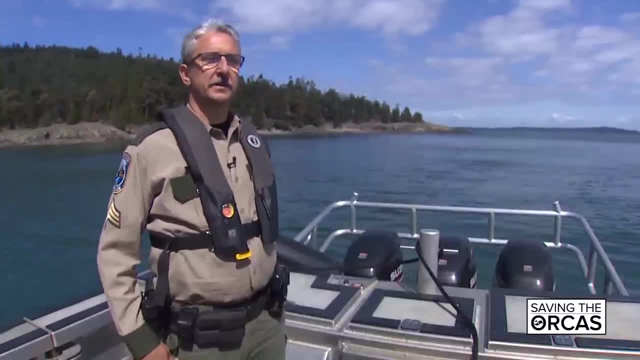 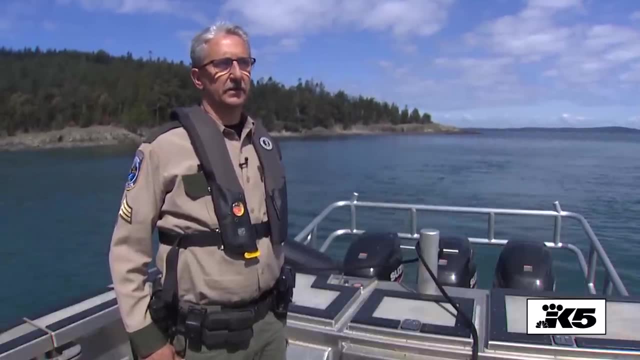 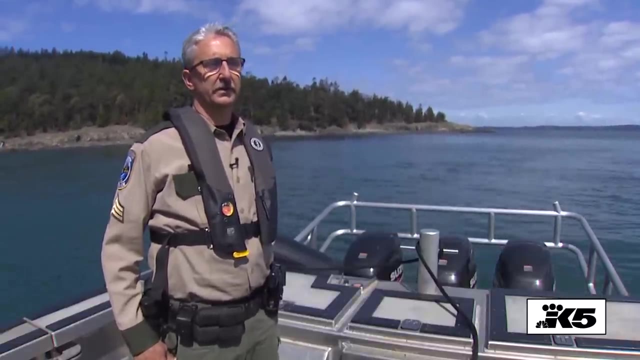 that state law is now changing to protect them. The changes to the existing law are going to be the addition of a one-half nautical mile go-slow zone around southern resident killer whales, as well as expanding the no-go perimeter around the whales from 200 to 300 yards on the sides. 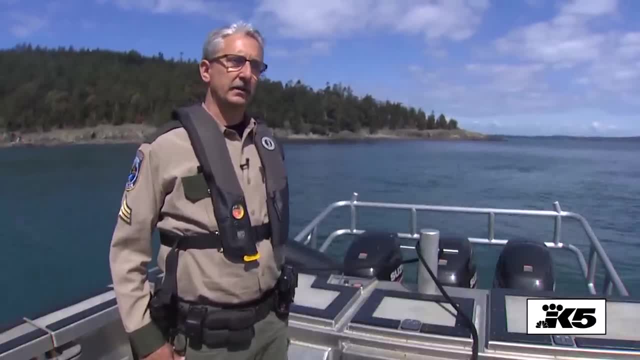 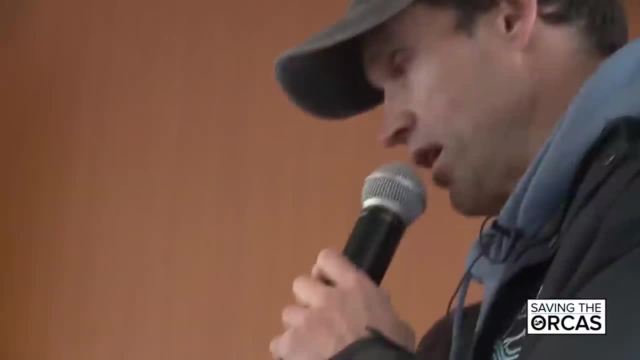 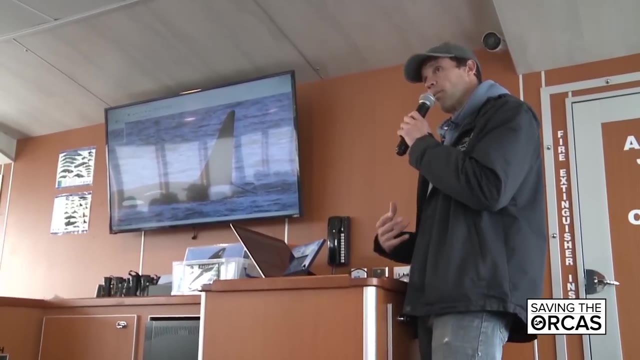 and 400 yards in front and behind the killer whales. if they're traveling, Boaters could face fines, but Sgt Mullen says they prefer education. These orcas can travel all the way from southern California to southeast California- Education like what naturalist Bart Rulon does on this whale-watching boat. 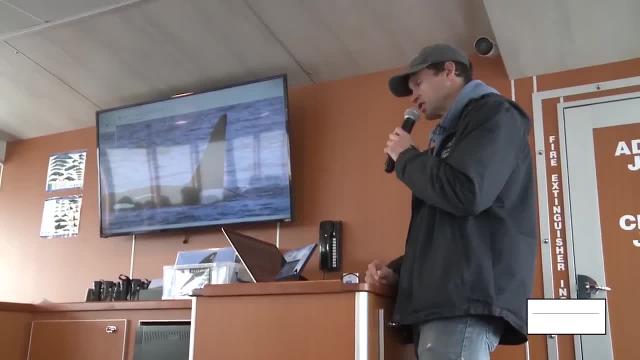 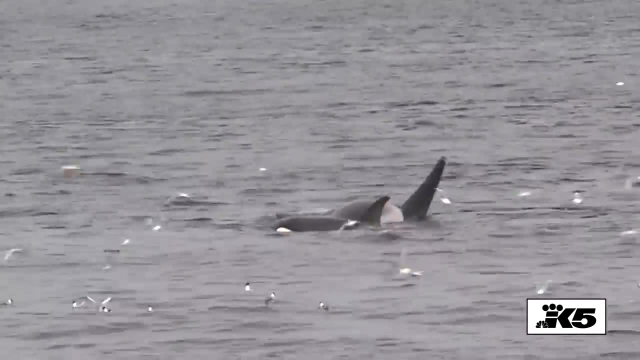 The cornerstone of orca research and other whale research is being able to identify individual animals. While we were with him near Orcas Island, we saw transient killer whales hunting a sea lion. Rulon captured photos that show the orcas in action. 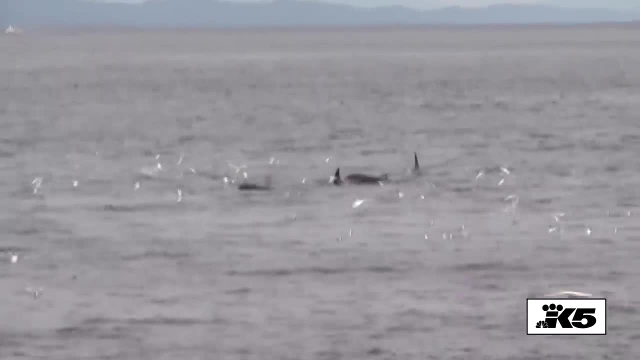 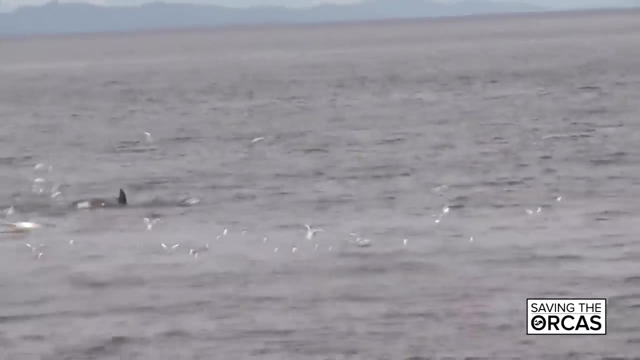 Transient killer whales eat marine mammals and have plenty of food, which is why boat noise is not as much of an issue for them and why Rulon has seen a lot more of these orcas. It's also why he says they've seen less of the southern residents. 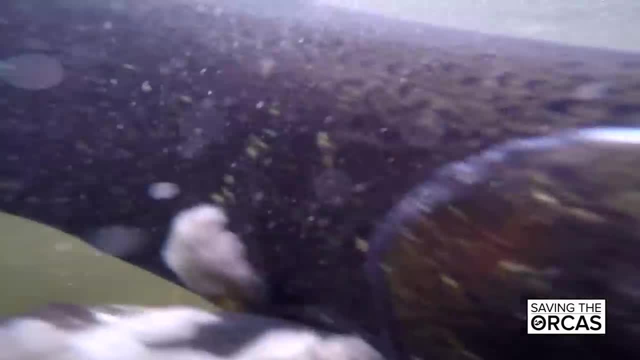 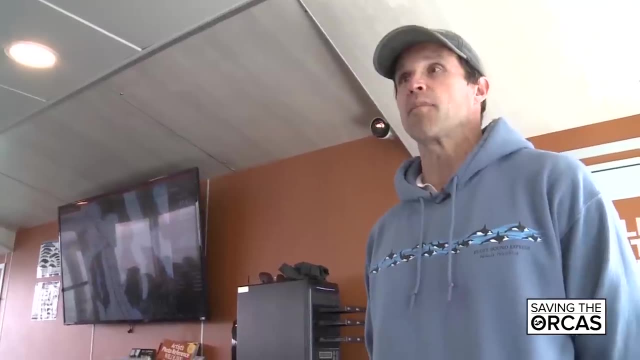 who only eat fish almost exclusively- Chinook salmon- that are also dwindling in number. It's all about the food with these orcas. That's what the residents need. They need more salmon And that's what these transients are benefiting about right now. 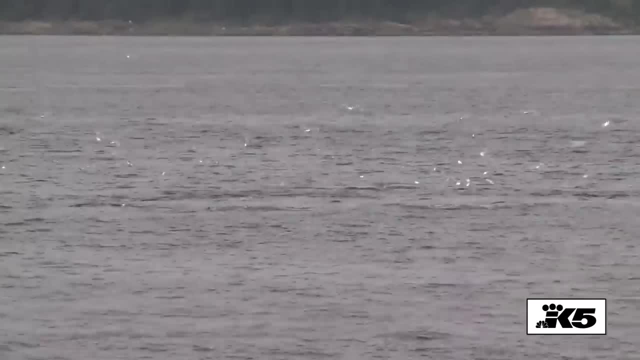 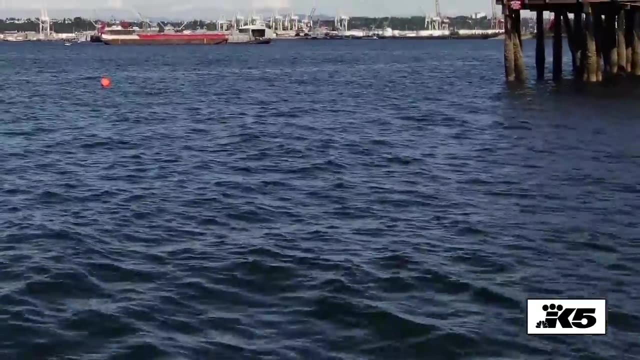 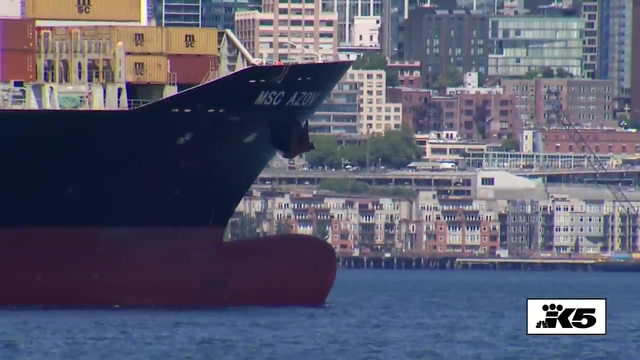 It's amazing how much more we see the transients. So just how noisy is it underwater, And how do scientists measure that? Well, one group has placed hydrofoils underwater recording devices around Puget Sound, And all of us can listen to them live online. 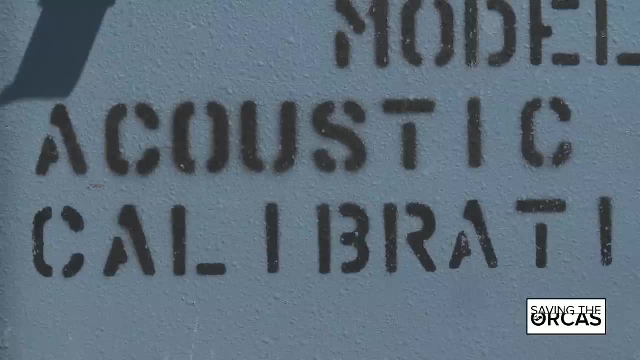 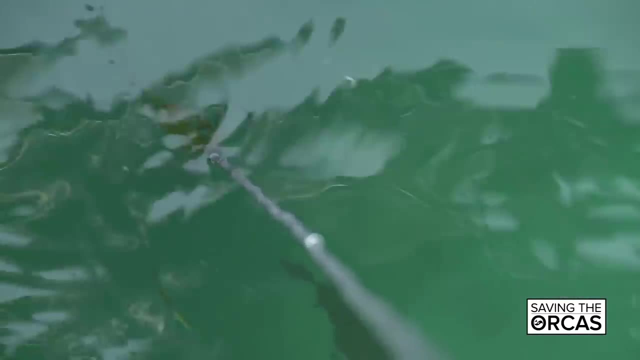 as the boats are moving through. We're on the Edmonds Pier fishing pier and I've got a hydrophone, an underwater microphone, dangling down here like a fishing line. This is one of the areas the southern resident killer whales often visit when they come to Puget Sound. 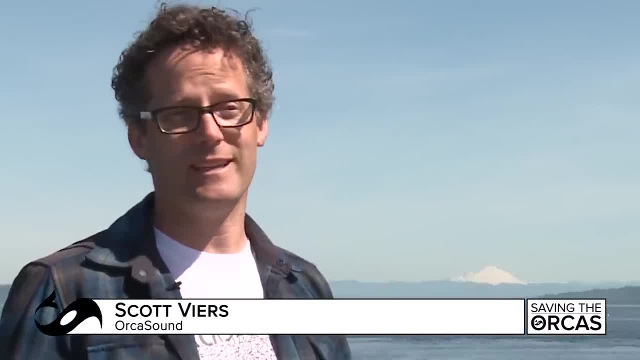 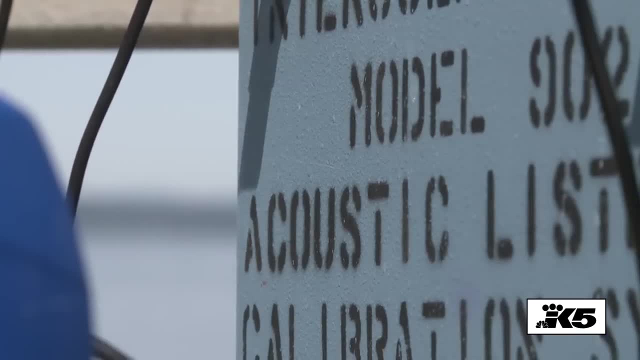 We have killer whales who are acoustic specialists, living basically in the shipping lanes. Scott Beers is coordinator of Orca Sound's hydrophone network. The underwater acoustic monitoring system has shown just how noisy it is when the southern residents come here looking for food. 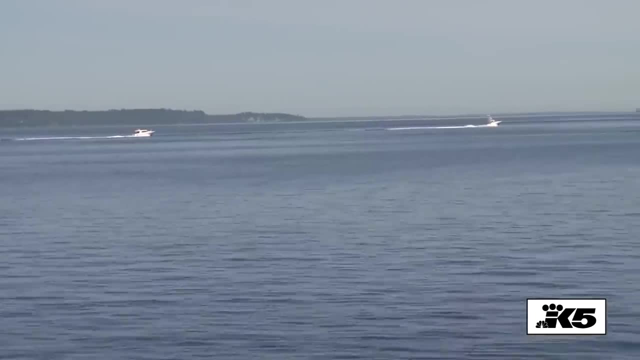 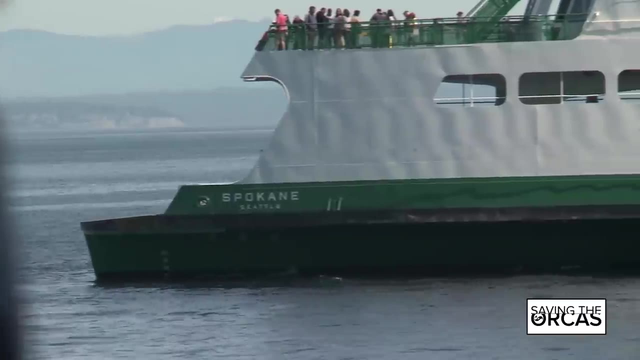 Noise comes in lots of variety: Small recreational boats, big cargo ships and, of course, the ferry system. You can see the ferries leaving the dock now. The noise level is increasing, So now we're above 130 decibels. 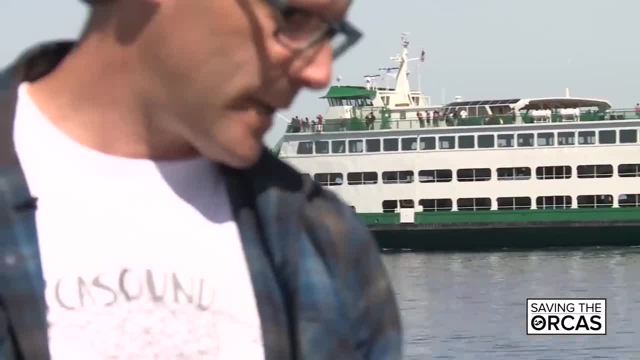 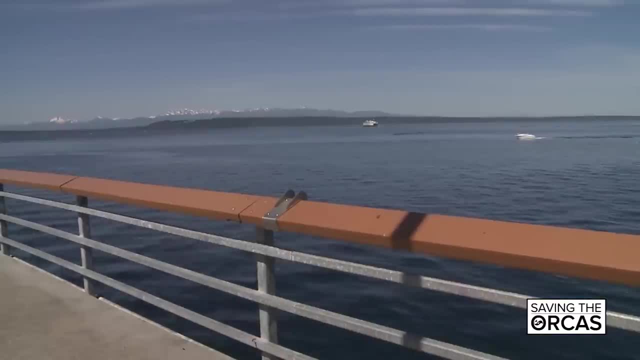 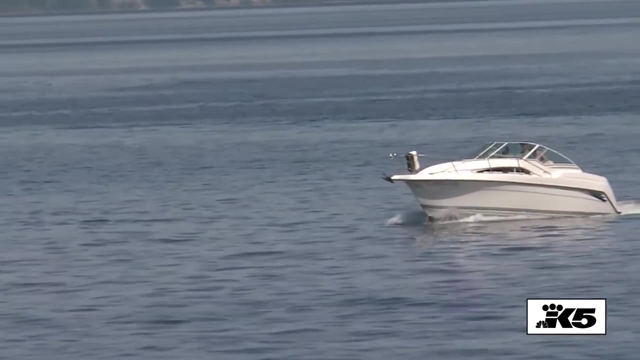 Now it's more than 133.. So now we're at 136.. Plus they don't just contend with one boat at a time. It's sort of the lower frequency chugging of the distant ferry and then a higher buzz from this powerboat probably. 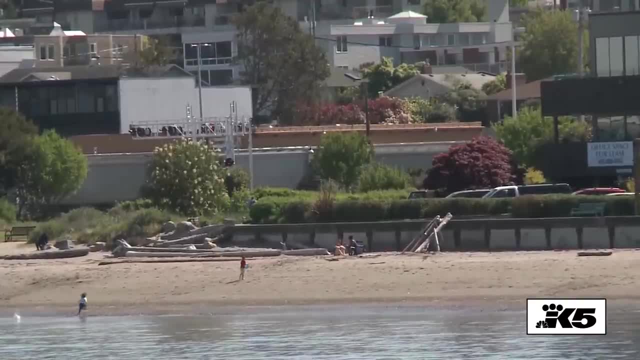 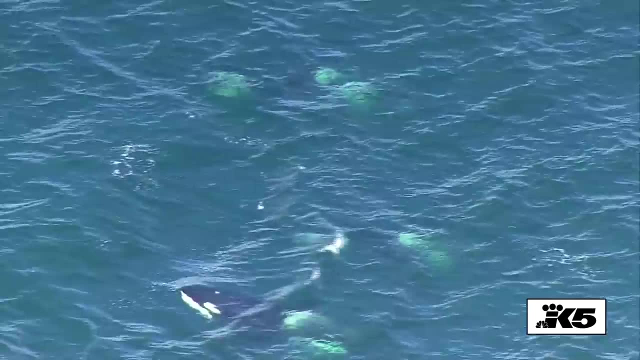 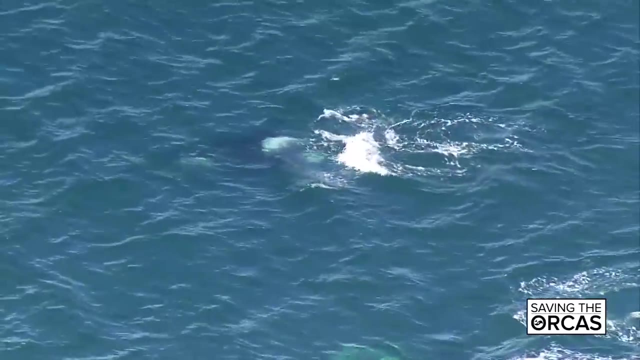 Now add: in a train, I automatically make my voice a little louder so that you can hear me over the train whistle. Just like us, the orcas have to talk louder too, which may cause stress. Sometimes it's so noisy they just give up looking for food. 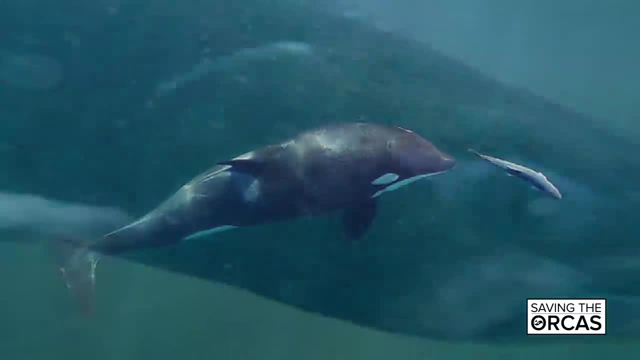 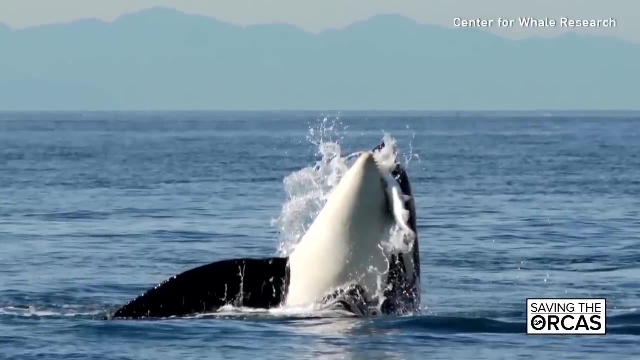 Their preferred prey, Chinook salmon, are decreasing in number and much harder to find than a few decades ago, And that's why quiet is so important. The easy thing to do to increase access to salmon is reduce noise. He says quieting that traffic will make a big difference. 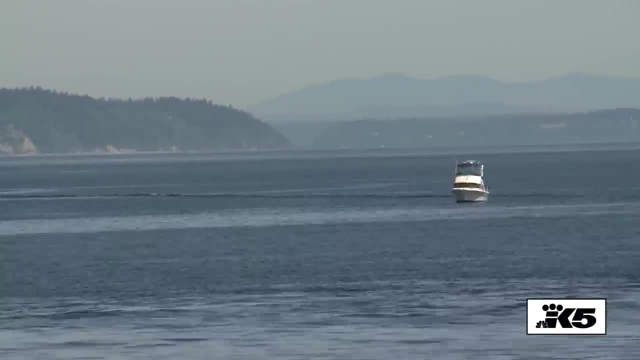 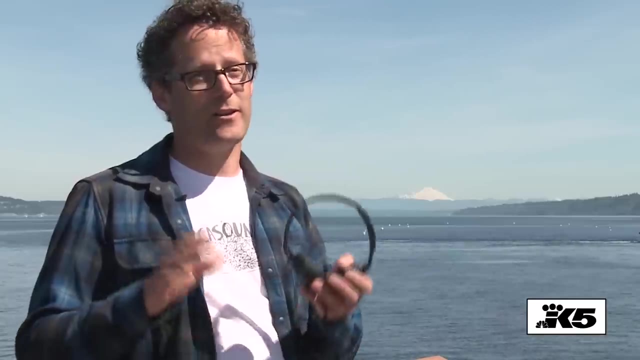 Once you start turning the propeller in a way that causes this thing called cavitation. cavitation makes this really high frequency hissing sound. That's important for the killer. It's important for the whales because they're high-frequency specialists and they click at frequencies that are well above what we can hear. 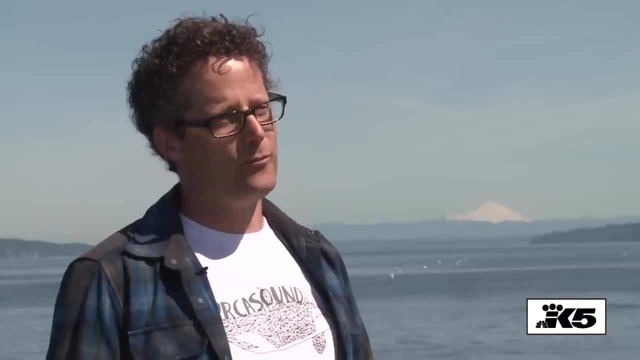 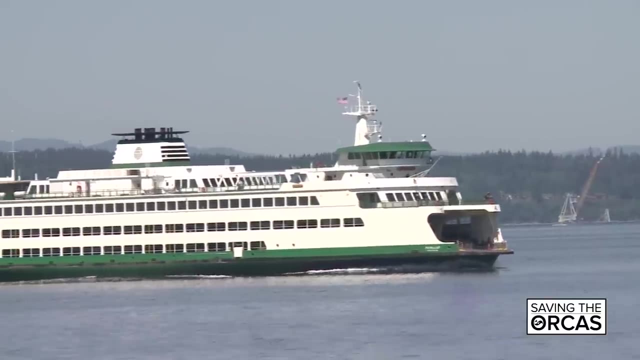 Anything you can do to keep a propeller from cavitating will be helpful to the whales. You're starting to hear the Kingston ferry coming in For Veers. all the other problems are still important to fix, like salmon habitat recovery and reducing pollution. 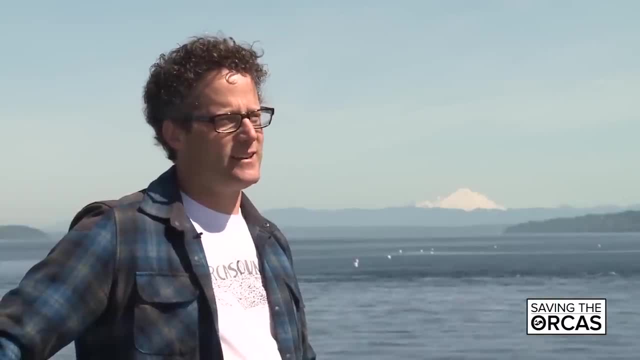 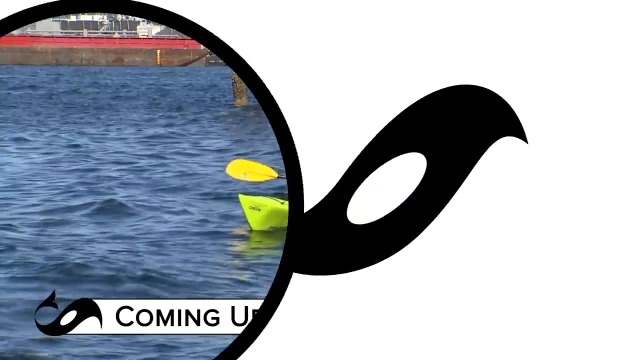 The good news about noise in the ocean is that if you remove the source or you quiet it, it's going to go away. Pollution is poisoning the southern resident killer whales Coming up. we'll tell you where it's coming from and what's being done to clean it up. 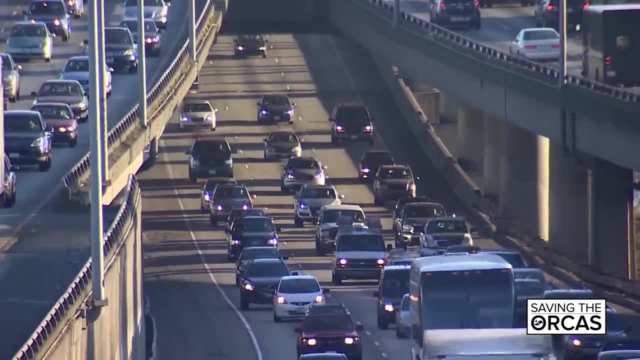 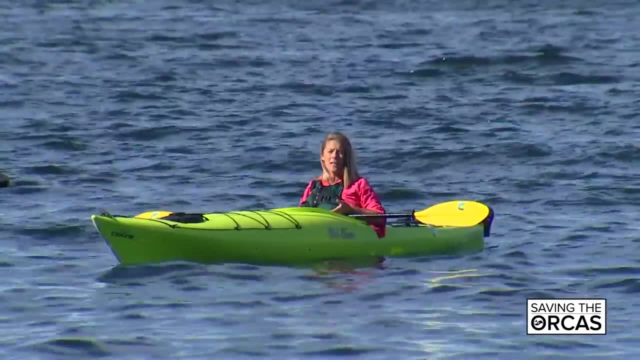 Every time we drive down the road, our cars leave behind tiny particles of pollution from our brakes, our tires and the exhaust, And when it rains, that pollution flows into Puget Sound and builds up in the fat stores of the southern resident killer whales. 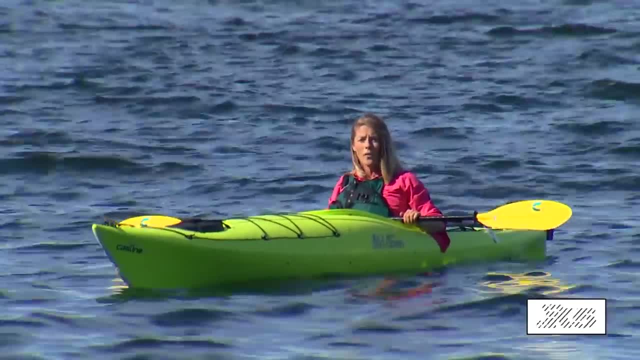 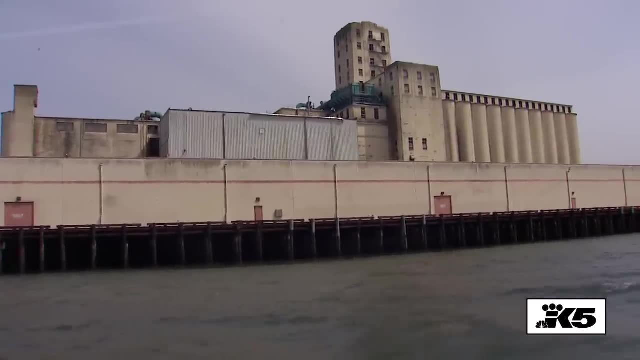 But the roads are not the only problem. Seattle's working waterfront is also a challenge. You can see all the creosote pilings that are there. They're still leaching toxics into our waters, Whether it's these toxic wood pilings or chemicals leaching. 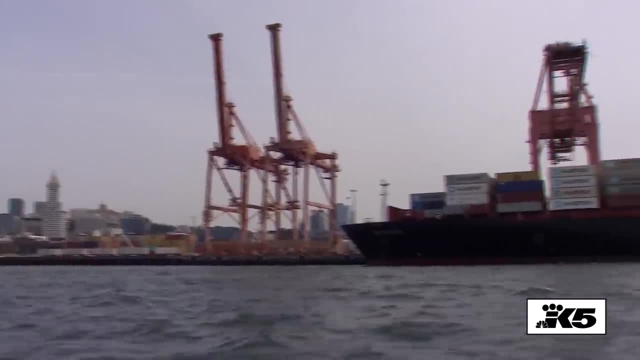 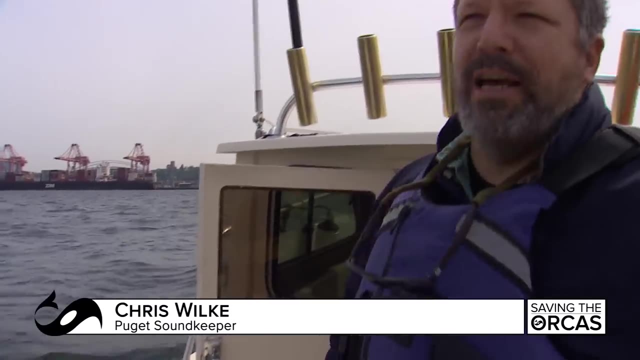 from a scrap metal recycling facility. Seattle's working waterfront is a focus for Puget Soundkeeper. When a lot of people think of stormwater, they think of roadways and parking lots and rooftops and things like that, But it's also industrial sites. 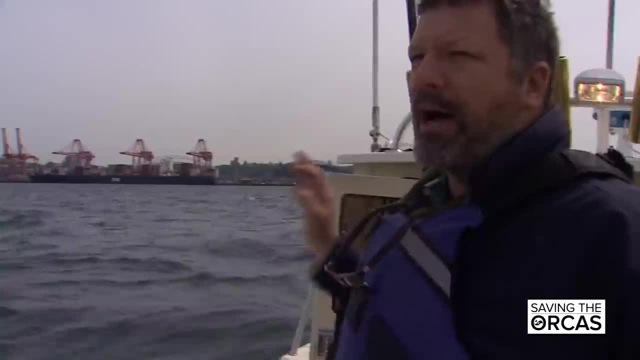 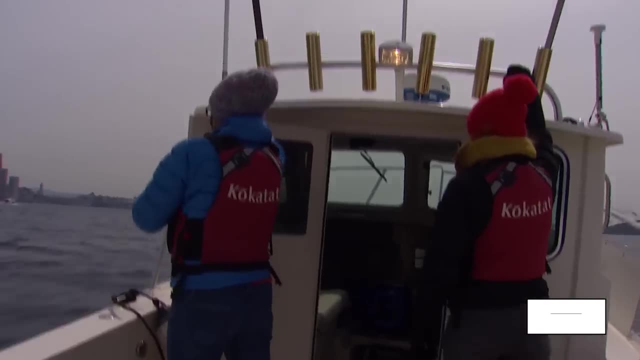 And so this site over here and some of the ones behind me over here have been out of compliance with their stormwater permit. Chris Wilke is executive director of the nonprofit that investigates water polluters, focused here on contaminants that can have lethal effects on marine life. 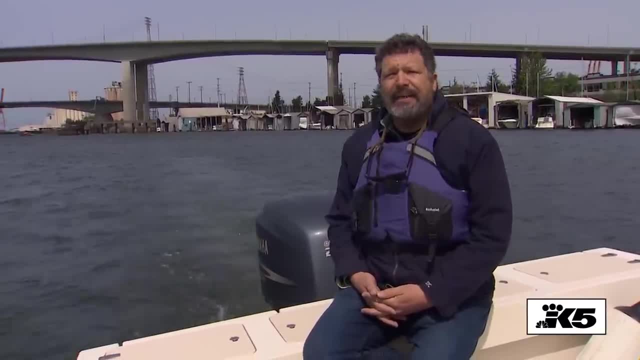 There are chemicals like PCBs, lead, copper and zinc at very high levels that are not safe for marine life. They're not safe for marine life. There are chemicals like PCBs, lead, copper and zinc at very high levels that are not safe for marine life. 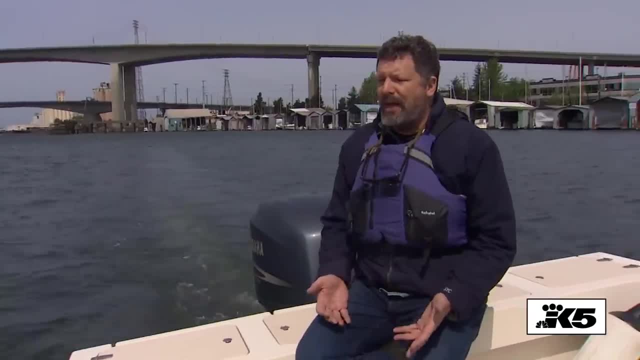 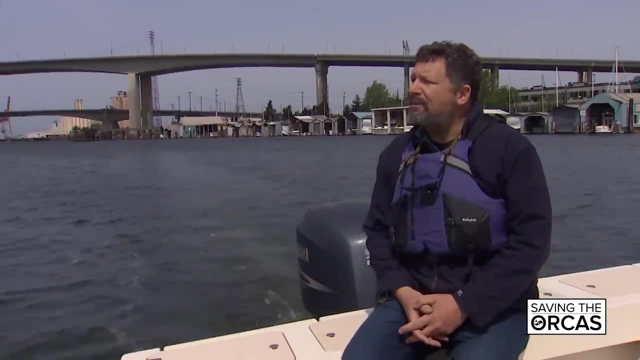 One of the key measures of that is whether or not it's safe to eat the fish, And we are going by right here, to the right of the boat, is a public fishing pier that has signs on it in eight language. that's saying it's not safe to eat the fish. 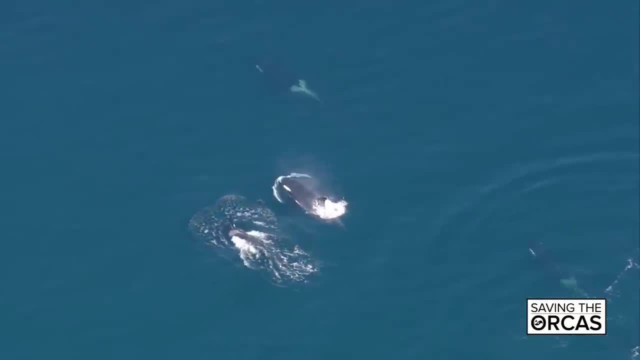 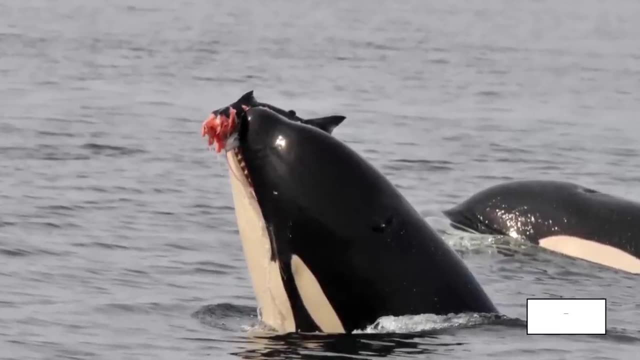 The Southern Resident Killer Whales are often called some of the most contaminated marine mammals on earth. Their fat is filled with toxics like PCBs, And when they don't have enough to eat, they metabolize that fat and that poison ends up in their blood. 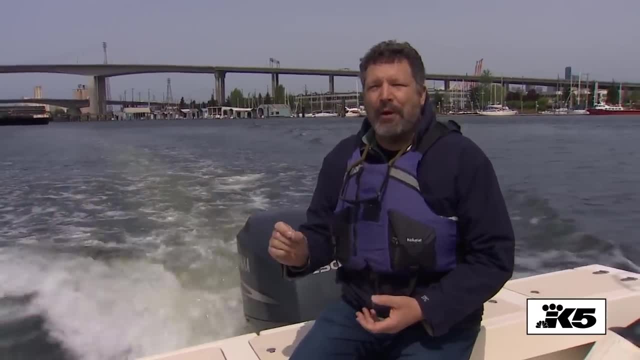 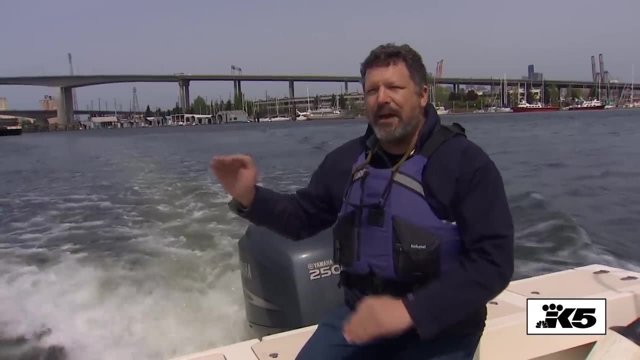 Start with the small micro-element, All microscopic organisms, and then tiny shrimp-like zooplankton, on up to herring, on up to salmon and then on up to orcas and people And every step of that food chain those pollutants accumulate into eventually. 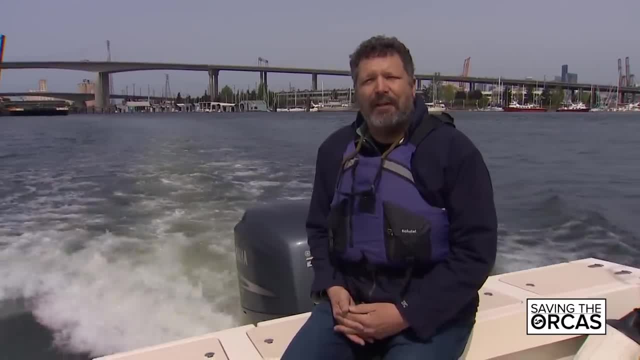 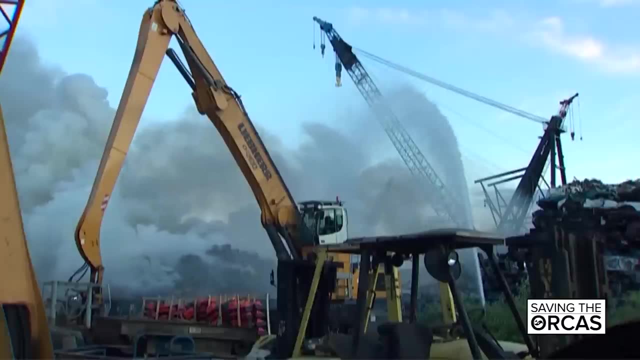 by the time you get to an orca whale. it's extremely unhealthy for the animal, But it's even unhealthy for the salmon and the herring as well. Here at Seattle Iron and Metals, a fire last year caused even more concern. Puget Soundkeeper recently reached a million dollar settlement. 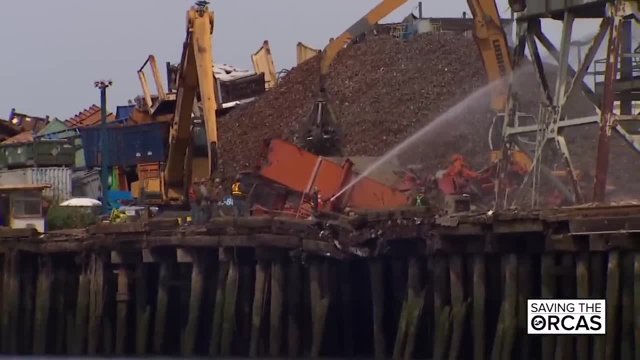 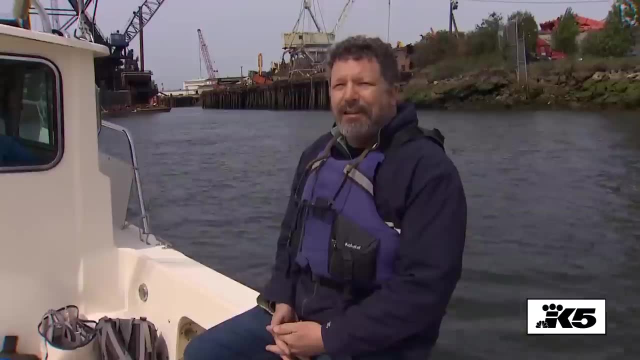 with the auto recycler, forcing them to make changes to protect the waterway. Wilkie says they're celebrating but also critical of all the battles they have to fight And the state is really not living up to their mandate- A lot of the toxic contamination issues that we have. 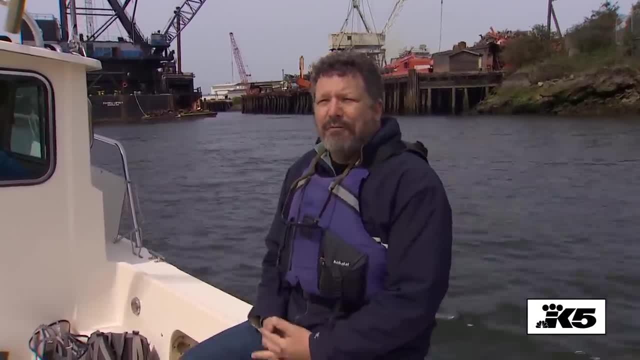 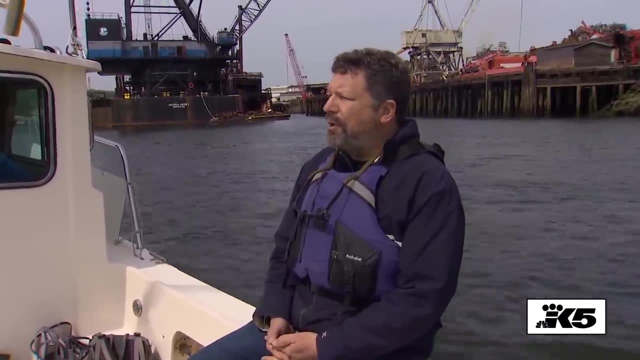 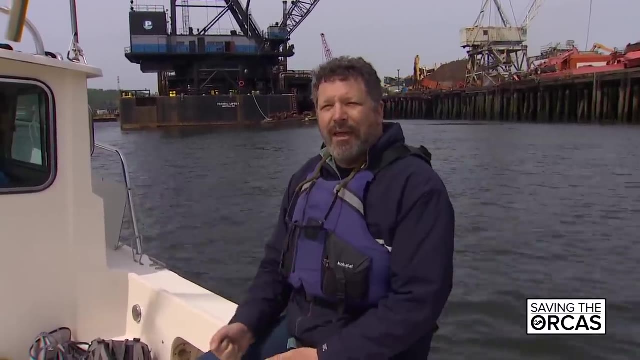 with our salmon and our orcas can really be traced to the fact that the state of Washington is not enforcing the Clean Water Act to the extent that they should, And when citizen groups like ours are able to step up and force industries into compliance, that's a good thing. 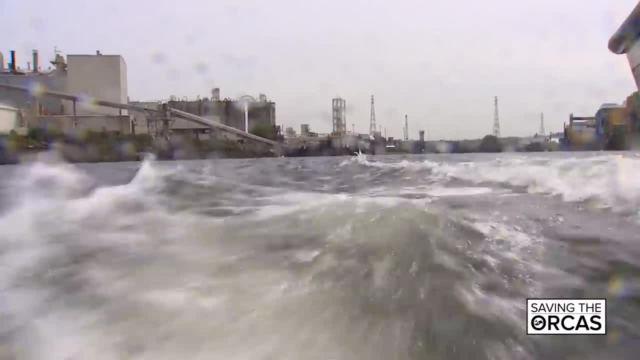 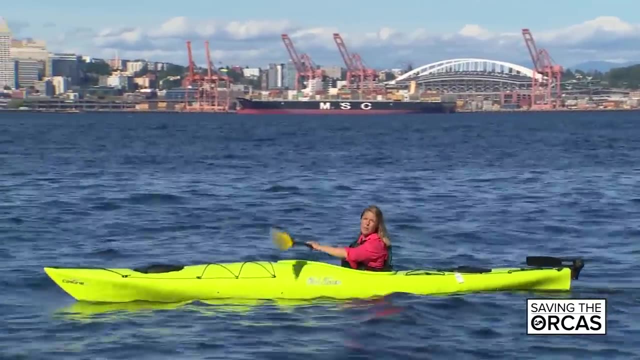 But it shouldn't be falling on us to do this. This is really the central job of the state. The port says that it's done a lot to clean up the waterfront out here. Here's Port Commissioner Fred Felleman. Study of killer whales was my motivation. 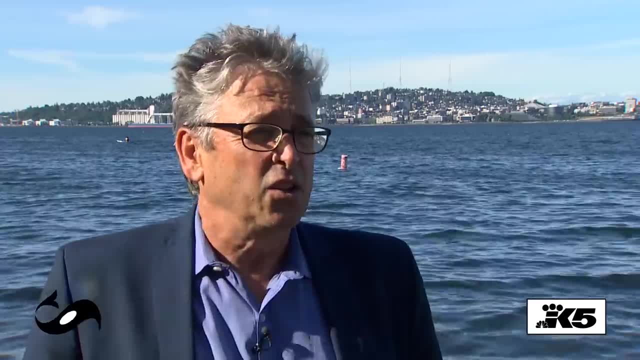 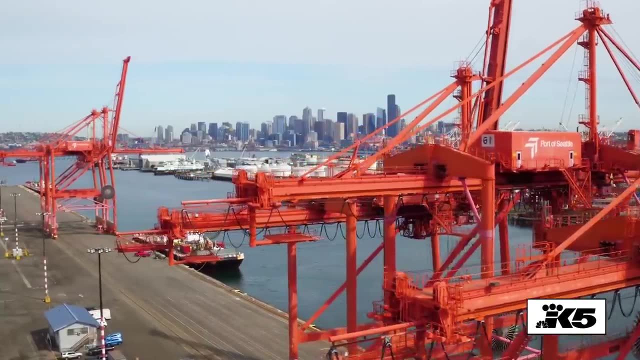 for public service, And I'm proud of what the Port of Seattle has done to restore some of the polluted sites that they inherited. We're not making marine sanctuaries, but we are making life better for both the whales and the people who depend. 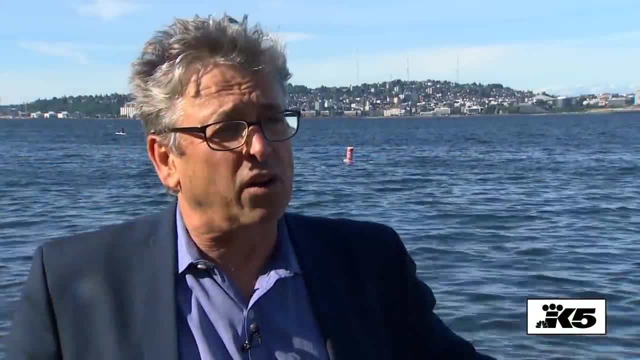 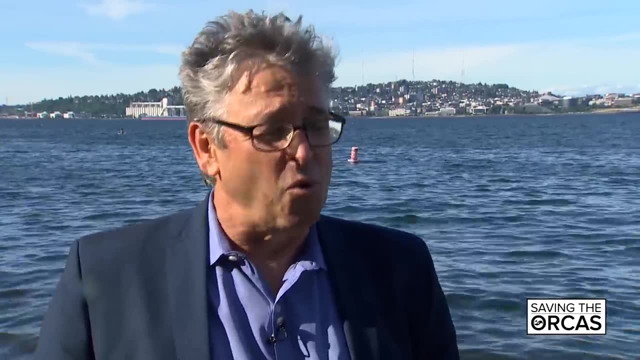 on the marine environment, We have over eight marine parks that provide public access for the public, but also cleaned up the water so it becomes more swimmable, more fishable, but still we have a long way to go. Our wastewater flows into Puget Sound. 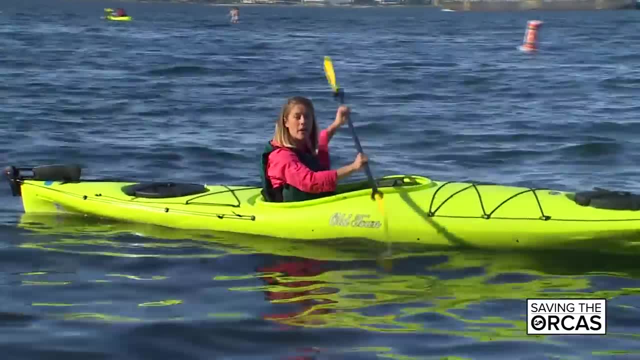 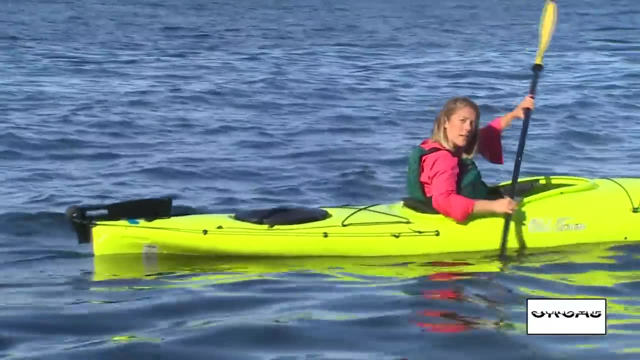 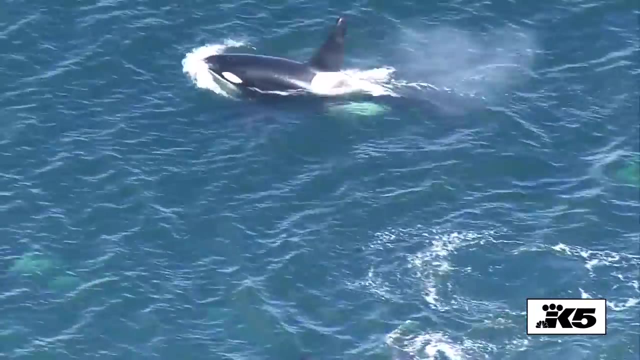 in both treated and untreated forms, And microbes like fungus and bacteria and other parasites make it into the marine environment. So scientists want to know how those microbes are affecting the southern resident orcas. Whenever a southern resident killer whale comes up for a breath, it sprays a mist into the air. 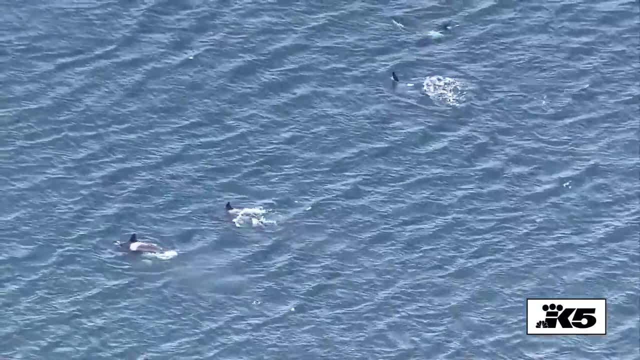 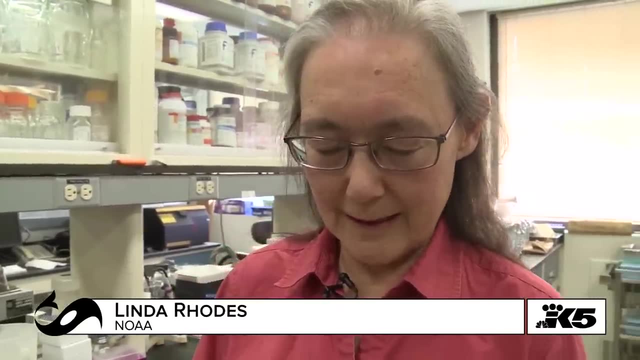 It's a plume of valuable information That contain material from their lungs and their respiratory tract, And we hope to capture that on this nylon mesh, if we're lucky, And then we'll close it back up again And after that we'll extract the droplets. 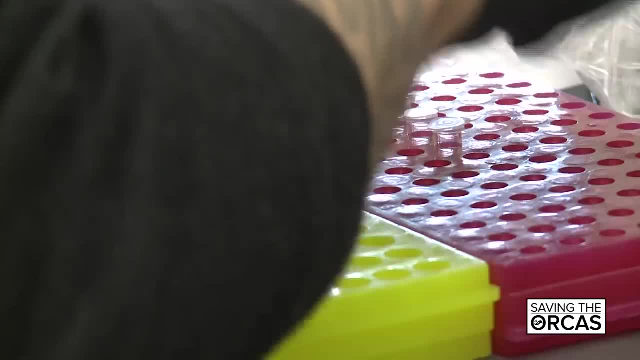 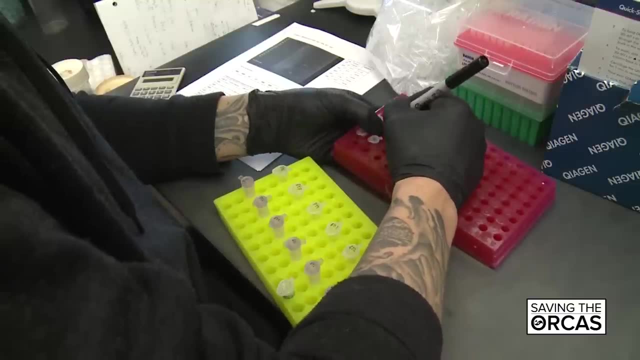 that are stuck to the mesh. Linda Rhodes is a microbiologist with NOAA who is part of a team that's trying to understand how the killer whales are impacted by the tiniest of problems: microscopic organisms that are invisible to the human eye. 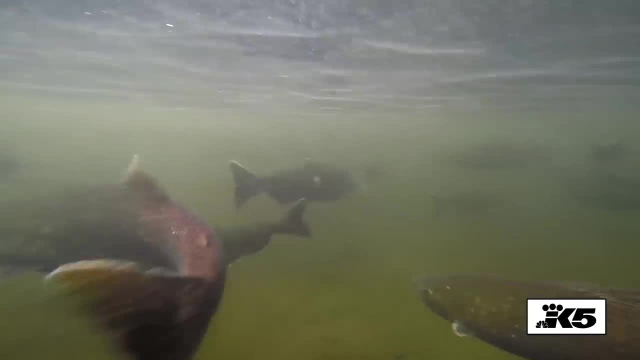 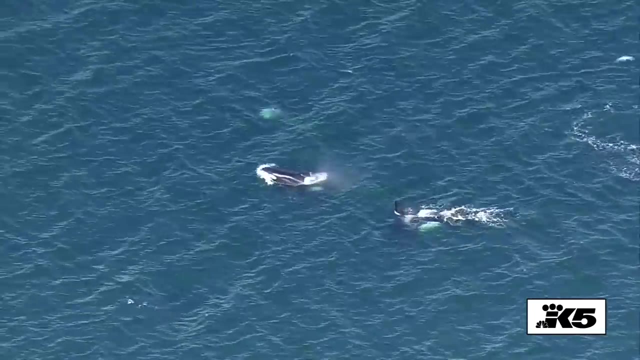 Though lack of food is often a focus of recovery for the orcas who depend on Chinook salmon, which are also dwindling in number, it's possible that disease is making the whales less likely to eat or even more vulnerable to infection. They carry a lot of parasitic worms. in their intestinal tract. And it's not a surprise, because these particular kinds of parasitic worms also infect salmon, and they actually need both the fish and the mammal for that parasitic worm to complete its life cycle. Three years ago, 20 year old male L95 was found dead. 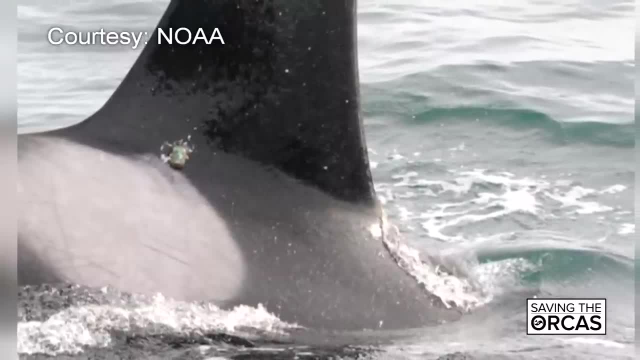 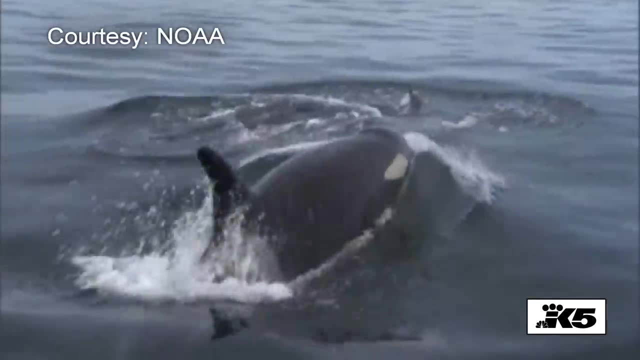 from an infection that started at the site of a satellite tag- And researchers admitted they hadn't followed proper disinfecting protocol- Started at the skin and spread to the lungs, And we figured out what species of fungus that is, And it's a fungus that is very, very active. 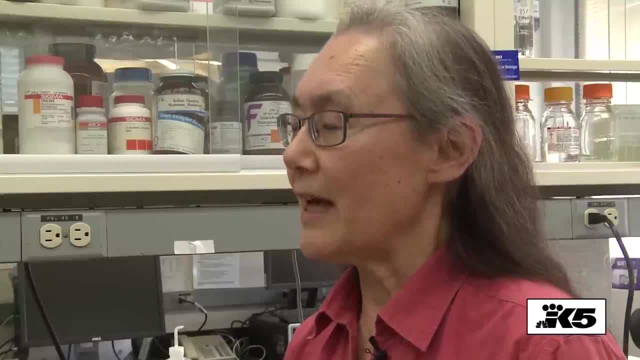 And it's an infection that has been all along the edges of the earth. And it's an infection that has been all along the edges of the earth. And it's an infection that has been all along the edges of the earth, invasive once it gets inside of the animal, and actually it's a fungus that 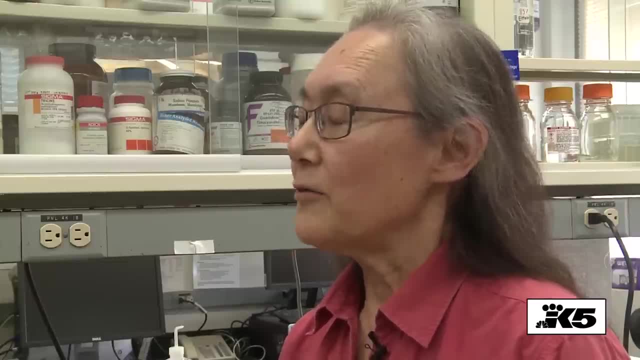 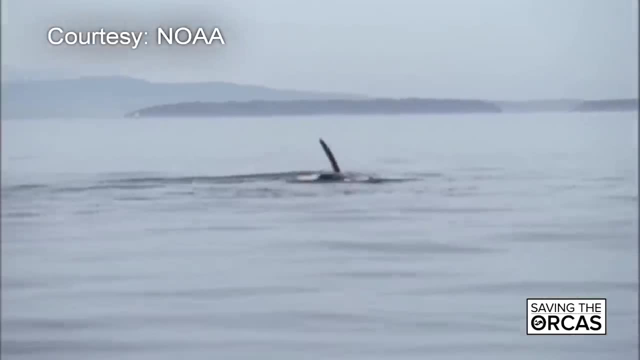 also infects humans, and when it's in humans it's a very bad situation. L95's death showed scientists that infections may be a challenge for recovery of the whales, who often show signs of a mysterious condition called peanut head before they die. Road's team is trying to trace the connection. 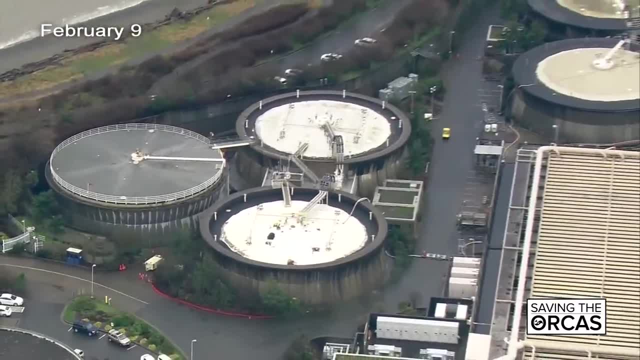 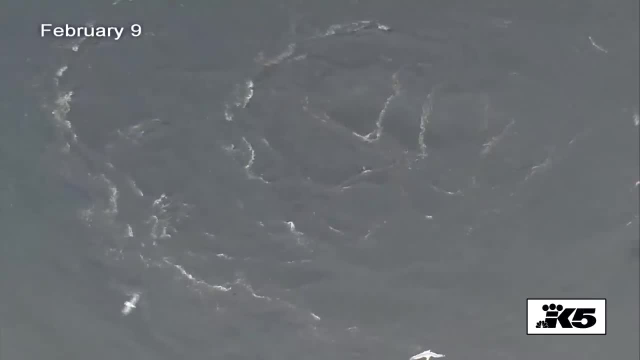 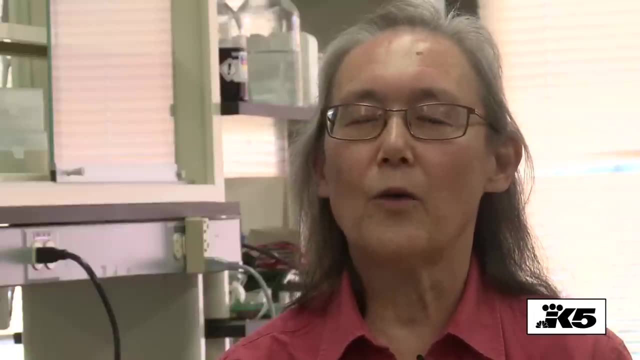 between the health of the whales and our wastewater. This malfunction at King County's Magnolia treatment facility in 2017 released hundreds of millions of gallons of untreated waste. but even on a rainy day, there's a lot of human waste entering Puget Sound and the Salish Sea. I was looking at a study where, on one day in October in 2016, just from the city of Seattle, somewhere on the order of a hundred and fifty million gallons got dumped into Puget Sound through these combined sewer overflows, or CSOs, and the estimate for Vancouver billion is about $1.5 billion. 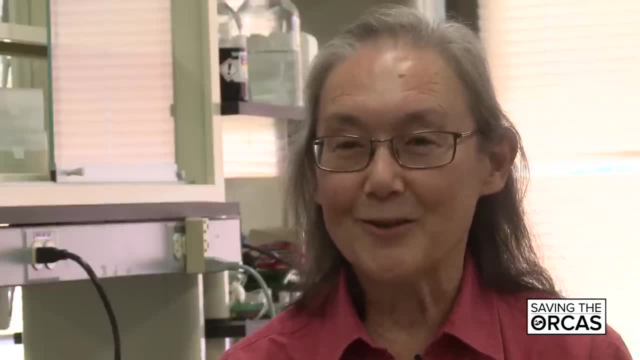 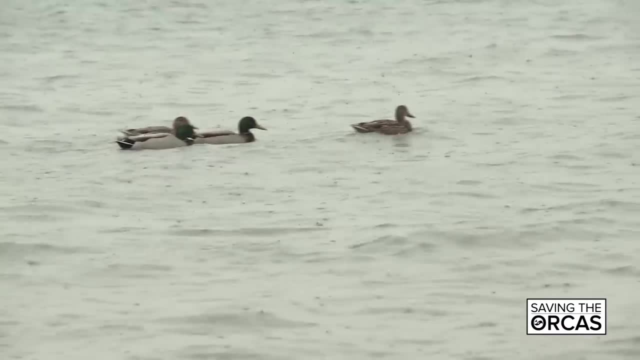 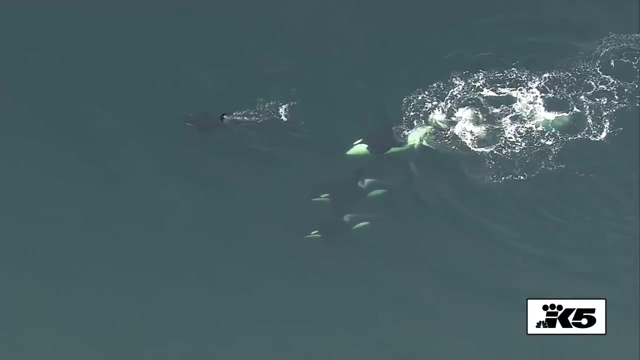 BC is something on the order of 12 billion gallons of untreated waste. In some cases, Road's team has found detectable human fecal material far offshore and deep in the water, indicating our more urban waters are far more contaminated. It's our responsibility to understand what we are. 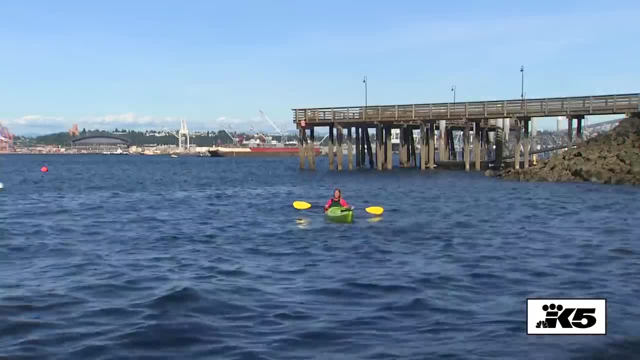 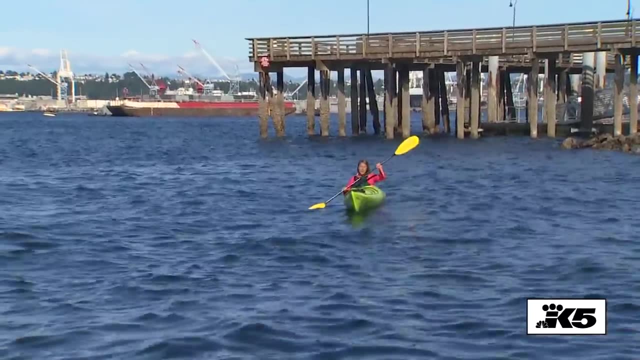 doing because we are the one thing that can change. The southern resident killer. whales are often called some of the most contaminated marine mammals on earth, and it's because they spend a lot of time in urban waterways like this. So every other year, scientists survey fish all around where I'm sitting right. 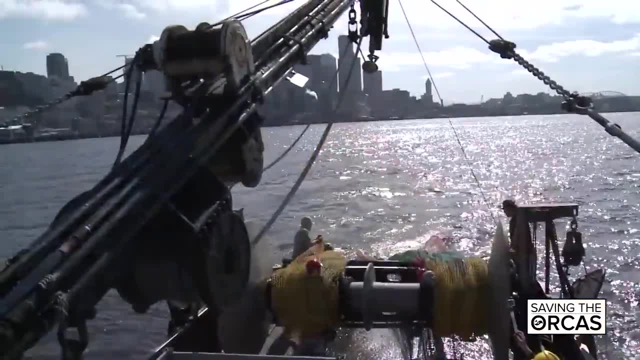 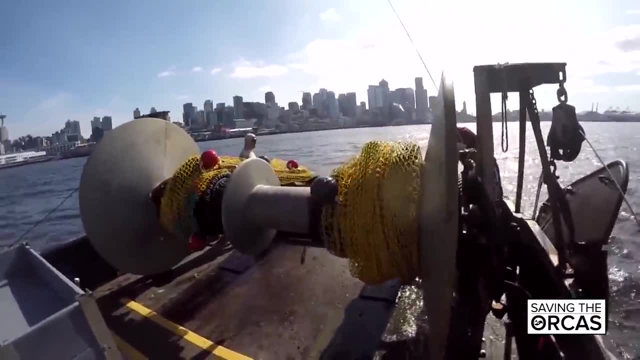 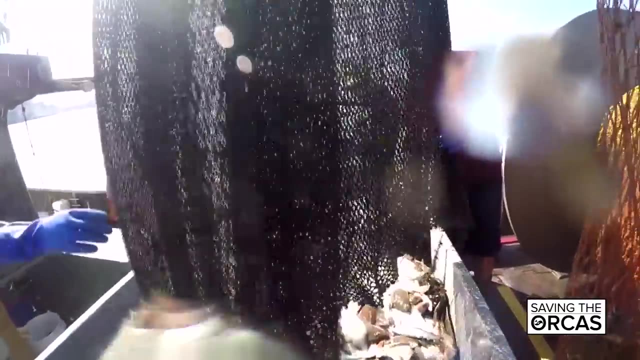 now to test them for toxic contaminants. It's a beautiful day on Elliott Bay, but if this fish survey teaches you anything, it's that what you see on the surface doesn't tell the whole tale. This net is about to pull up fish who live near the floor of Puget Sound, Fish who are 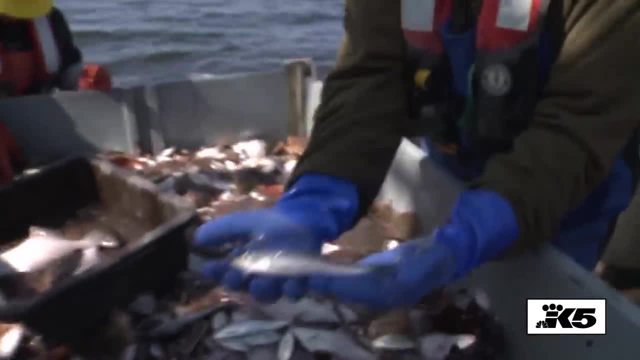 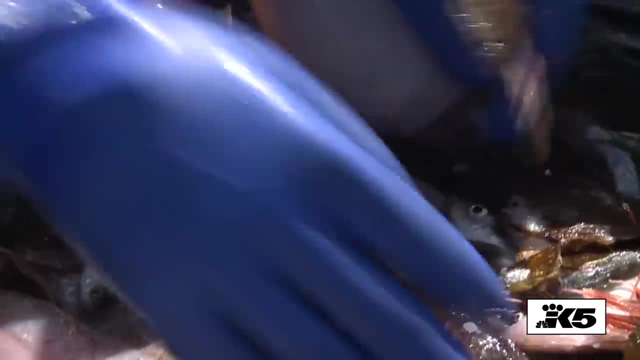 exposed to contaminants in the sediment. These are spawning in Elliott Bay. Jim West and a team with the Washington Department of Fish and Wildlife have been doing these surveys for nearly 30 years. We got about four or five species of soul in here and we're trying to pick. 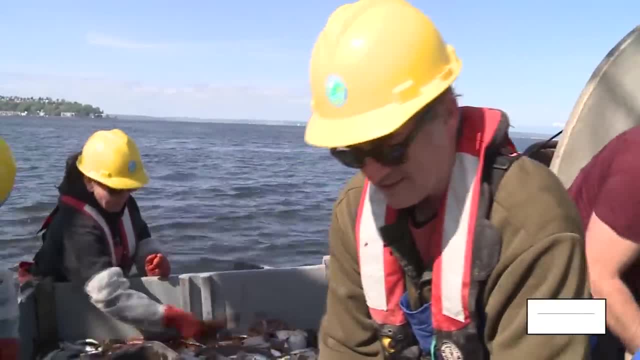 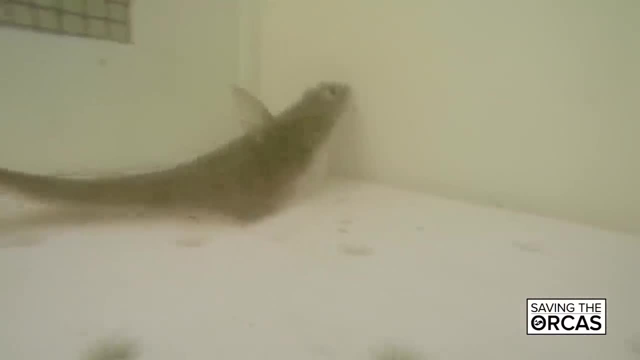 out the ones that were called English soul. Here's a skate. Once the fish are sorted and the rest returned to the water, the English soul are put in a holding tank. It represents what's happening on the seafloor in the sediments. A lot of contaminants end up in the sediments, and so we want a. 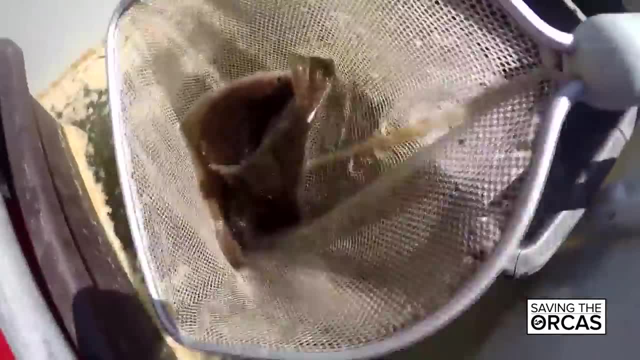 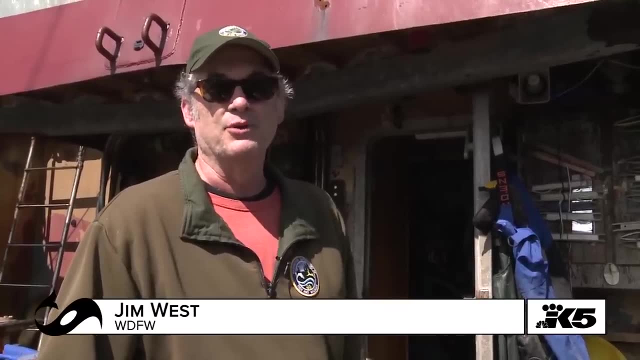 lot of fish that are sitting there and feeding in the sediments. But in the sediments the contaminant loads in Puget Sound are pretty much in the urban areas, So we can find English soul out in the middle of Puget Sound that are really 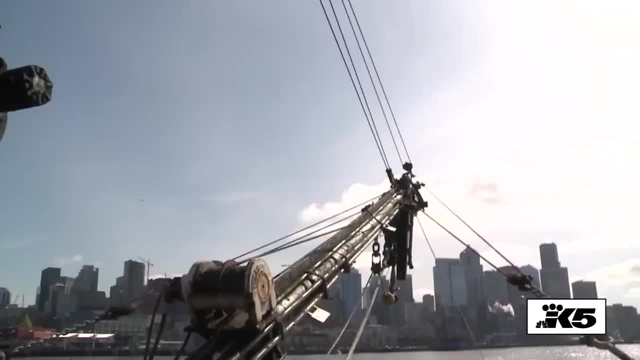 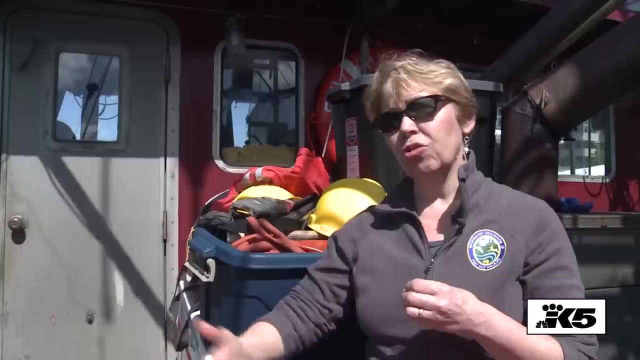 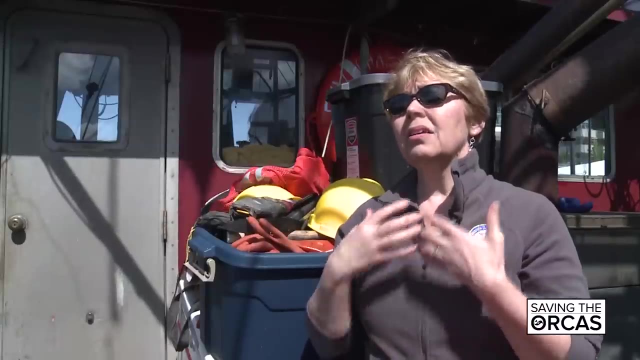 clean, but as soon as you move into a place like Elliott Bay here they're highly contaminated, West says. in seven of ten survey sites the contaminants are either not declining or getting worse Over the course of our lives. the more we eat, the more it accumulates, and whatever if we eat a fish, we are then in. 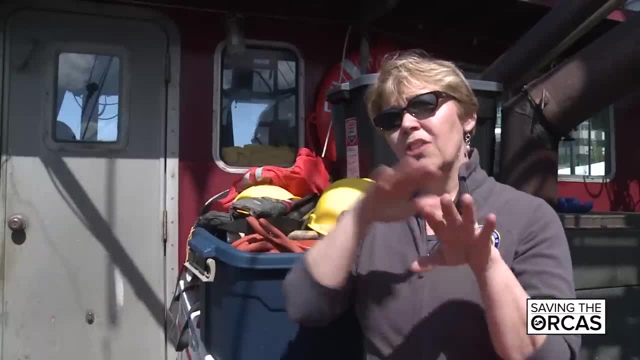 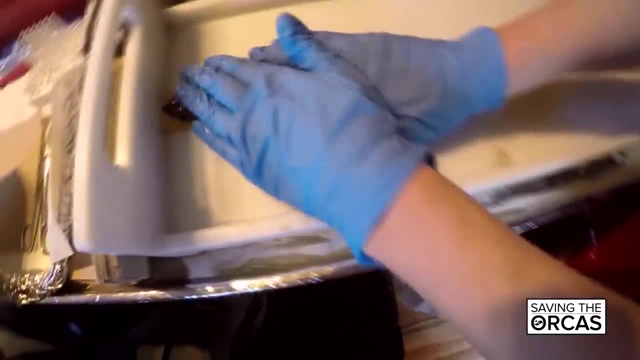 consuming and accumulating what the fish is eating, and so as you move up the food chain, you get higher and higher concentrations of these bioaccumulative contaminants. Senior research scientist Sandy O'Neill calls the fish an indicator species that gives early warning signs of the health of Puget. 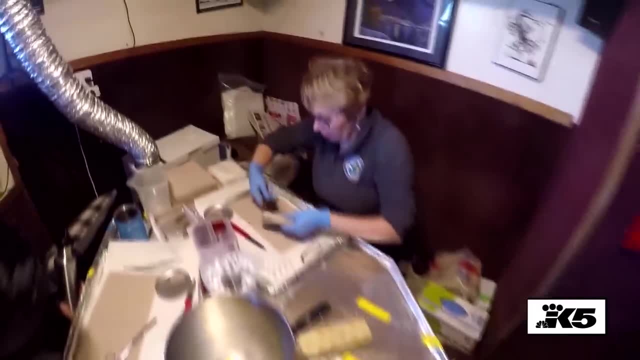 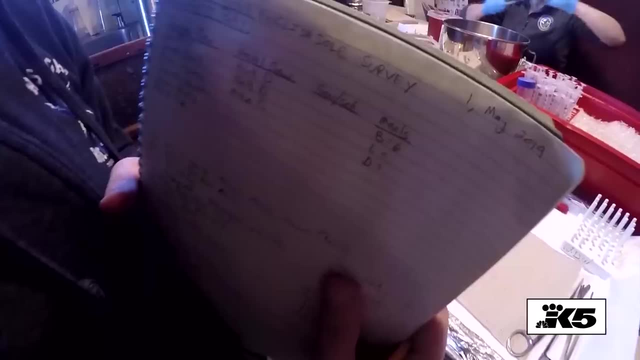 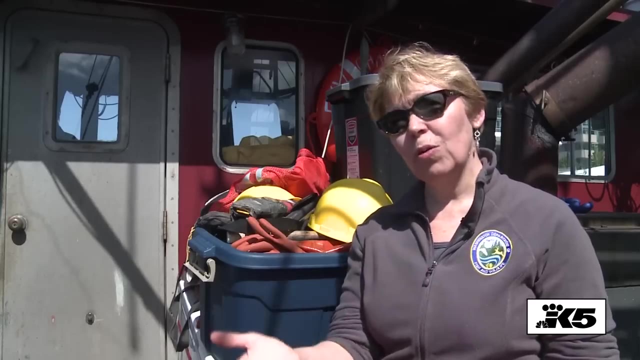 Sound. They're tested for chemicals used decades ago, like PCBs, as well as what are called contaminants of emerging concern, like pharmaceuticals. When you get a prescription, you go to the pharmacist. you know the first thing the pharmacist says is say: looks at your list of medications and tells you: is it? 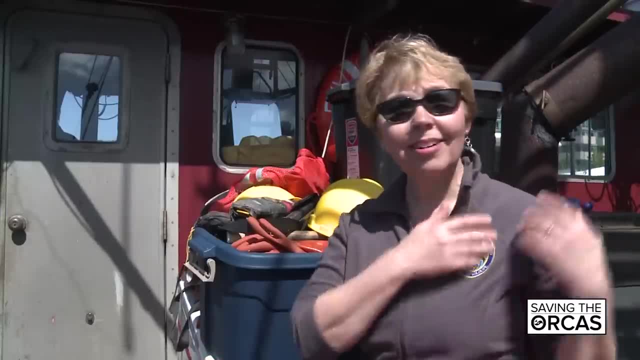 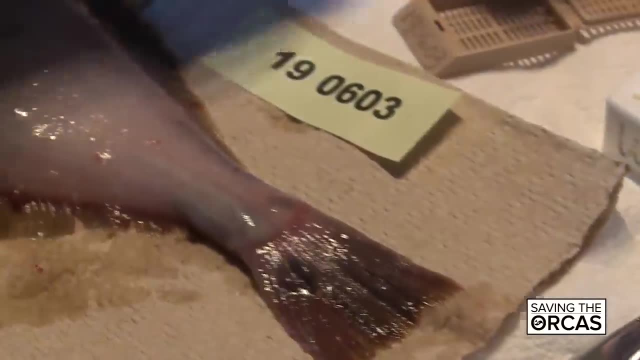 okay to take this medication. with that medication, The fish don't have that option. they're just they're getting exposed to a whole slew of them all at once. The scientists have found compounds that model estrogen are likely causing male fish to produce female egg yolk protein, and that includes salmon a. 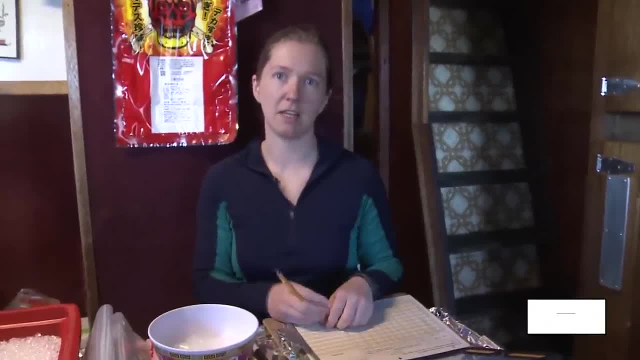 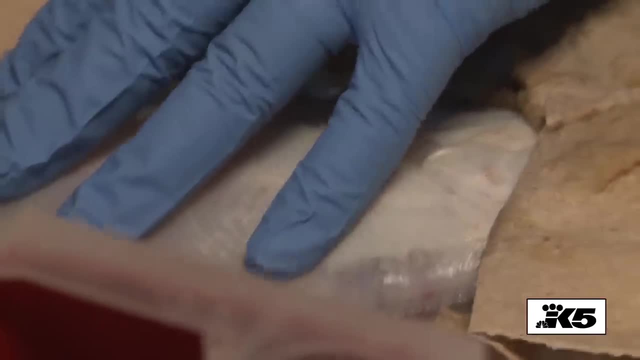 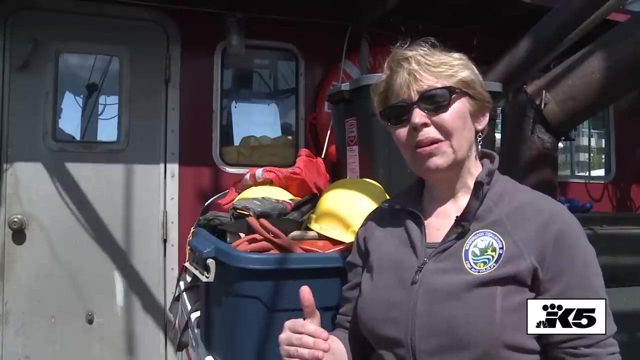 favorite food for the southern resident orcas. It throws off their hormone balance and it could affect their ability to reproduce. The long-term monitoring data that we produce can be used for can be used to document effectiveness of any management actions that are implemented, So we're going to see declines in contaminant levels in. 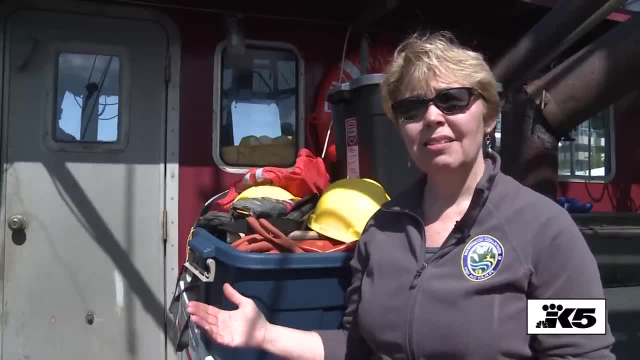 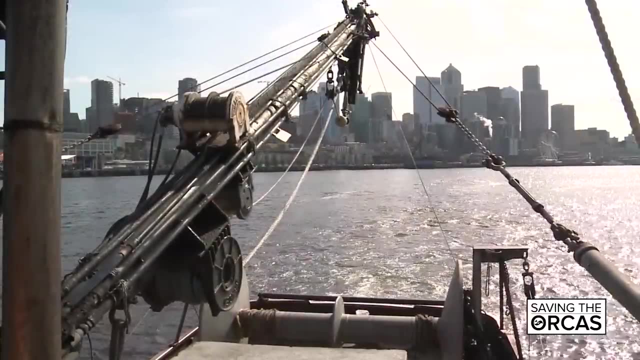 herring and juvenile salmonids before we're going to see declines in contaminants and killer whales. So they will be our early warning indicator species that things are getting better or worse. Cities all around western Washington are starting to take inventory of their effects on the 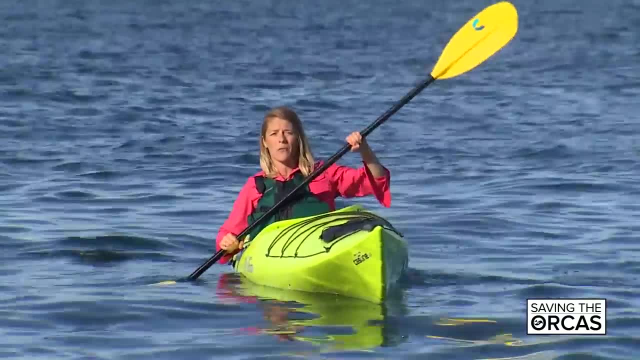 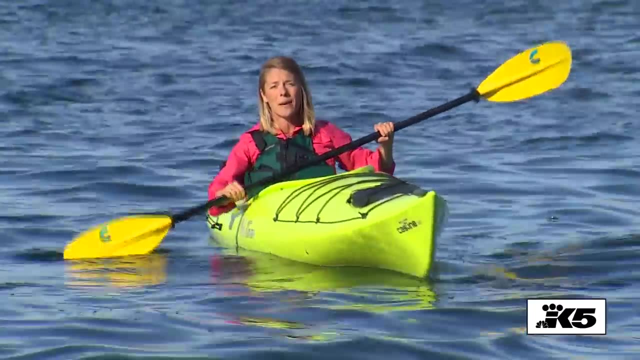 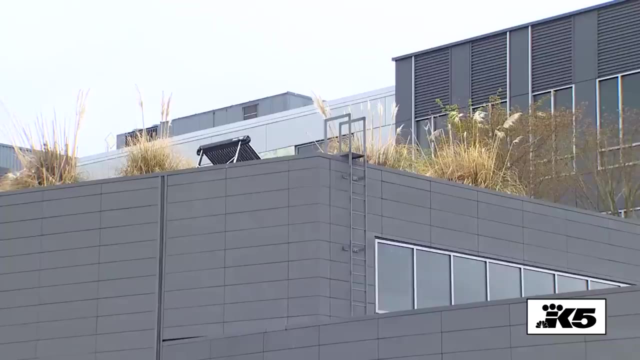 southern resident orcas. In fact, Shoreline just became the first city in Washington state to become salmon safe certified, and they're second in the country, only to Portland. But it did not come without its share of mistakes and lessons learned. Shoreline's new city hall building was meant to be a beacon. 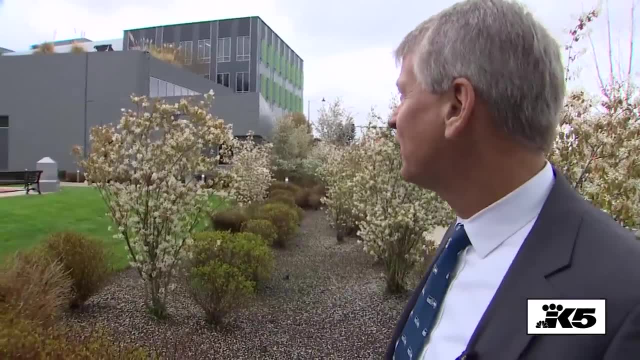 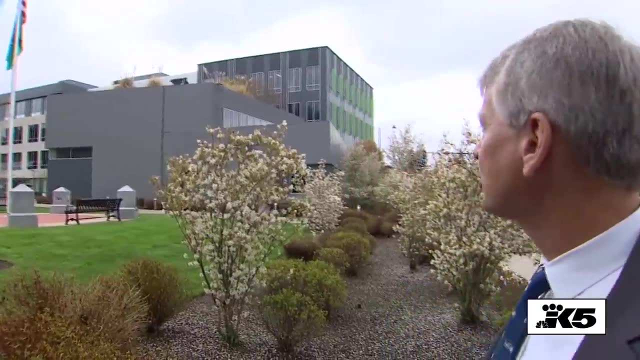 of environmental advocacy. We built in a number of environmental features. The green roof on top of city council chambers have plants that filter the rain and slow it down before it goes into our stormwater system. There's there's a lot of things that we're going to have to do to make sure that the 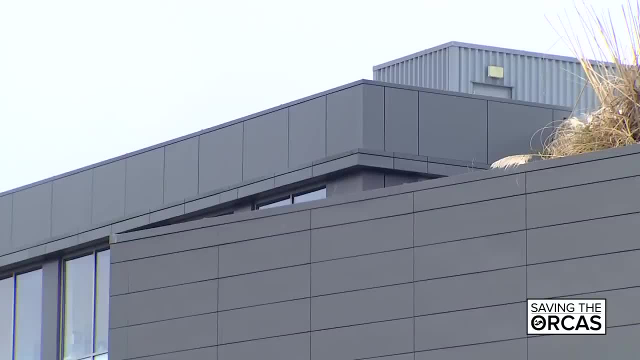 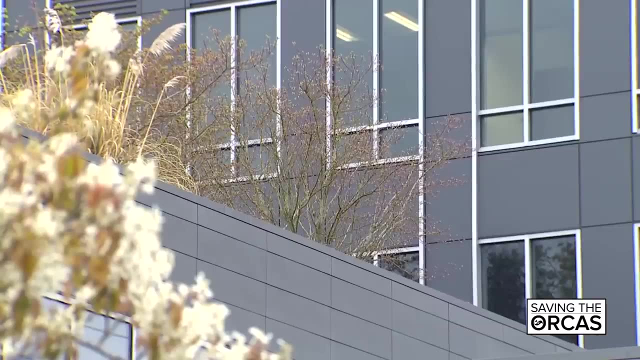 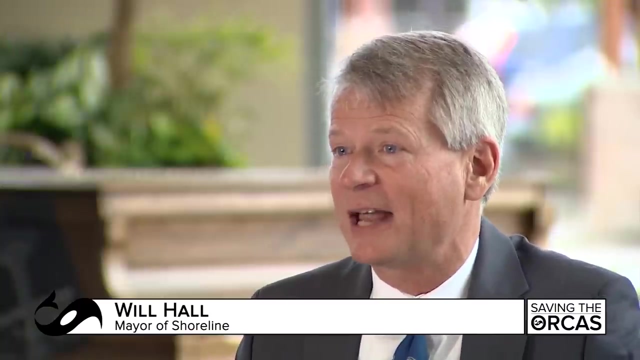 there's hot water heated by the sun. on top of the council chambers and on top of the parking garage there's a huge solar array to generate electricity. But after it was finished, city officials learned the building was actually bad for salmon. We built the building to meet up to a very high level of industry standards. 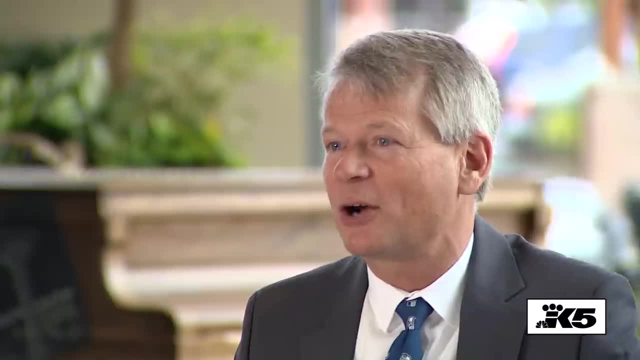 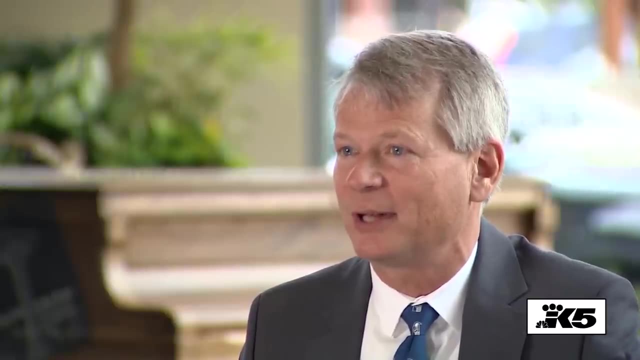 but that standard didn't take into account stormwater, and it was when we started looking more at water quality and salmon protections that we realized that the building itself was a source of stormwater pollution that needed to be treated. Shoreline Mayor Will Hall showed us the problem: The building's outside walls are 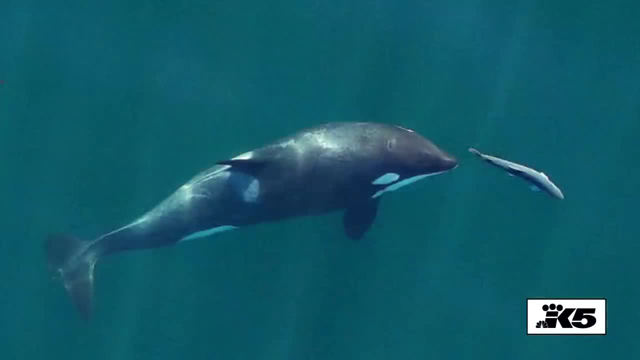 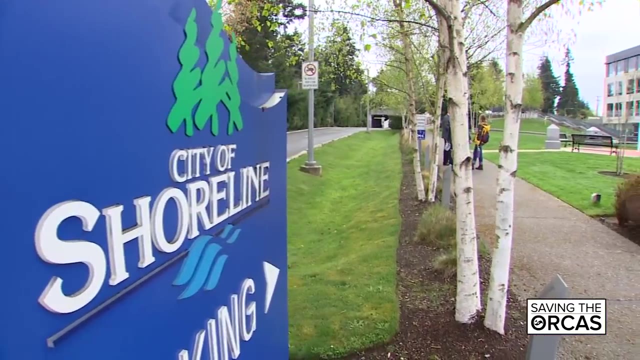 coated in zinc, And zinc is toxic for fish like the Chinook salmon that make up the main prey for endangered Southern Resident killer whales. That's when Shoreline decided to get even stricter with its building codes. Our community wants to see salmon and orca. 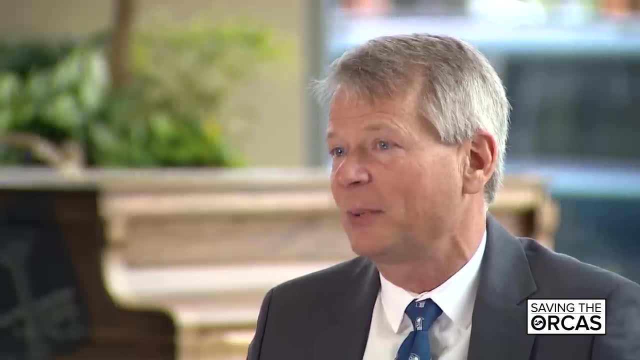 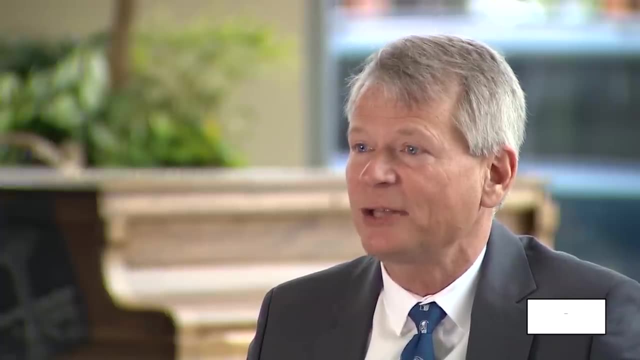 whales in the future, and so they're demanding that our local governments do its part. So we're looking for ways to become better for the environment and the salmon. safe certification is the way we're going to do our job, the program that's helping us learn to do better. Now, the second city in the 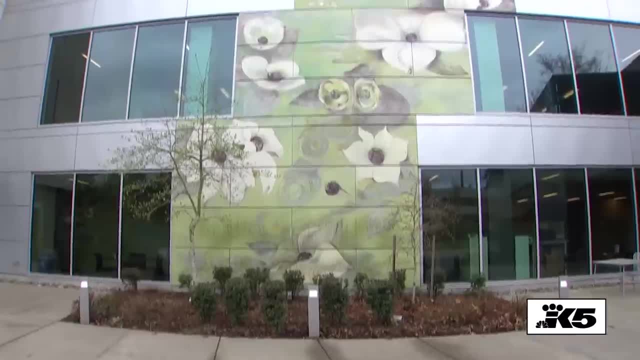 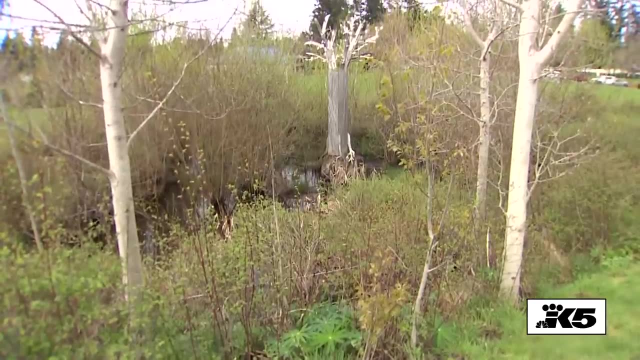 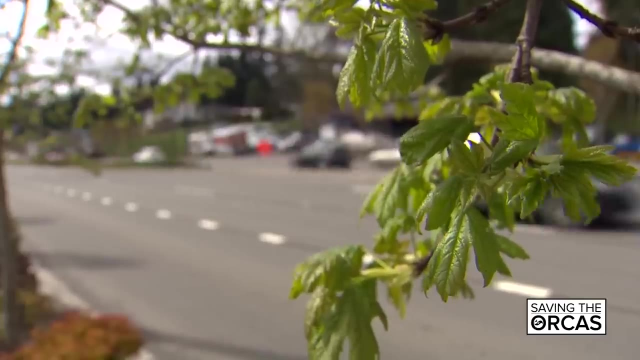 entire country. to be certified salmon safe, new infrastructure will have to follow stricter building codes. The city is also focusing on green infrastructure, like this park, designed to trap stormwater and filter contaminants, just like these rain gardens on Aurora Avenue. We've watched this region grow for the 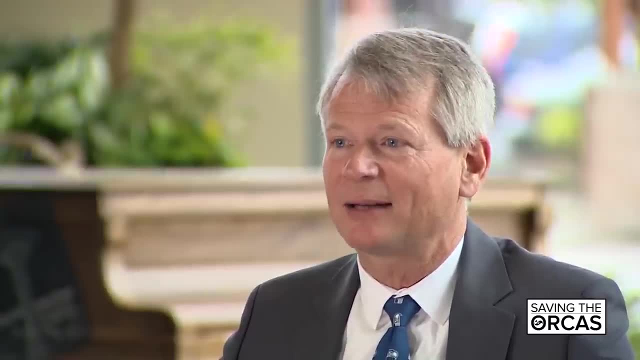 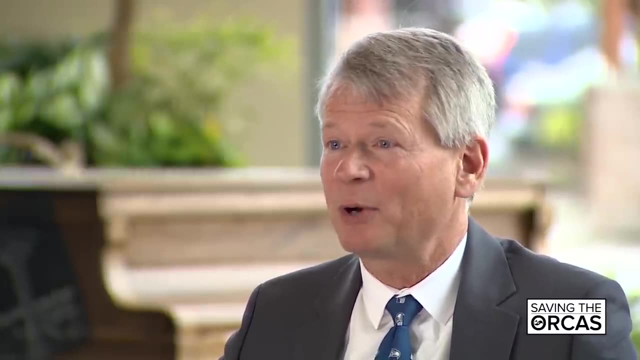 past five decades. All of that growth is having an impact. Every time a car drives down the road, it leaves little bits of its tires, little bits of its brake pads, little bits of its exhaust, and then, when it rains, that rain carries all of that. 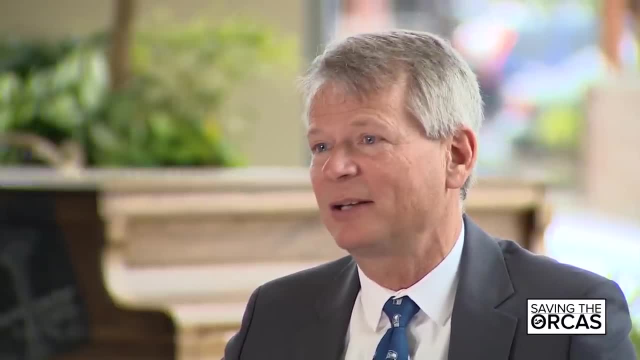 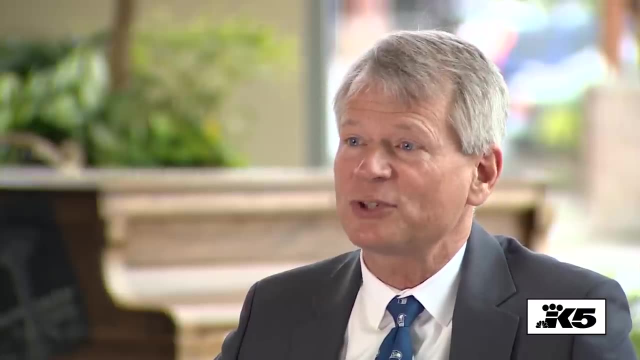 pollution into Puget Sound and that's part of what's killing our salmon and killing the ecosystem. So people in this community are saying enough is enough. They want us to clean up the environment and that's what's driving our City Council to take these steps. Hall says they're committed to do whatever they. 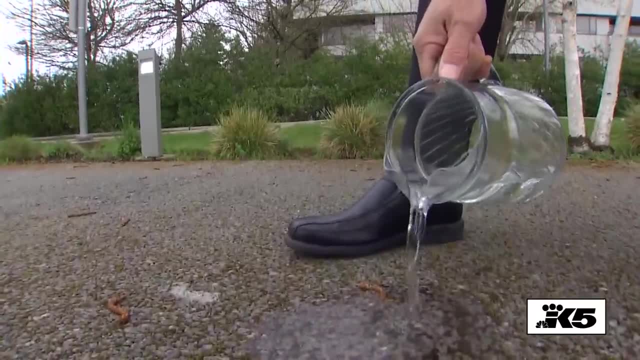 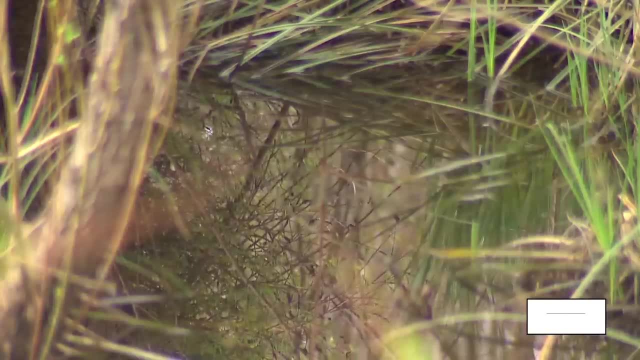 can here in Shoreline, whether it's a short sidewalk built with material that traps stormwater, or a big park that reminds everyone of the importance of clean water. My hope is that here in the city of Shoreline, we'll learn to make all of our 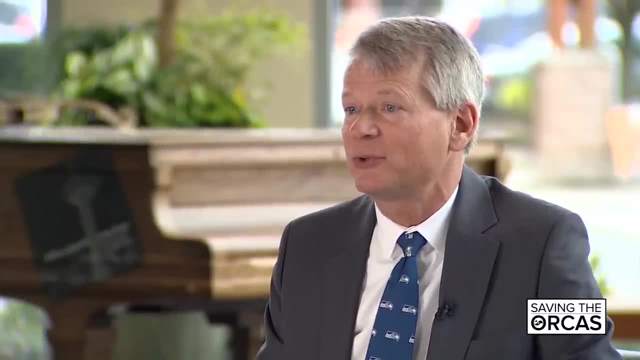 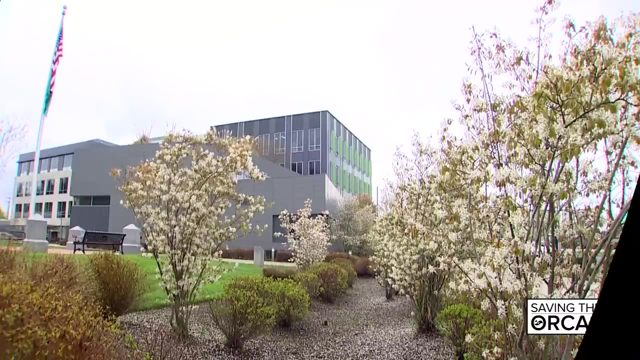 practices safe for the salmon and that other cities around the region will follow suit and that our children and grandchildren will be able to go salmon fishing and watch the orca whales just like we did when we were kids. Lack of food is the number one threat to the survival of the southern resident. 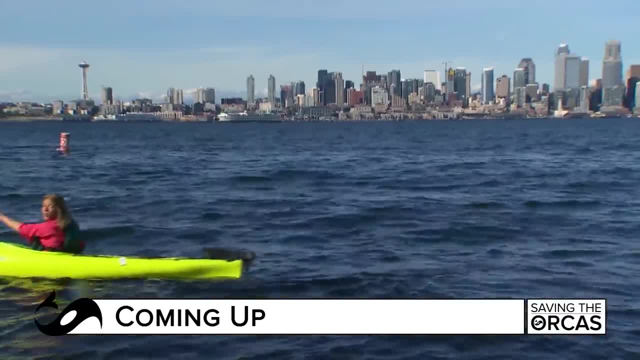 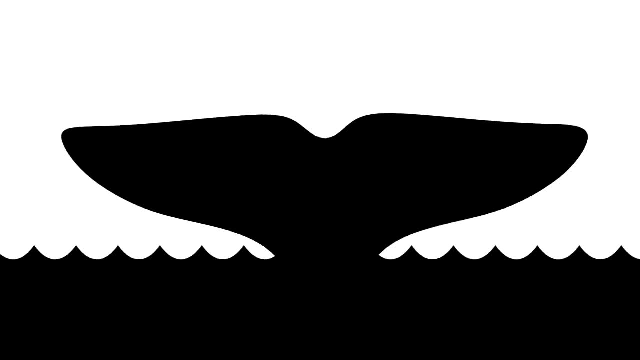 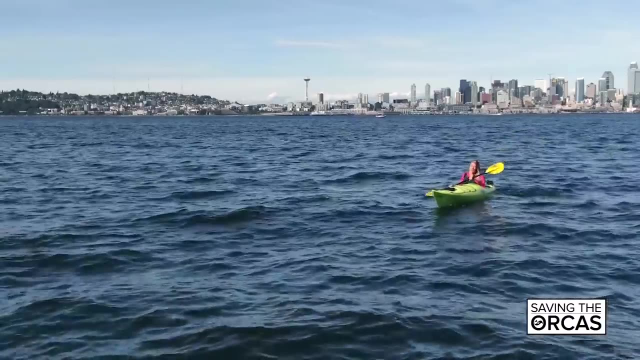 killer whales Coming up. we'll tell you why salmon are disappearing and what we can all do to save them and the orcas who depend on them. So far this hour, we've learned about how noise and pollution are hurting the southern resident killer whales, but the main challenge to their survival is a 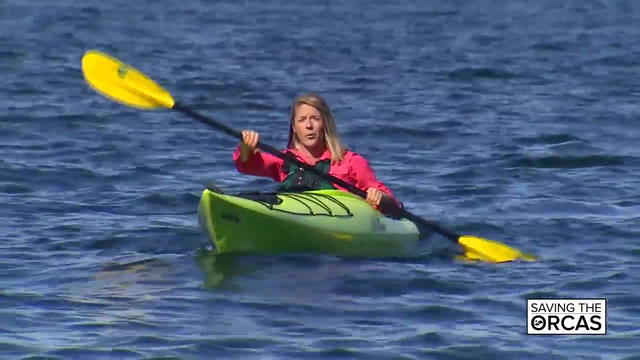 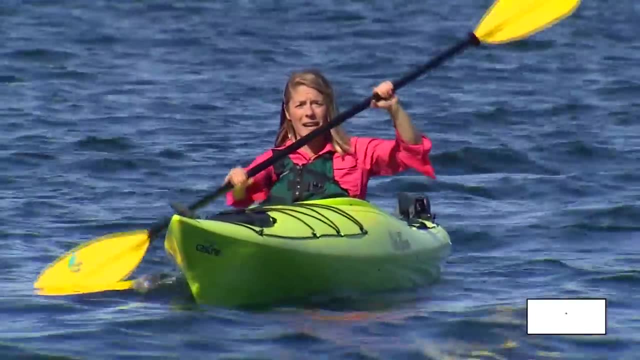 lack of food. You see, these orcas don't eat other marine mammals or sharks, like other orcas do. They only eat fish, and their favorite food, Chinook salmon, are also declining. So the story of saving the orcas is really a story that's been 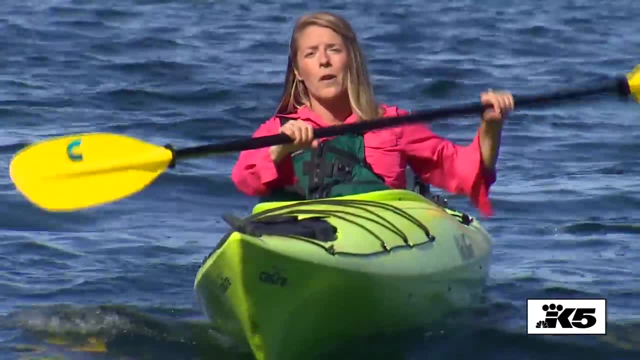 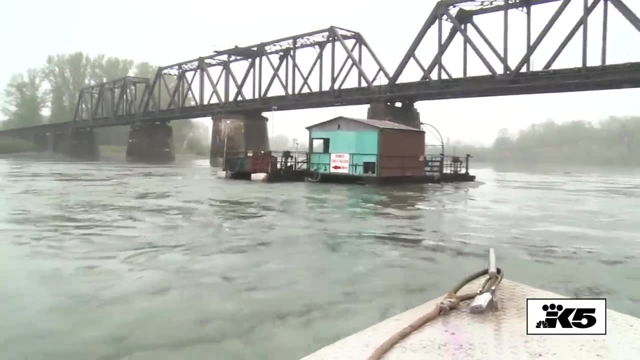 passed down through history. First we're going to go to the Skagit River, one of the most important rivers for salmon in the Puget Sound region. In the middle of the Skagit River, somewhere near Mount Vernon, there's a hut-looking 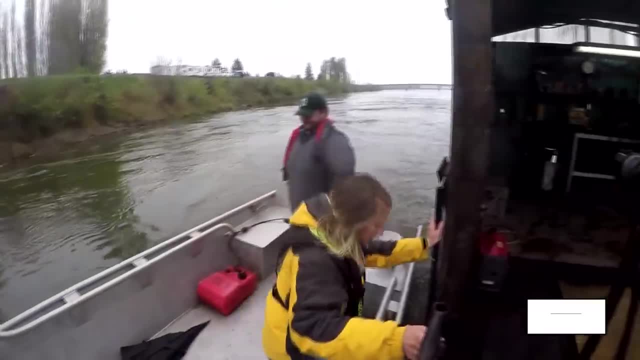 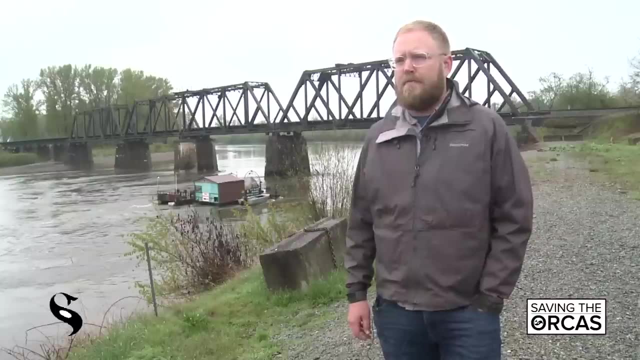 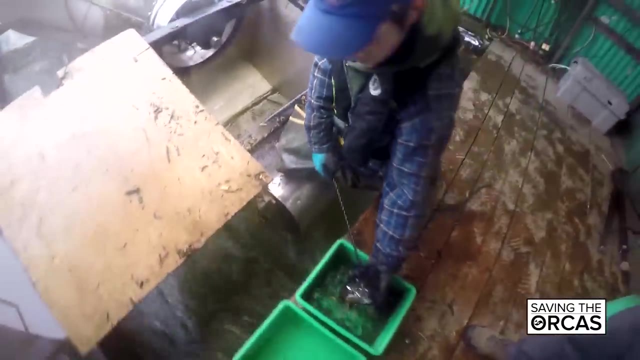 structure floating on the brown water. It's a fish trap where each morning state wildlife technicians check to see what's been caught. We operate it from January through mid-July to count juvenile salmon as they're migrating towards Puget Sound. Ben Kinsol is a biologist with the Washington Department of Fish and Wildlife and his team 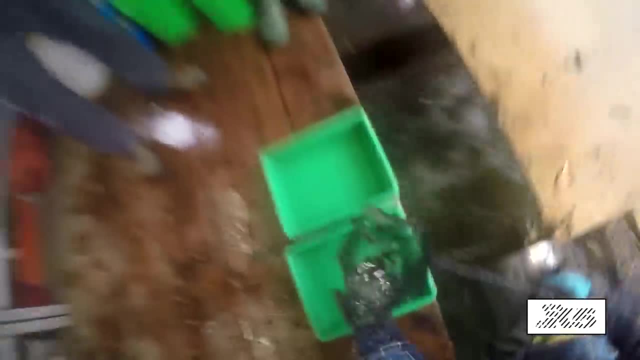 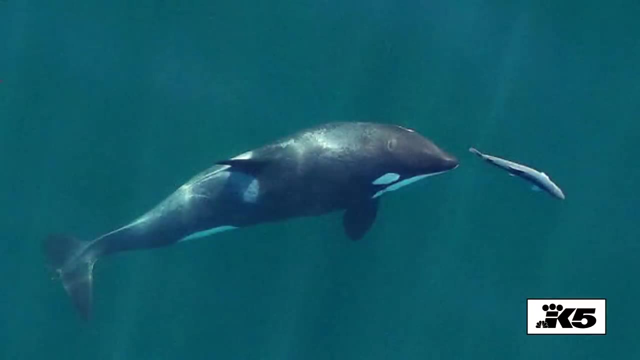 is mostly counting chum salmon. right now some 3-4 thousand each night. Southern resident killer whales do eat chum, but scientists believe their diet depends on Chinook salmon And, like killer whales, Chinook salmon runs are dwindling. This fish trap is helping scientists. 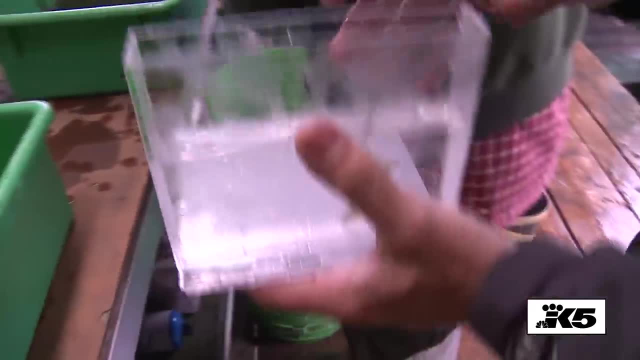 figure out how to stop that. It tells us how many fish are coming downstream to the Puget Sound. It's a tool we use to set fisheries, manage fisheries, to inform the community Fishing for Chum. you can find it on the Kinsol website. 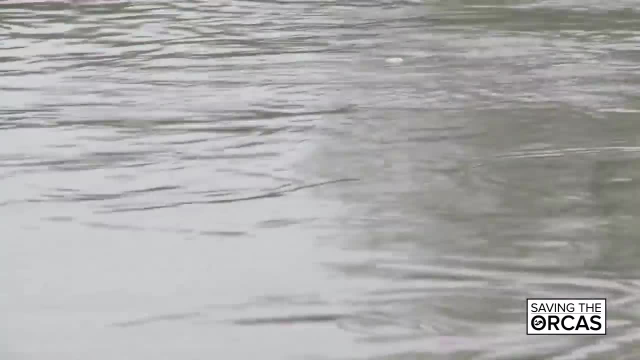 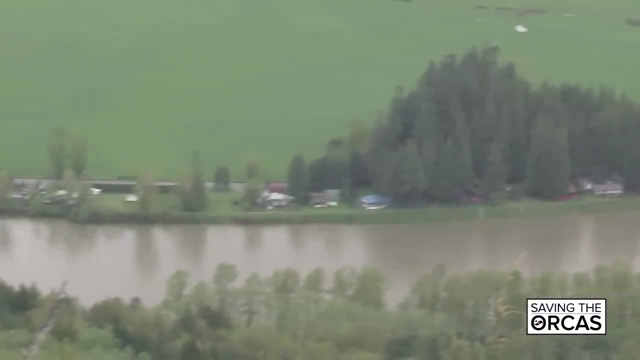 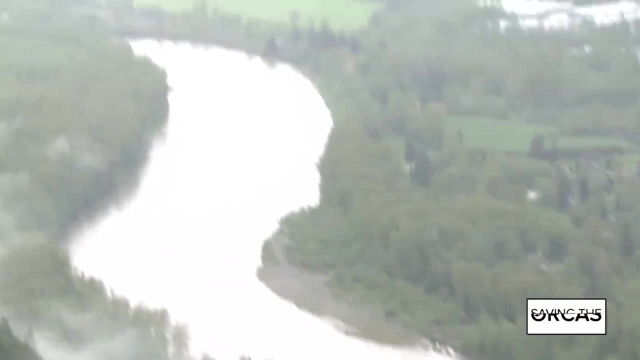 to inform habitat restoration in the lower river. Habitat restoration, the two words you'll hear more than most when it comes to Chinook salmon recovery, especially here on the Skagit River, where dikes and levees have cut off side streams that are important for young salmon trying to grow bigger and stronger for their journey to the ocean. 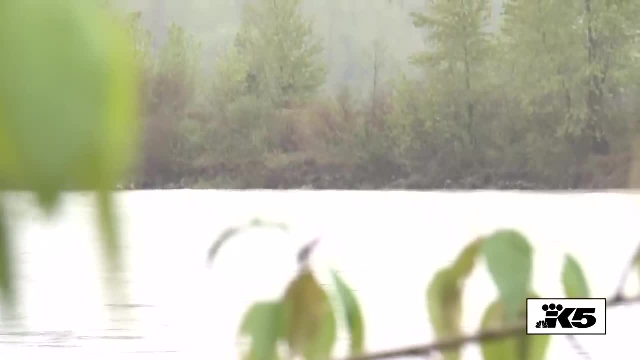 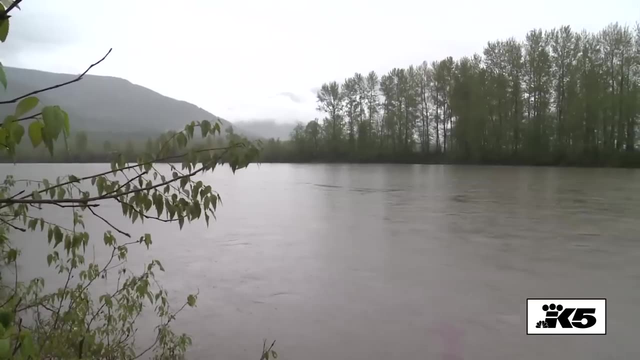 These are places where the river used to flow many years ago and are now cut off. As a result, those places are now inaccessible to juvenile salmon moving down the river. Corey Green is a federal scientist with NOAA's National Marine Fishery Science Center. 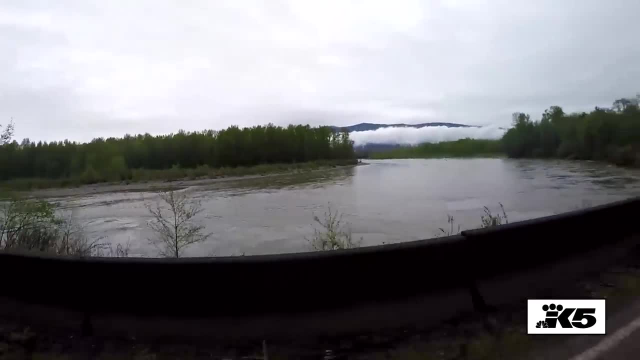 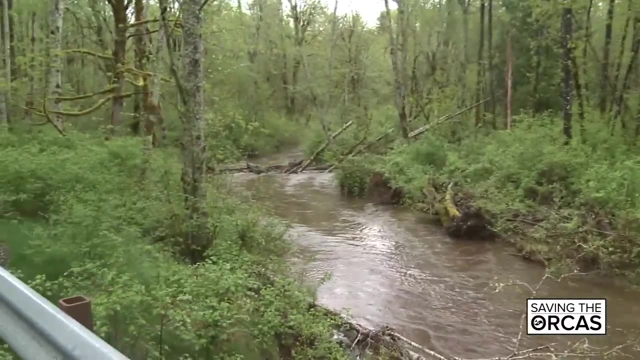 Instead of a well-manicured river with a road right next to it. he showed me what young salmon need to survive. As you look downstream, you can see a big pile of wood, and those areas provide safe places for salmon to rear. 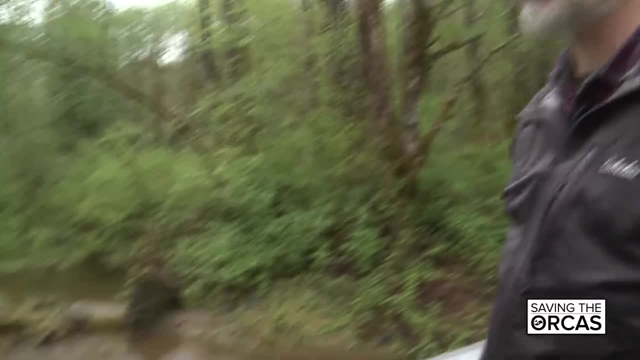 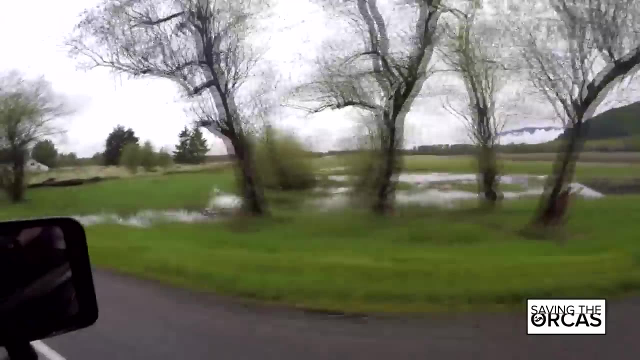 And then these little spots right here, this little pond. that's another place where salmon can duck in This land is what Green and other scientists call a freshwater floodplain. It's important for salmon, But it also makes for great agricultural land and scenic riverfront properties. 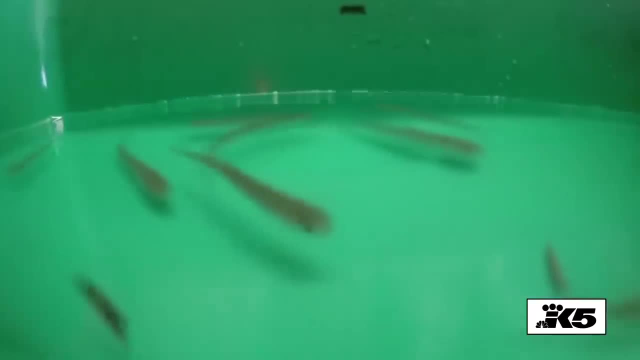 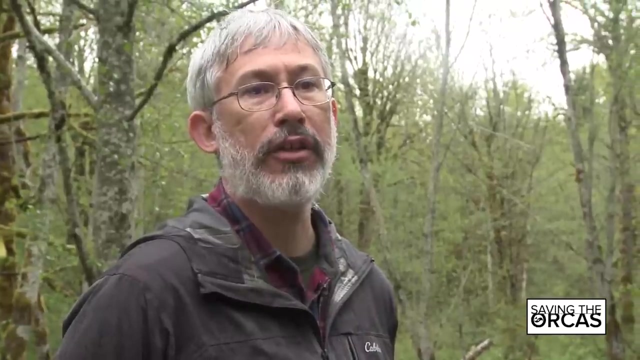 The Skagit has lost more than 50 percent of its floodplains and Chinook salmon runs are just 10 percent of what they once were. A pretty large wild population, the largest in Puget Sound. Nevertheless, you've got less habitat for rearing salmon to use as they're bulking up. 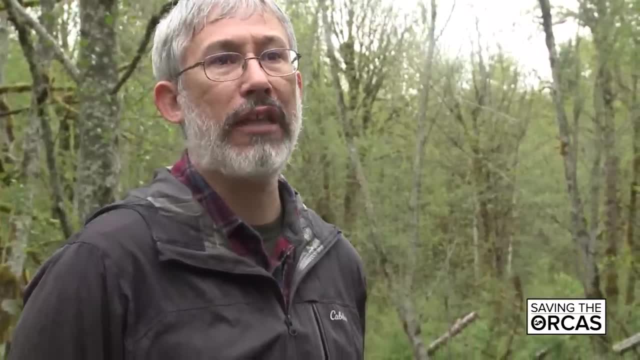 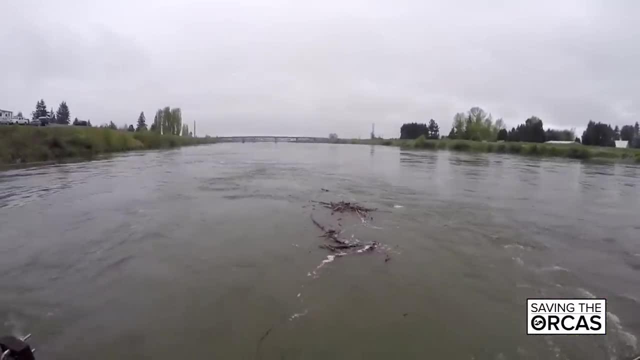 And, as a consequence, they compete with each other, And so that lost habitat means loss, And that's why we're trying to get the best production of adults down the line. It's on rivers like the Skagit where scientists and others are trying to figure out a balance. 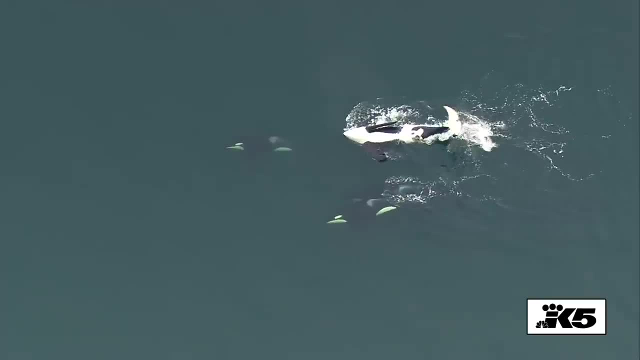 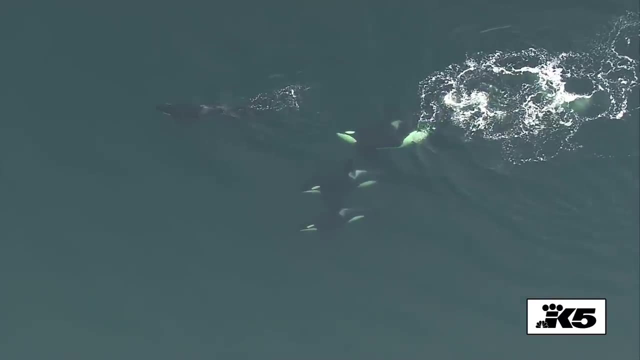 so we can produce food for hungry humans and food for hungry whales. It's going to take a long time to feel the effects of recovery, And so there's some short-term solutions people can take, and there's going to be longer-term ones. 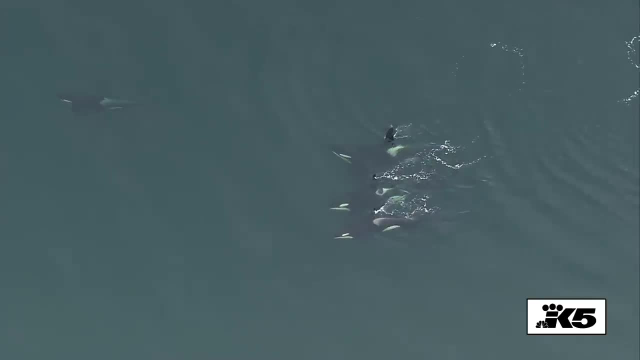 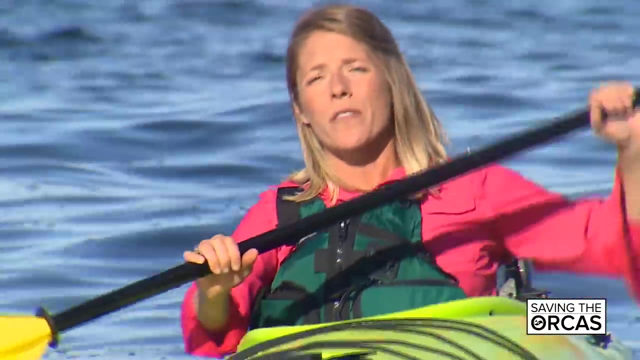 And if we want to have a population of salmon to feed those orcas, we need to think about the long-term as well as the short-term. And those long-term solutions really are about habitat. You just saw the importance of the habitat upriver. 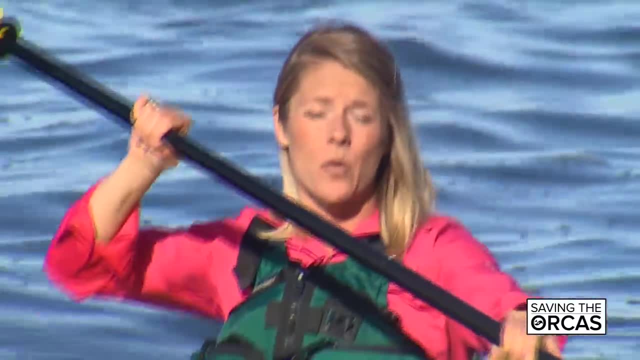 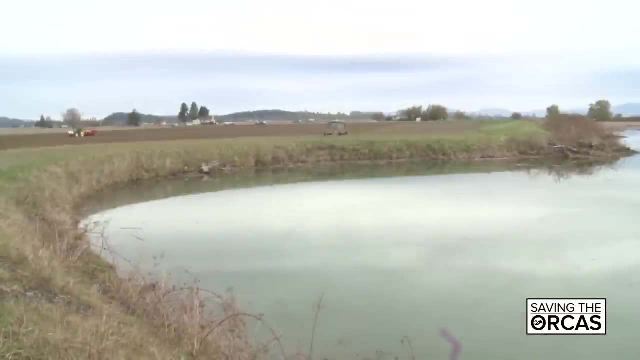 but the part of the Skagit river that empties into the Sound called the estuary, is also vital habitat for salmon. It's where salmon take even more time to grow up big enough to venture out to the ocean. The channels give safe habitat filled with food for growing Chinook. 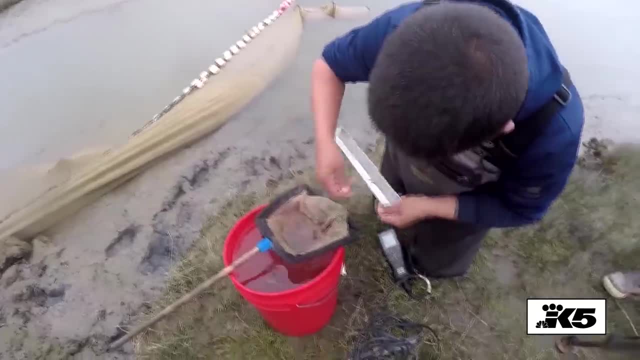 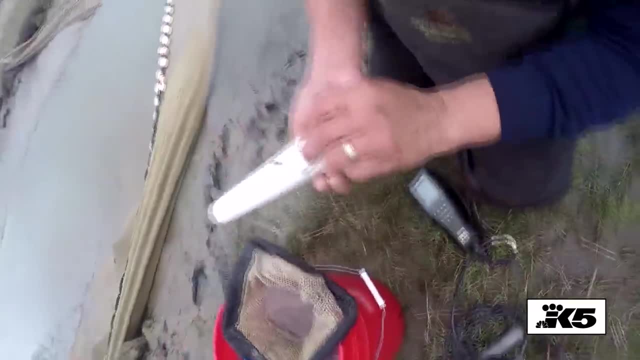 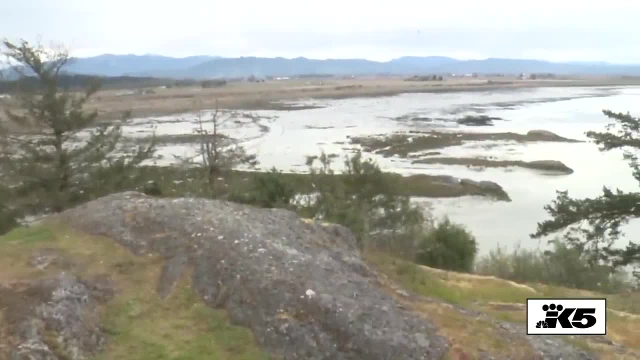 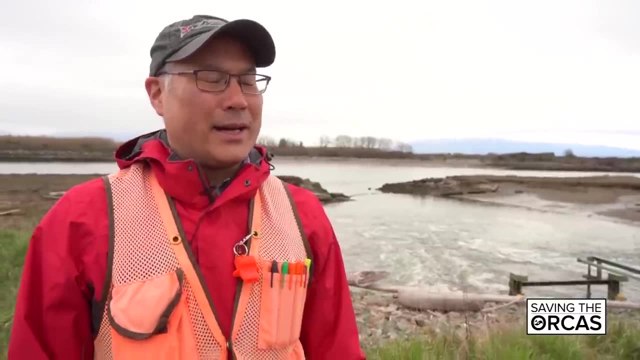 That will mean restoring hundreds of acres and protecting existing habitat like this. Right now. I'm the seventh generation from my ancestors at the treaty signing time And I don't think they could ever imagine what things could have changed to looking at the landscapes they are now. 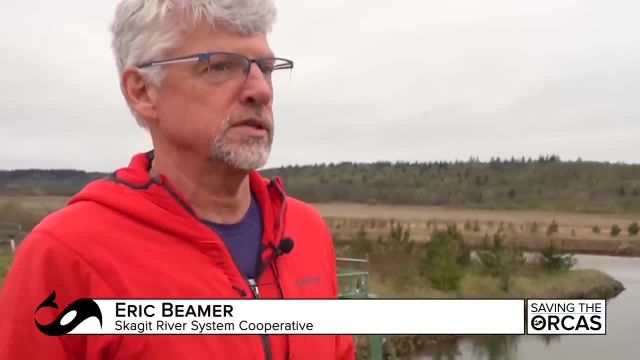 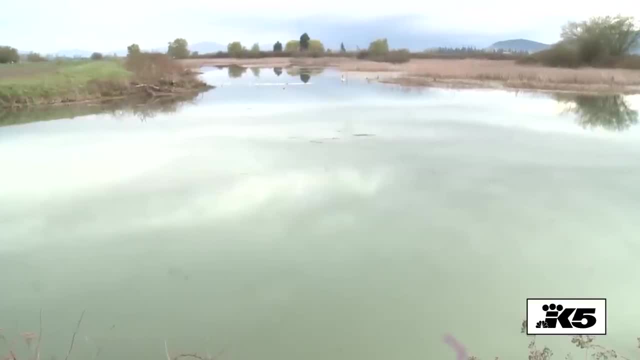 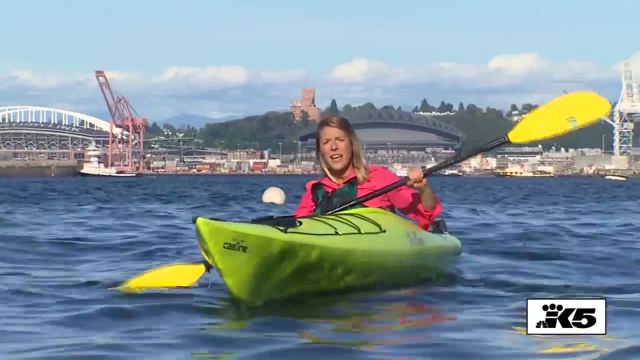 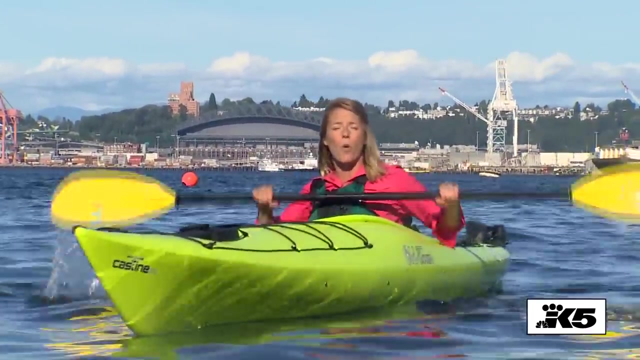 To restore enough habitat to achieve salmon recovery goals. There is so much habitat to restore for salmon that some estimate it could take 90 to 100 years. So some farmers are stepping up and taking the lead, and one of them is helping restore salmon habitat in the South Sound's most important river system. 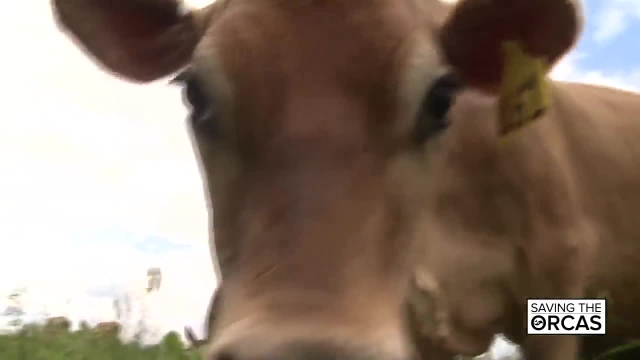 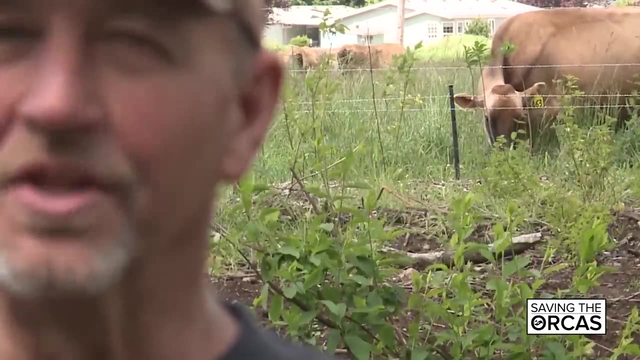 Jerseys are known as some of the best dairy cows, but they're also known for their personalities. Jerseys are very curious: If there's a gate open, it won't be just one, they'll all go. John Van Warregan's granddad bought the farm in 1936. 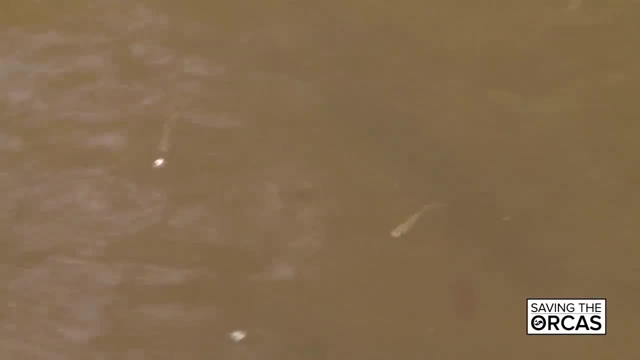 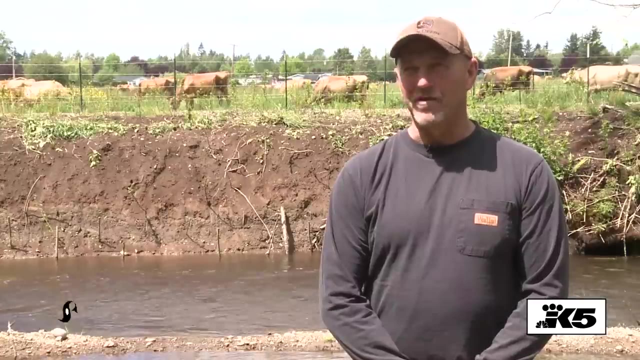 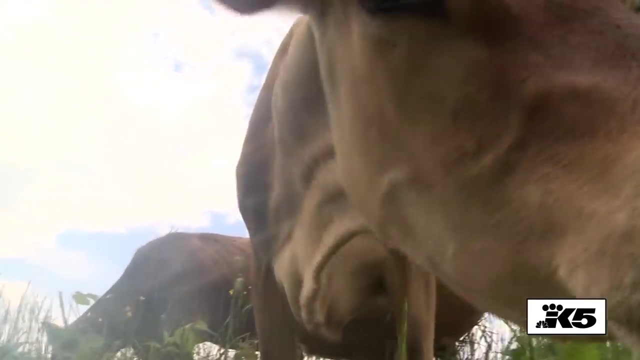 His father describes the nearby creek decades ago as full of salmon. I'd like to bring it back to that. The idea with doing this project was to make it so my grandkids' kids would be able to see that very thing. So the organic dairy with the curious cows is now the site of one of King County's latest salmon habitat restoration projects. 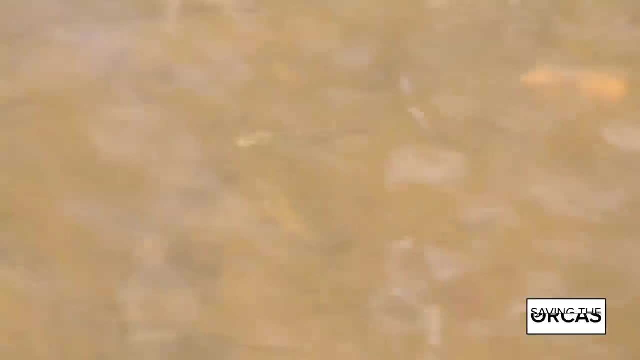 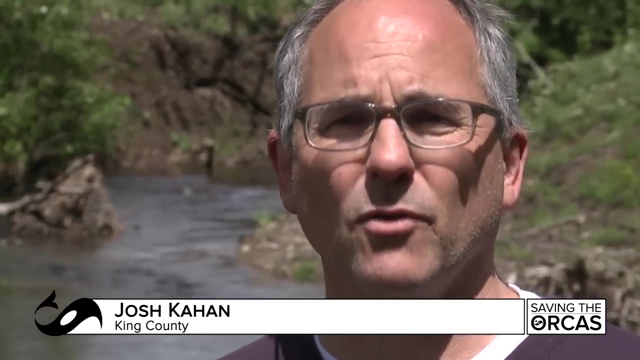 Crews excavated this side channel of Boise Creek, one of the most important habitats for wild spring Chinook. Boise Creek is the only stream in King County that provides habitat for spring run Chinook, which is one of the most rare runs of salmon in Puget Sound. 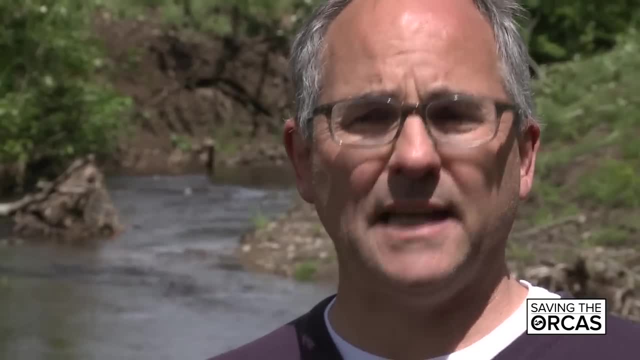 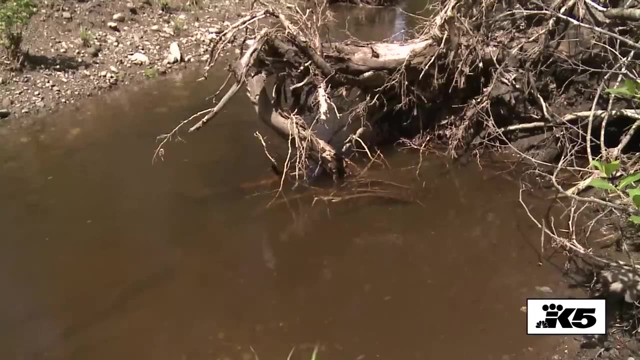 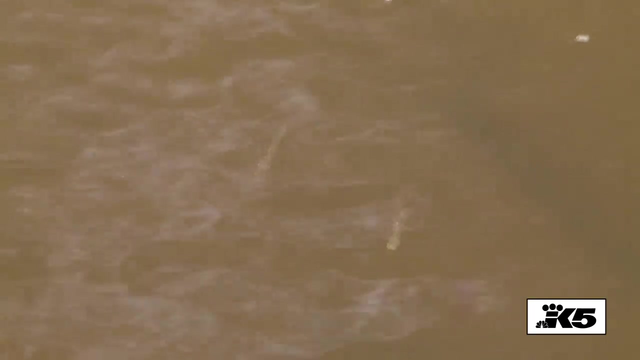 So we are very keen on restoring and enhancing the habitat in this stream in particular, so we don't lose that fish run to extinction. Josh Kahn says Boise Creek was channeled decades ago for agriculture and the water often moved too fast to allow young fish the time to grow properly. 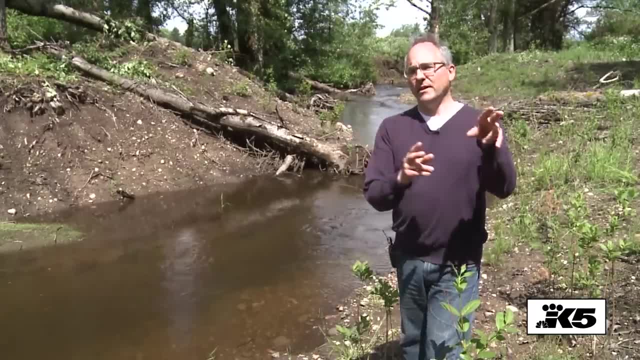 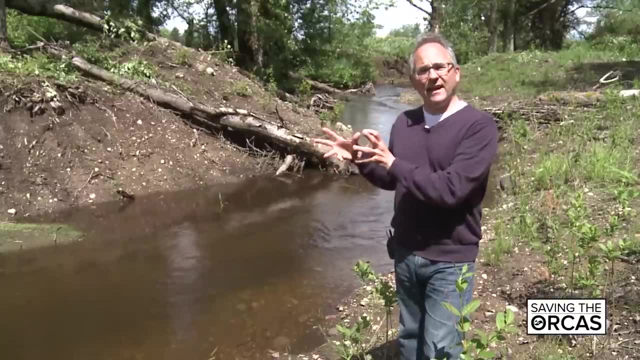 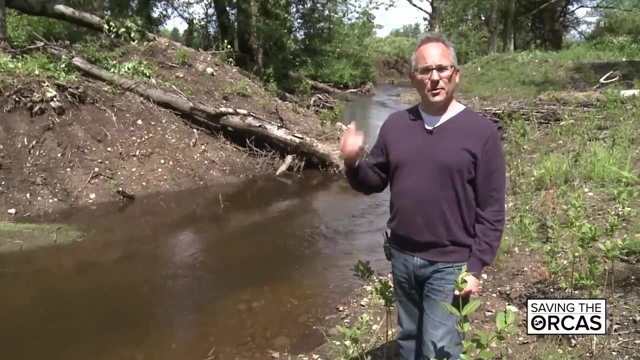 And if there were high flows they could get flushed out into the White River way before they were old enough to survive their migration out to Puget Sound. So having them stay in this stream system for as long as possible was really helpful to them in terms of maximizing their potential to survive. 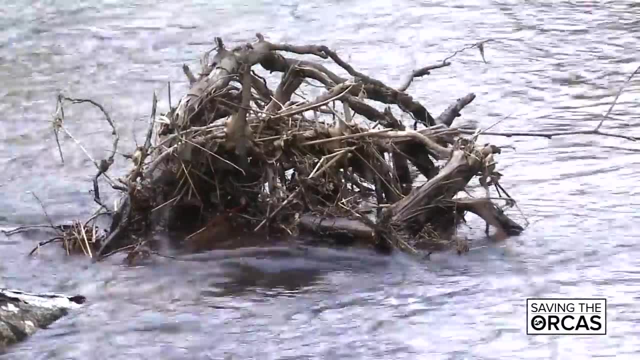 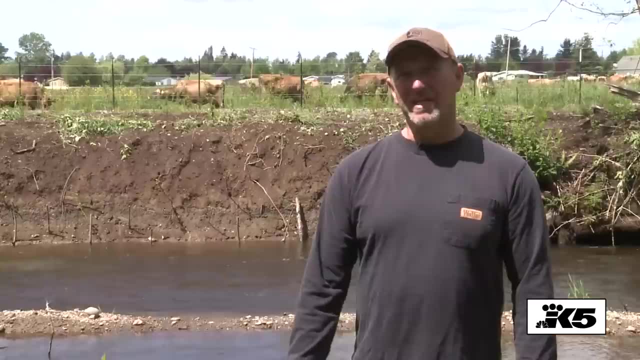 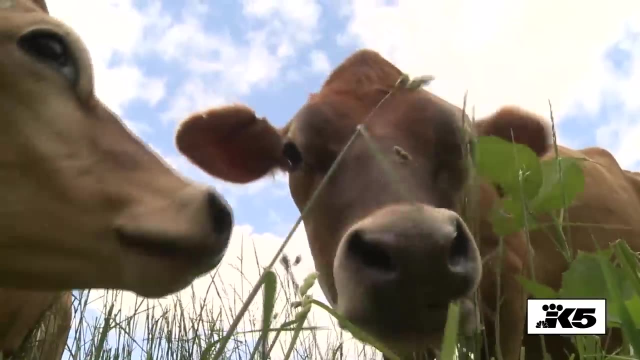 It's why projects like this are focusing on partnerships with farms and private landowners to restore hundreds of miles of land. We're trying to do everything we can to protect the salmon, protect the water, protect the ground that we farm, and hopefully this would show that that's exactly what we're trying to do. 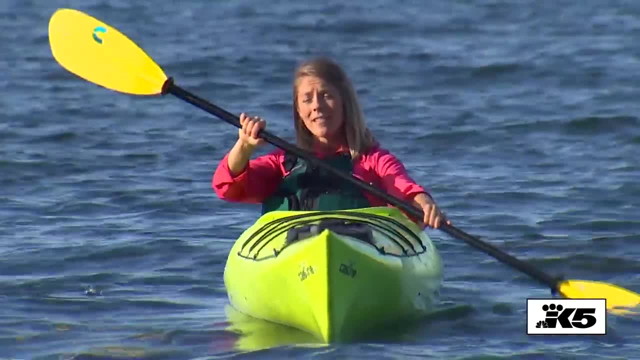 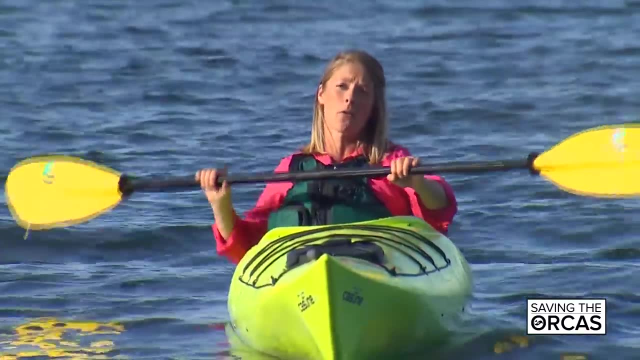 Habitat is not the only challenge facing salmon recovery. Seals and sea lions eat the fish and compete with the orcas for food, which has some calling for the killing of the marine mammals to save the orcas. One by one, they were all found dead. 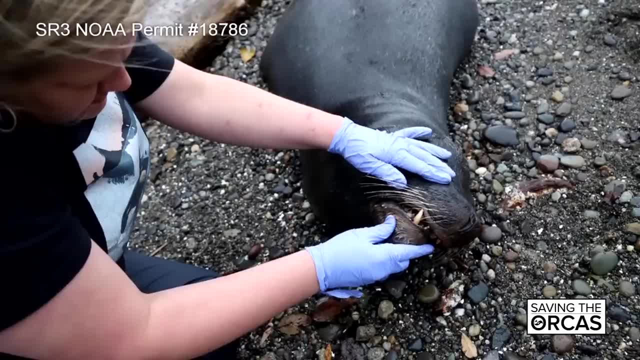 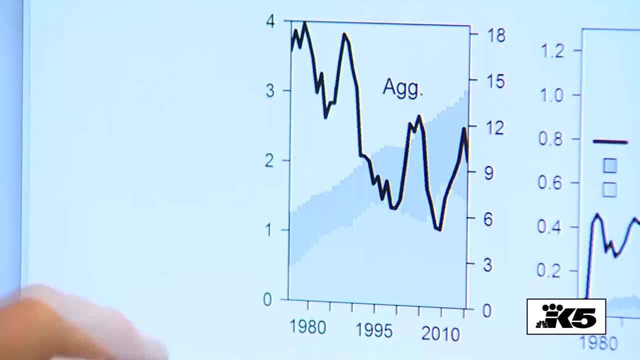 More than a dozen sea lions shot, many in the head, washed up around Puget Sound last year, mostly in West Seattle. Sea lions and seals are often seen as adversaries of fishermen. A recent paper published by federal scientists shows that in Puget Sound. 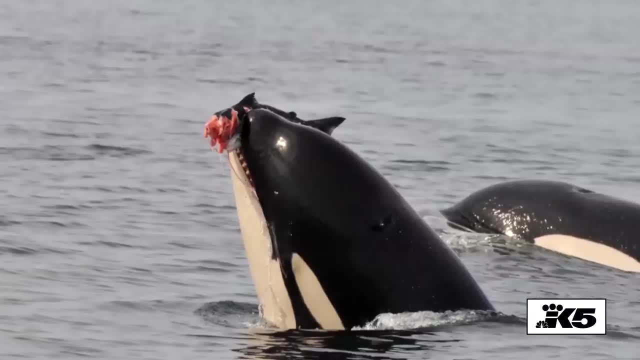 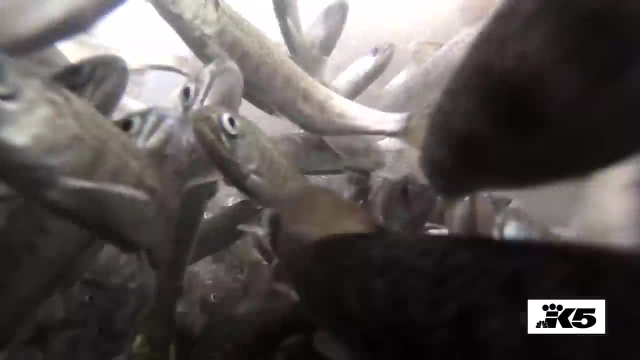 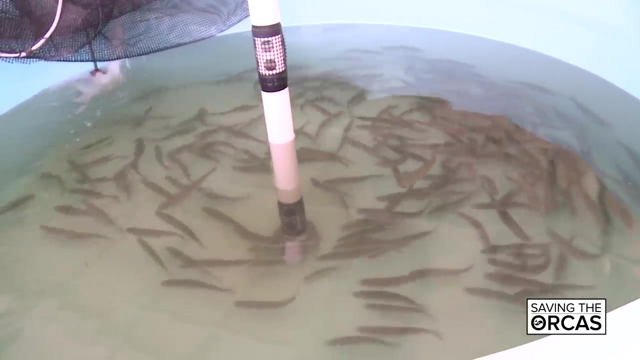 seals and sea lions eat twice as much Chinook salmon as southern resident killer whales and catch six times more Chinook salmon than recreational and commercial fishermen combined. Here at NOAA's Manchester lab, scientists are learning more about another kind of fish that may unlock new information to save salmon. 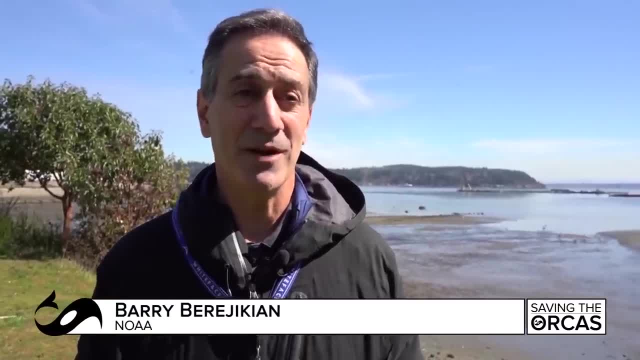 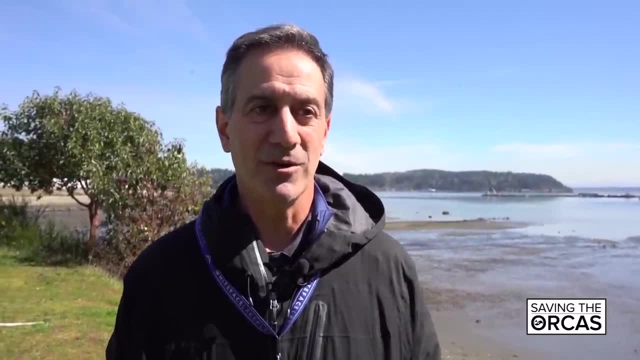 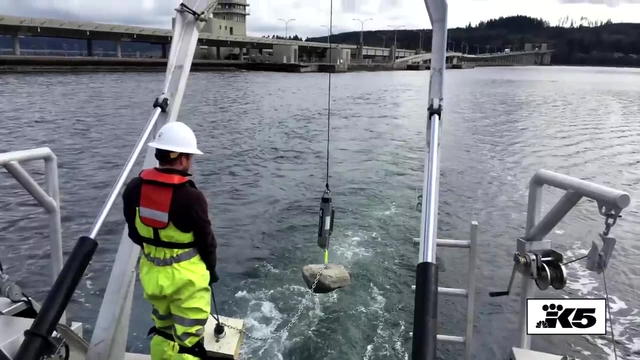 So we've been studying the survival of steelhead smolts as they migrate through Puget Sound and trying to figure out why they are dying as they make the brief migration from the river mouths to the ocean. Barry Berejeckian is a supervisory research fisheries biologist with NOAA's National Marine Fisheries Science Center. 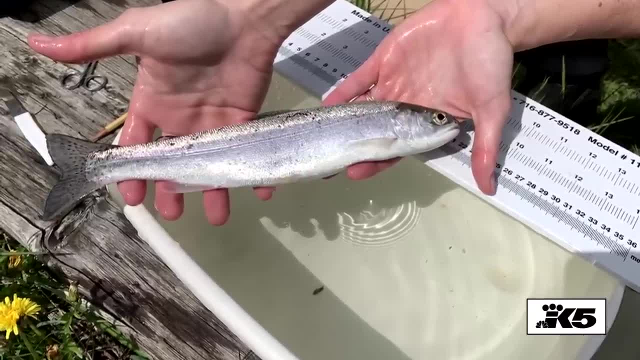 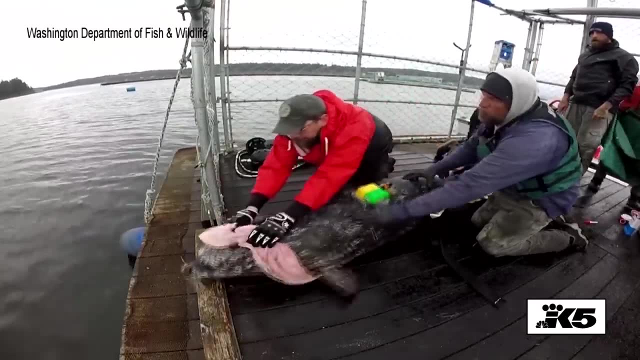 They've injected acoustic transmitters in steelhead that are detected by earphones on the floor of Puget Sound. They've also put detectors on harbor seals to see how they interact with the steelhead. In some cases they found the fish transmitters where harbor seals spend time on land. 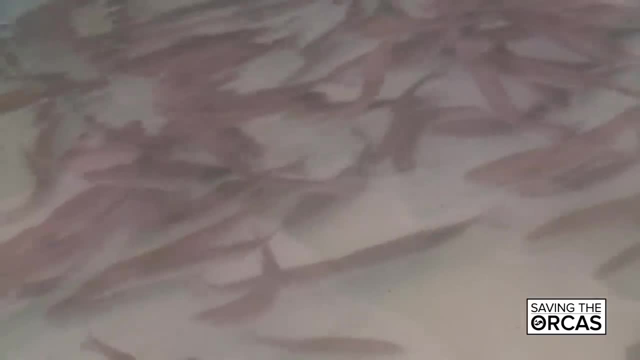 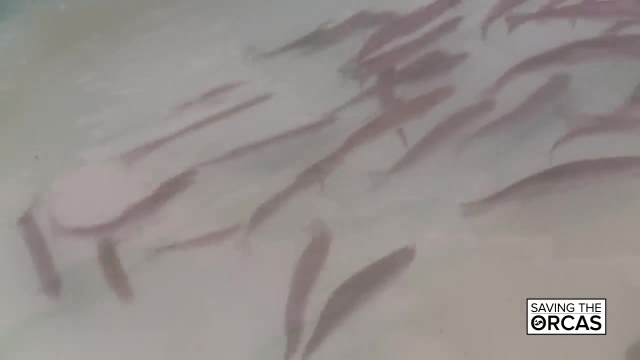 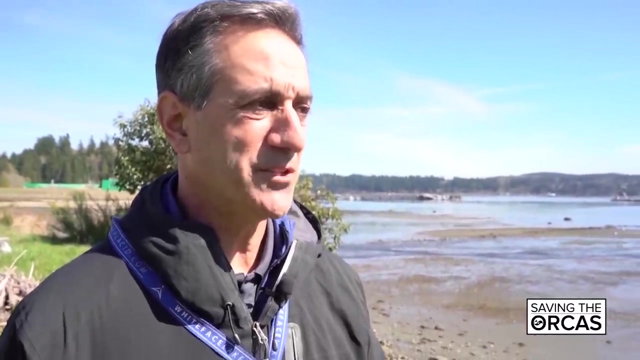 indicating they are eating the fish. But they noticed some years the seals ate more and some years they ate less, And the scientists believe it's connected to abundance of what's called forage fish And these other prey resources such as herring and anchovies and other bottom fish. 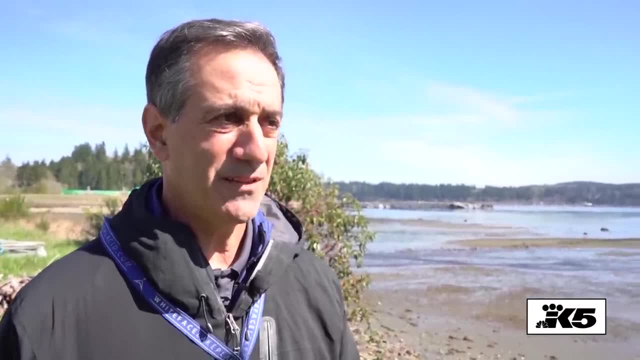 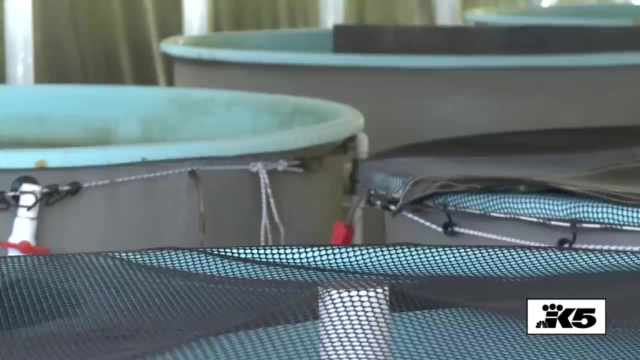 are much higher in fat and much more abundant, and so we think that seals and other things that prey on steelhead and salmon would prefer to eat those if and when they're abundant. At this lab, researchers believe seals and sea lions would prefer smaller forage fish. 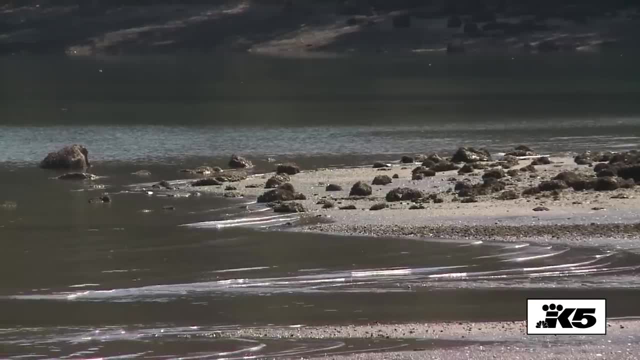 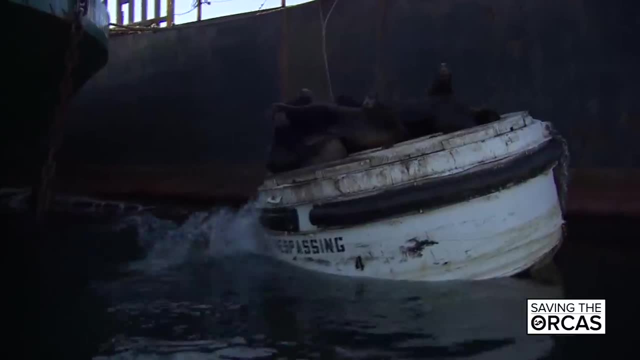 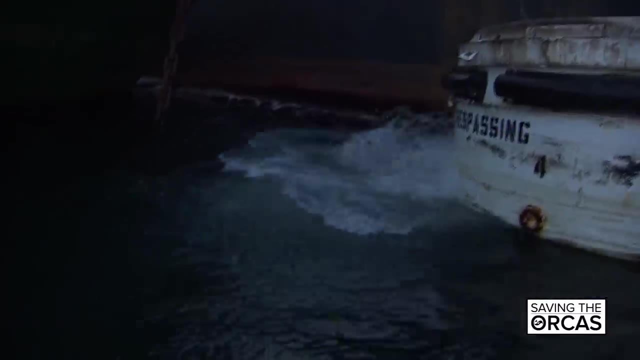 but those fish aren't always here. Berejeckian says they've started to see a connection between warmer water and an increase in anchovies, And when there are more anchovies, less steelhead are eaten by seals and sea lions. Essentially, what we're saying is that if we're right about this and that predation is greater on salmon and steelhead, 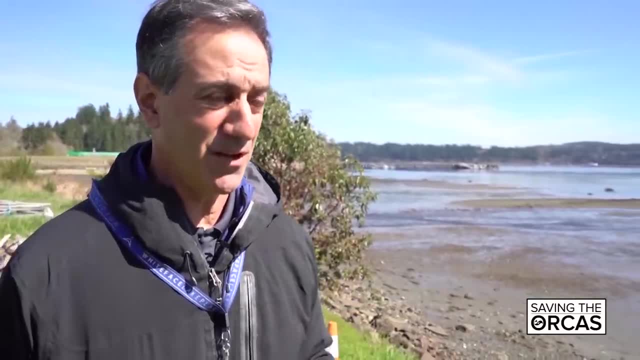 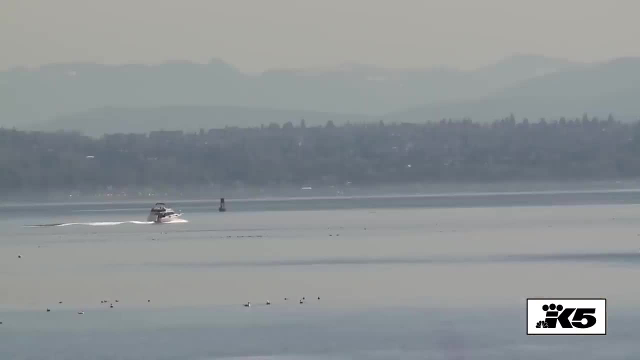 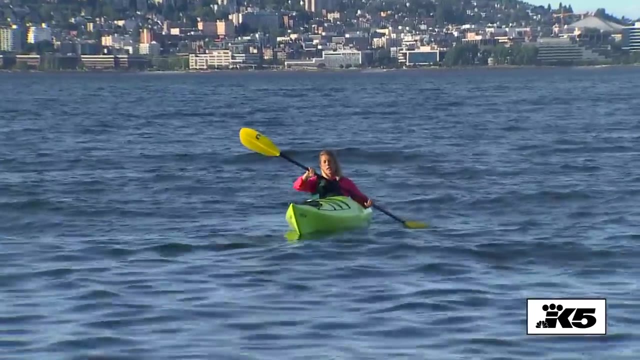 when other forage fish and other fish abundance is low, then really what we're talking about is restoration of the Puget Sound ecosystem to support these other prey species. While scientists are studying the problem of predators and habitat loss, hatcheries are producing more Chinook salmon to try to make up what's been lost. 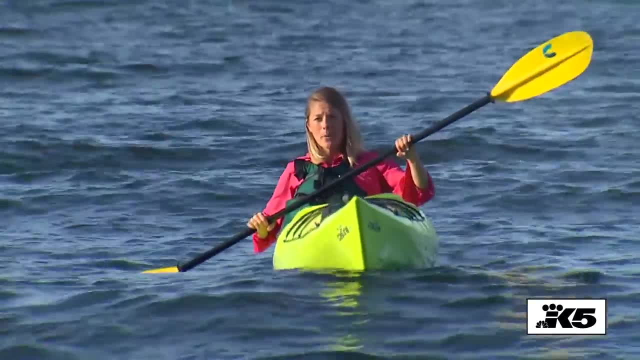 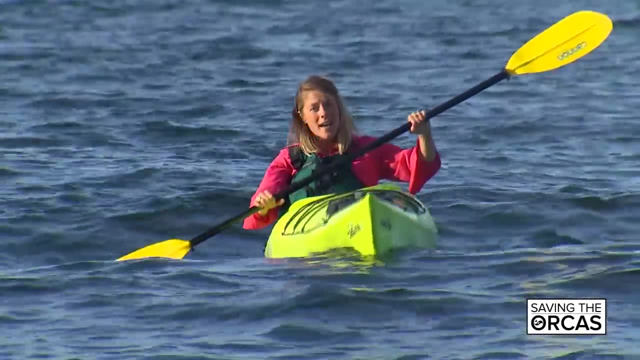 Governor Inslee has included $12 million in his operating budget to increase the amount of Chinook salmon produced at state hatcheries. But simply raising more fish is not enough. Hatcheries are having to change the way they operate to make sure more fish survive and make it to the whales. 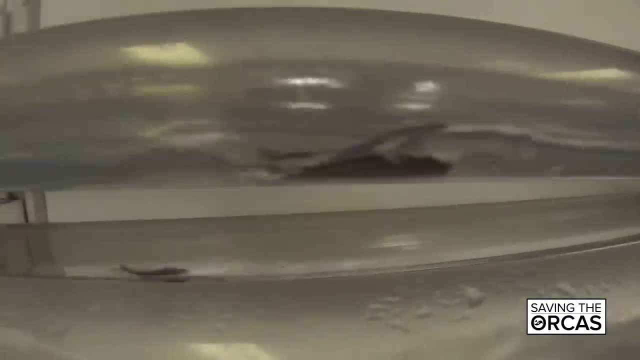 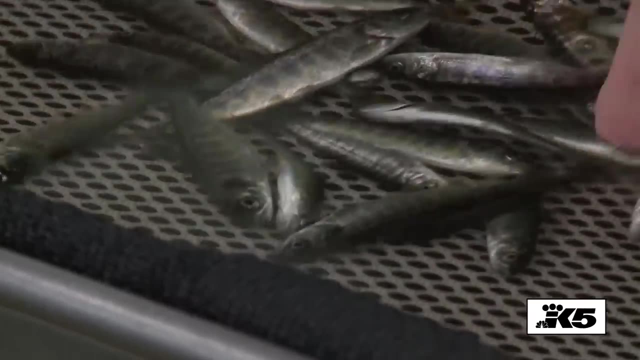 It may look like a water park amusement ride for salmon, but this is the way hatchery Chinook are marked for identification when they return to Puget Sound as adults. Their adipose fin is clipped and 200,000 of them will also be injected with identification tags. 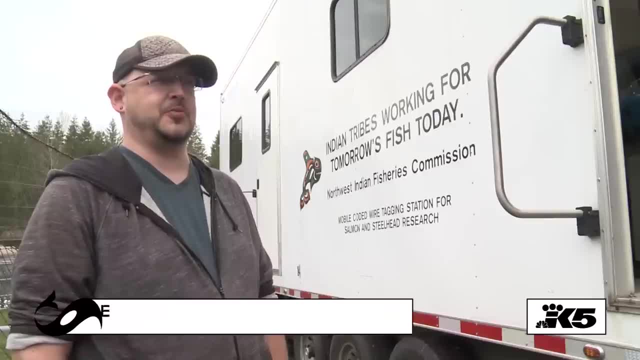 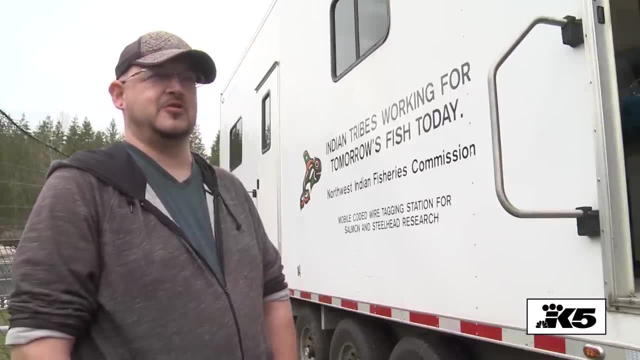 To solve the salmon problem is the same problem as trying to solve the orca problem. It's all interwoven. It's not just one piece that's going to fix this big, huge problem that we have: Lailup Salmon, Hatchery, Assistant Manager Jesse Rood and his colleagues. 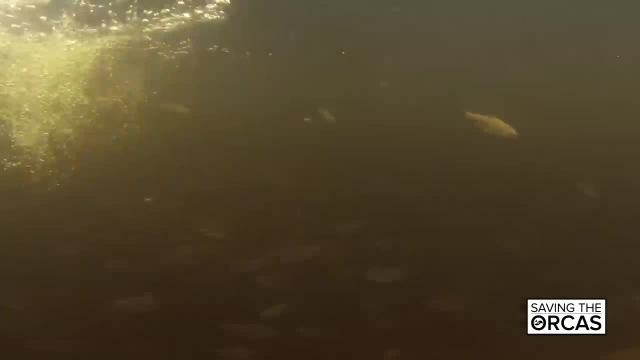 are working to improve the health and survival of the fish they release. Instead of releasing them all at one time, which is standard protocol, they're now experimenting with three release dates by changing water temperatures and how they're going to survive And how much the fish are fed. So we got three different programs- early, normal and late- And the earlies are going to be released here in a couple weeks. The normal group will be released in June and the late group will be released in August. Governor Inslee has included $12 million in his budget for increased hatchery fish production. And by the rate that they grow in the hatchery and when they're released, that can affect how many come back and how big they are. Like they might stay in the ocean an extra year and come back as a larger adult, and that's what we're trying to come up with. 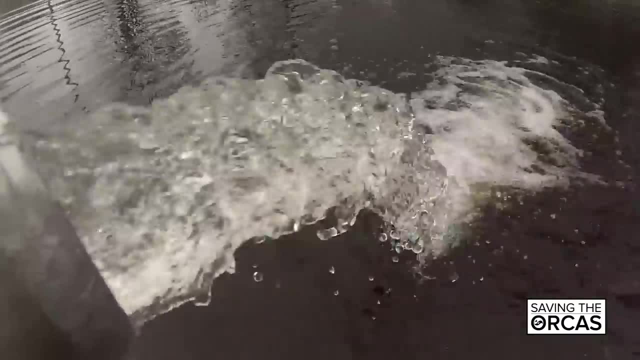 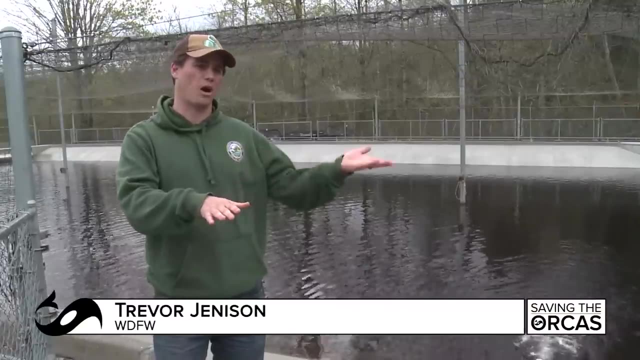 But studies have shown that hatchery fish can have a negative impact on wild fish if special precautions are taken: Making sure we're not just dumping fish into a system with a bunch of wild fish- and they're both competing for food- and just making sure that we're not outplaying anything. 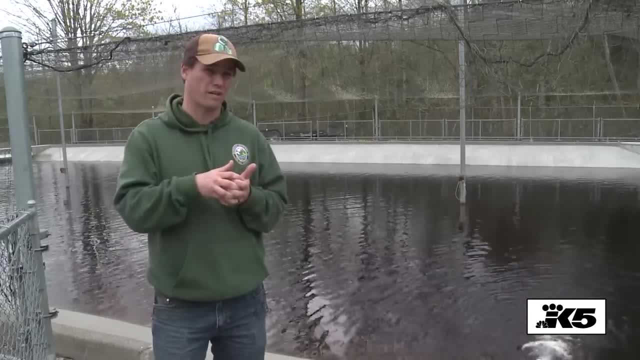 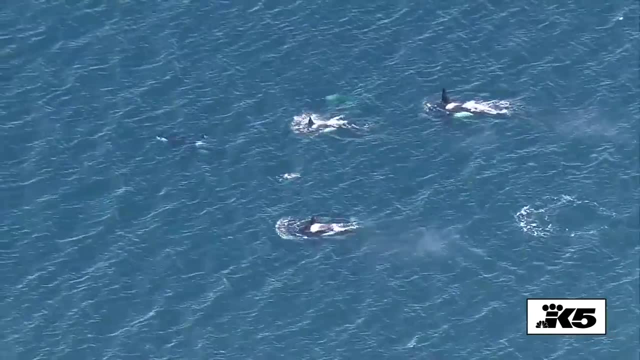 And if we are having an effect, what exactly are our effects, and are they adverse effects or is the effect not really creating any major issues? Trevor Jenison manages one of the state hatcheries, producing all that extra Chinook to help feed the southern resident killer whales. 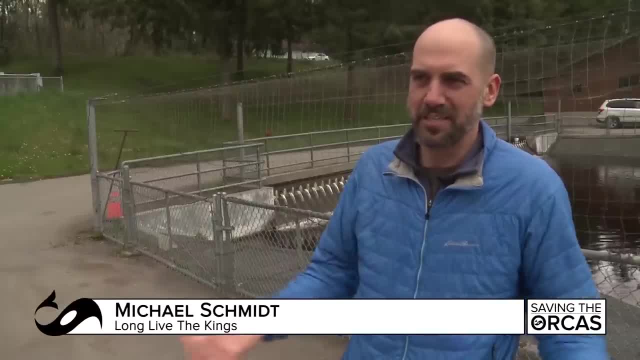 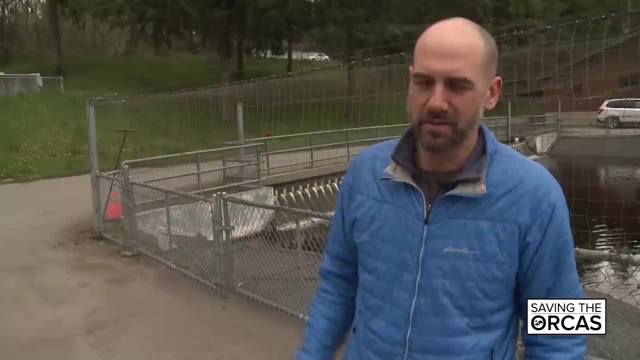 The fish that come back, they're 80% hatchery fish. right, It's just the way it is. And if we don't rear hatchery fish well and effectively, then we're not doing a service to the whales, to the fishermen, or anything. 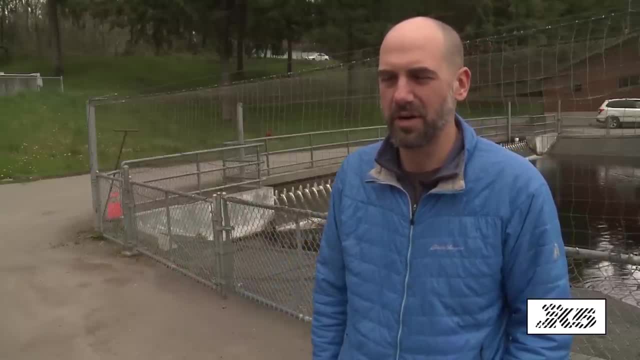 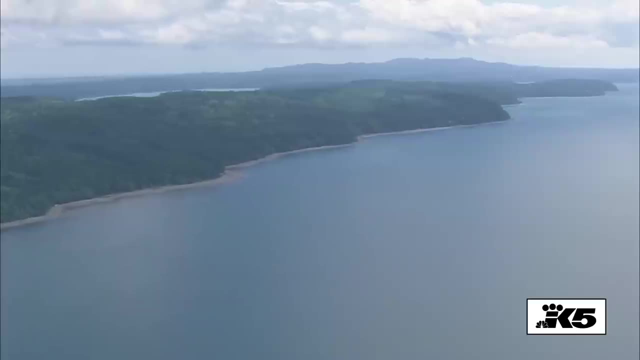 And at the same time, we ultimately want to get to the point where we have wild fish. Michael Schmidt is deputy director of Long Live the Kings, a group that's studying why threatened fish like salmon and steelhead aren't making it out of Puget Sound to the open ocean, where they grow to adulthood. 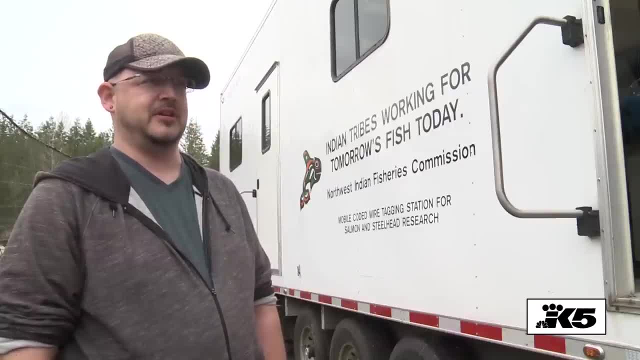 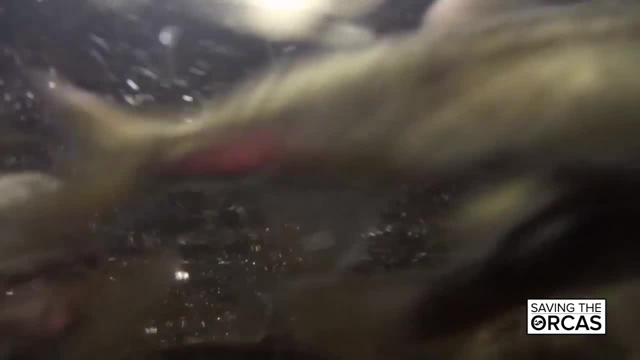 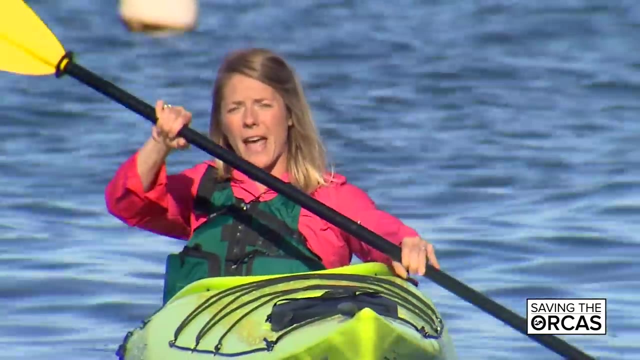 Salmon are the lifeblood of Tulalip, and that's who we are, So it's very important to each and every tribal member out here, because we are the people of the salmon. Some argue, though, that even if we produce more fish in hatcheries, it won't make much of a difference. 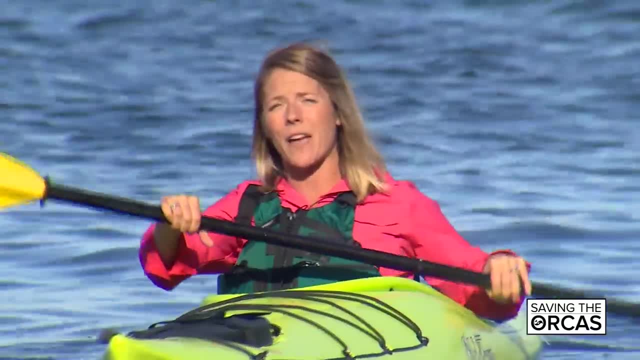 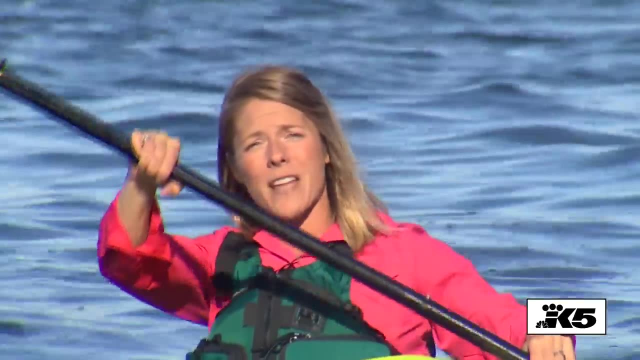 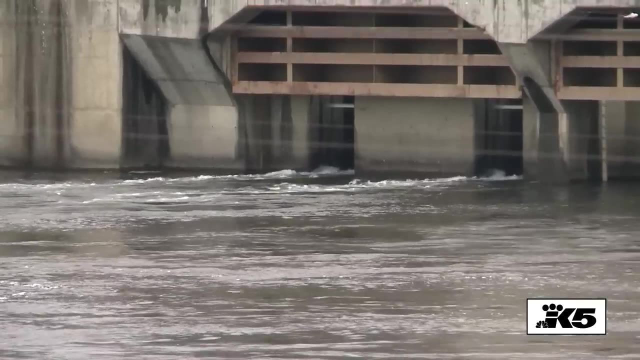 until we eat them, And that's why we take down barriers like dams that prevent fish from migrating up and down rivers, And one of the most controversial set of dams is on the lower Snake River. Those four dams are blamed for reducing salmon numbers on the Snake and Columbia River systems. 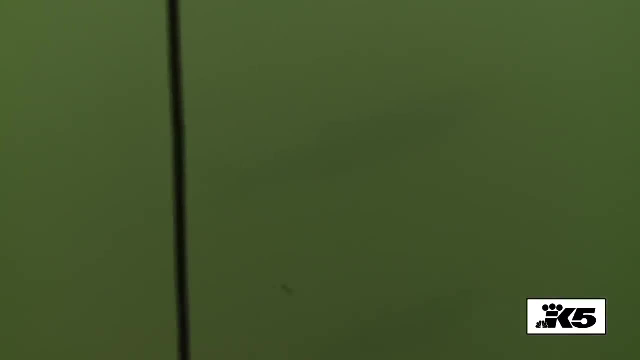 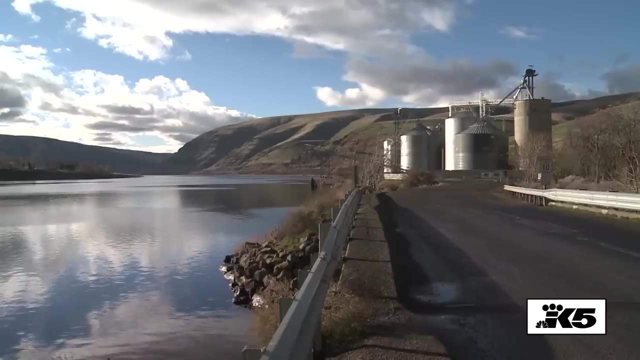 They slow water, which increases temperatures and makes young salmon more susceptible to predators. Critics say the dams are losing money and don't produce enough power to make them worth it, But the river system is used by wheat farmers to transport grain, and lawmakers in those areas have argued the dams should stay in place. 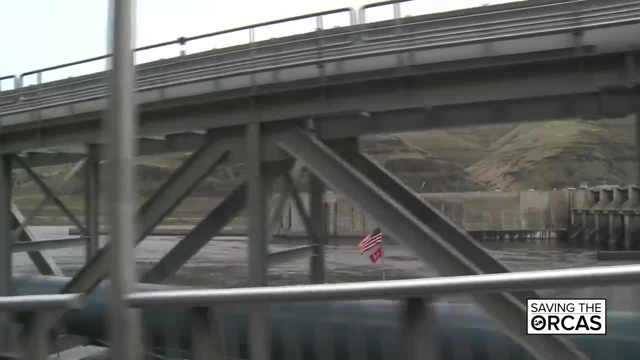 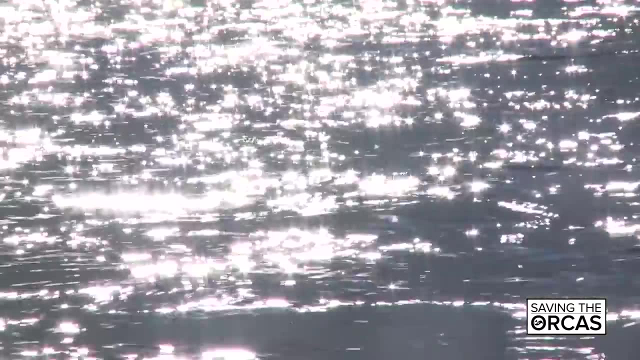 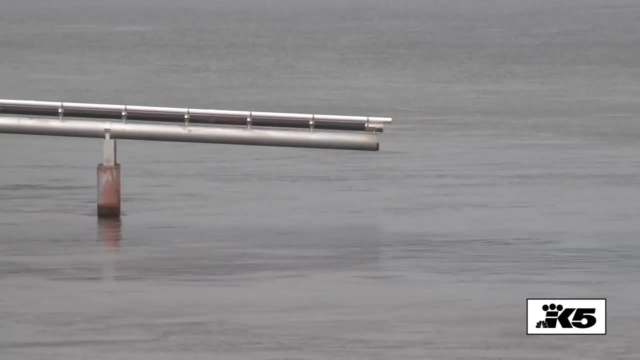 Governor Jay Inslee has signed a bill that provides $750,000 to study how to help impacted communities if the Snake River dams are breached. Both sides are critical of spending more money on studying the dams, but those who want to keep them say the decision is a federal one and the state is just wasting its money. 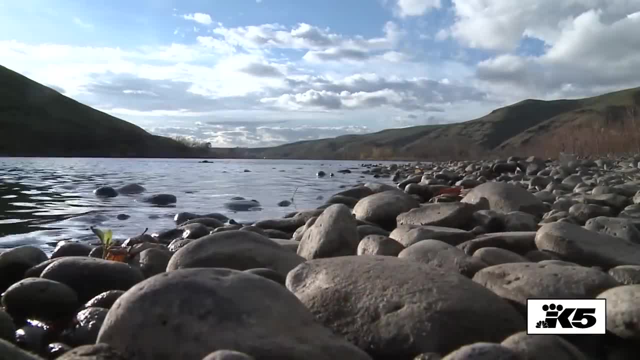 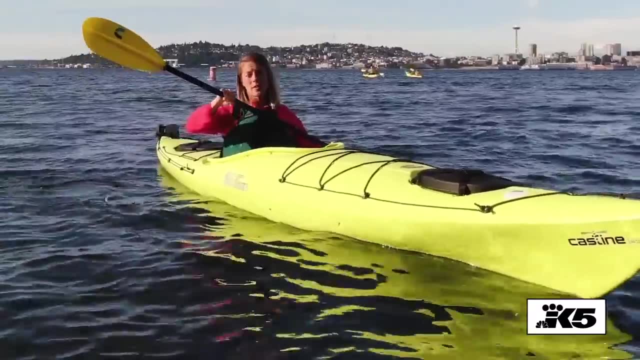 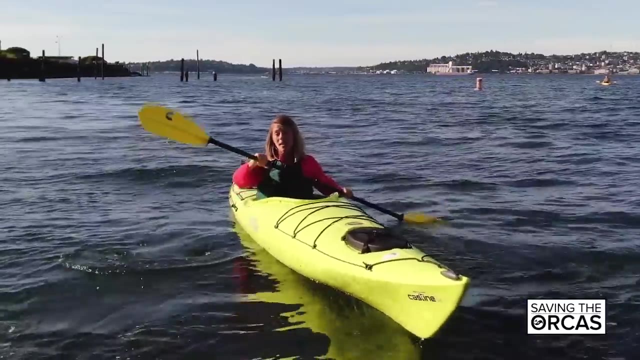 Those who want to remove the dams say there have been enough studies and no more are needed. While the Snake River dams have received the most attention, they are not the only dams that hurt salmon. In fact, right here in the Puget Sound area, there are several hundred miles of habitat cut off to fish because of dams. 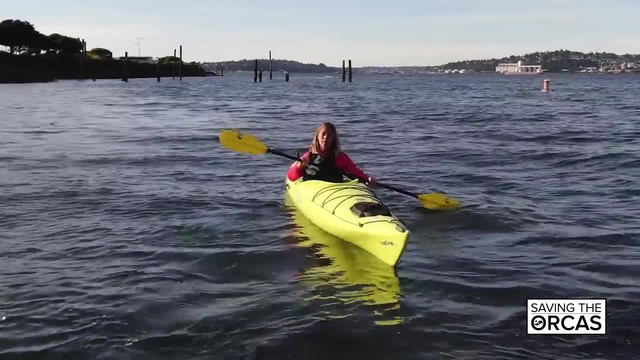 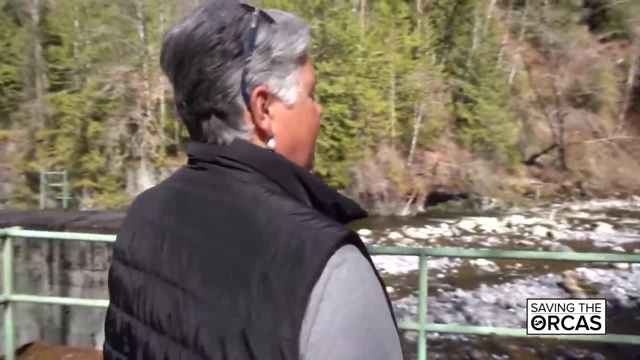 But two of them recently got a lot of funding to make some big changes. My dad was a commercial fisherman who ended up owning a fish processing plant up in Blaine For Bellingham Mayor Kelly Linville. this dam is personal. It cuts off salmon habitat at the middle fork of the Nooksack River. 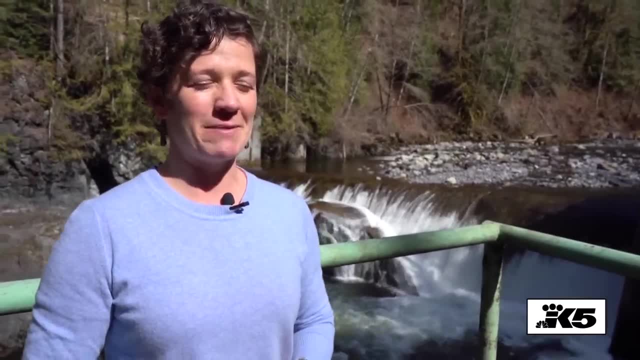 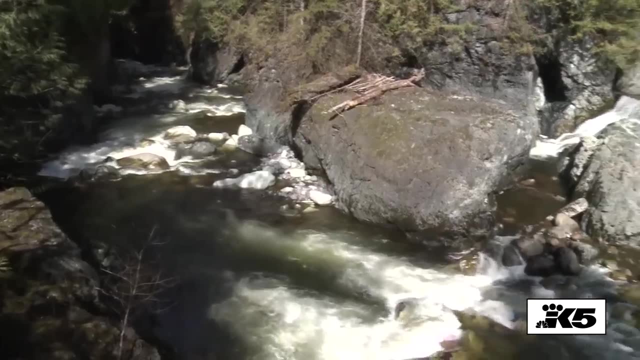 When the fish come up, they get to the dam, and they can't swim over the dam right, So they have to stop. April McEwen is the project manager for American Rivers, helping to spearhead work to remove the dam while still maintaining some diversion for Bellingham's water supply. It will open up 16 miles of historic habitat for salmon in clean, cold water flowing from Mt Baker. So it's going to be smart infrastructure that allows the water diversion to be maintained while we remove the dam. So we're going to then remove the dam. 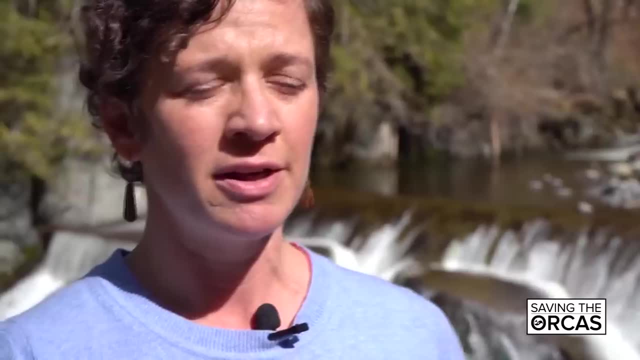 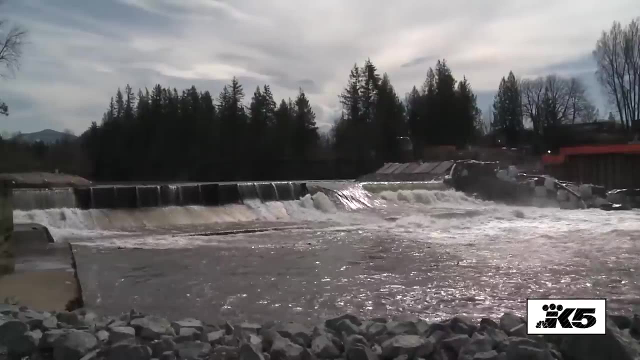 And restore access and fish passage. restore the channel through the site and restore access to upstream habitat. Here on the White River, salmon are getting a different kind of solution. Downstream from the Mud Mountain Dam will soon be the largest fish trap in North America. 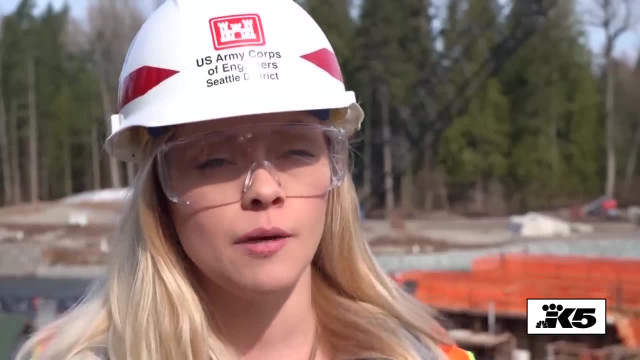 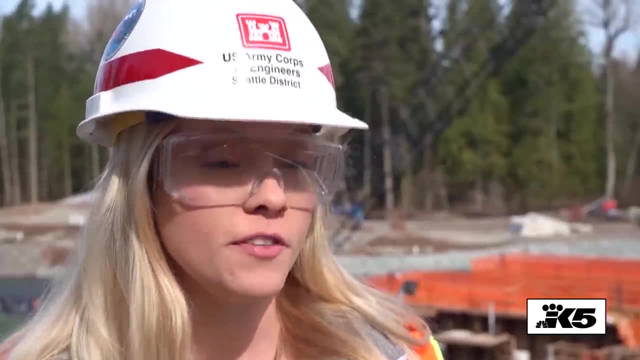 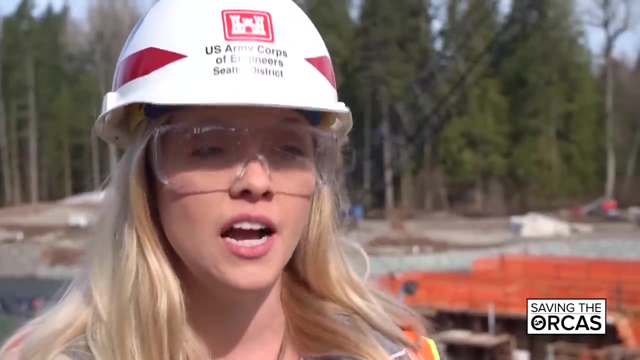 So the existing fish trap was designed to pass up to 20,000 fish per year. We've used it to pass more than that, but it still isn't supporting the massive number of fish returns that we're seeing yearly. So the new fish passage has been designed to pass 1.25 million per year and up to 60,000 fish per day. 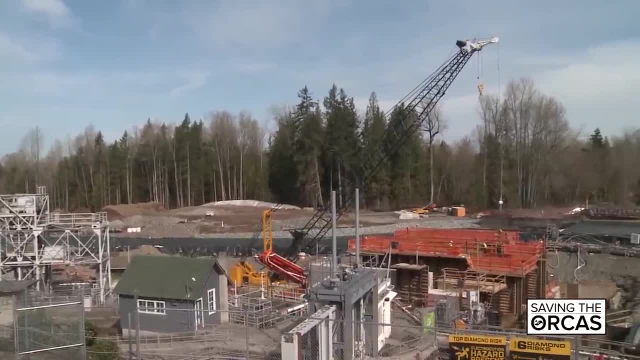 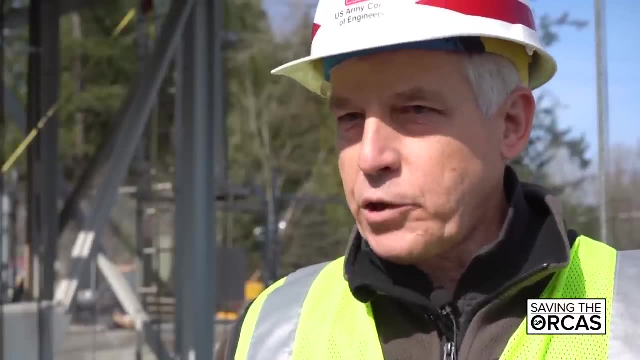 US Army Corps of Engineers, project manager, Leah Honstein says it was designed by more than 150 engineers from five different organizations. So if we didn't have a trap here with our dam, we would have a loss of tens of miles to hundreds of miles of habitat. 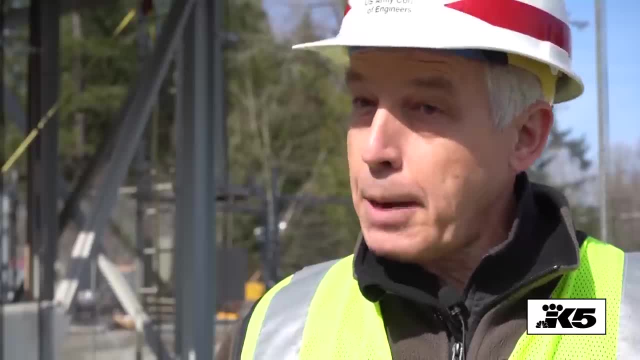 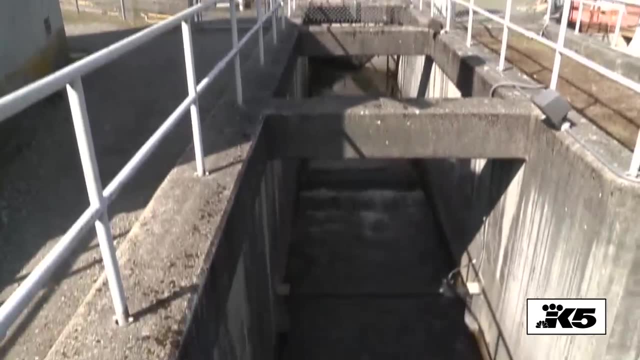 We would have fish runs that are much lower than they currently are, and they might actually go extinct. There may not be enough habitat for some of these fish. Fish biologist Fred Geffs explained how it works: The fish swim up a ladder and into the trap. 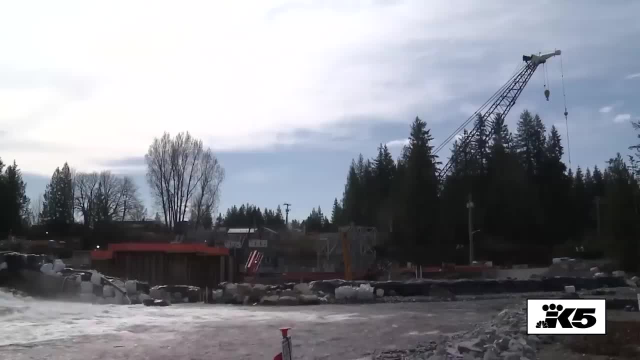 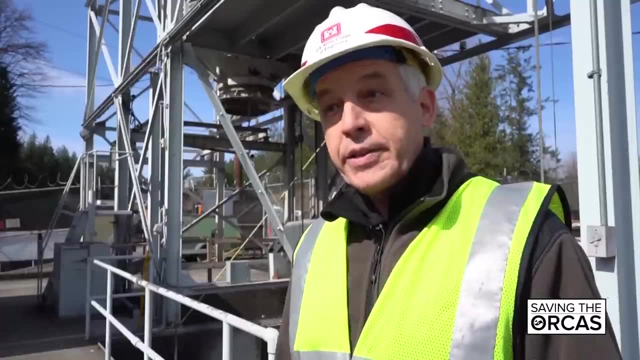 Then a truck will move them upstream and release them above the dam, again in an area with pristine water, perfect for salmon flowing off Mount Rainier. We are just one river basin of 14 that you'd find in the Puget Sound, But this is one of the most important basins. 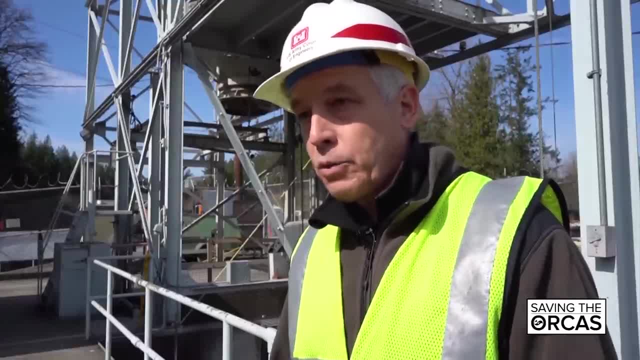 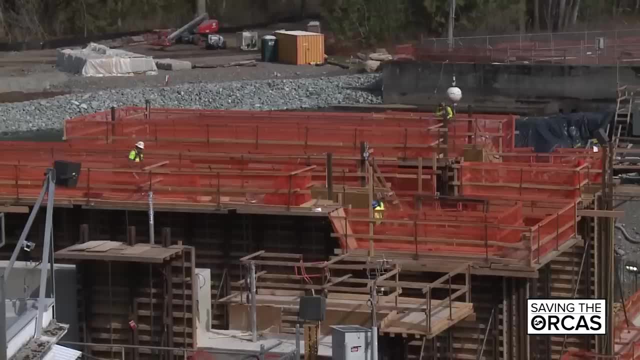 It's one of the largest. It has spring Chinook salmon, which is one of the preferred kinds of salmon that orcas eat. This project will cost $100,000.. This project will cost $112 million, but that money is already secured. 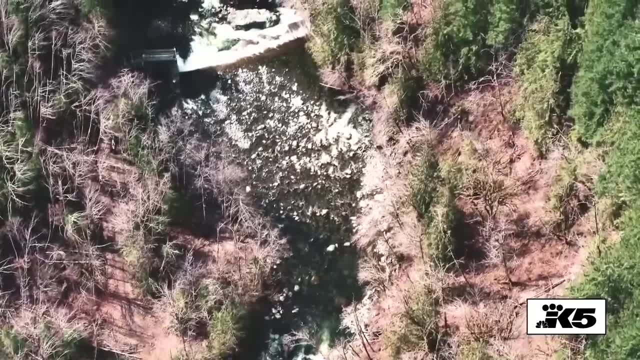 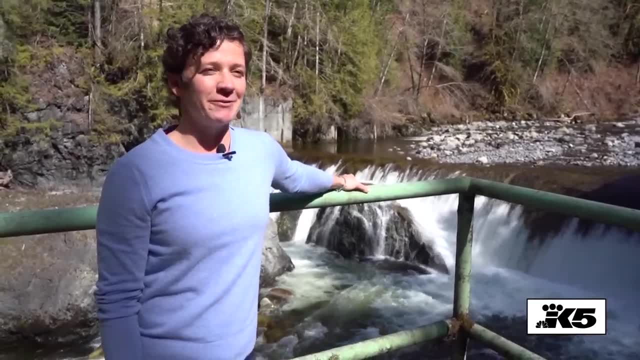 Back here on the Nooksack, though, funding is still unsure, as the project waits for state money And the state has said that this is a top priority project. So actions speak louder than words and we believe that the state will deliver on this. Critics of Governor Inslee's budget say it doesn't do enough for salmon habitat restoration, which they say could take 100 years if current funding levels aren't increased. Advocates for the project here on the Nooksack say it could increase salmon running. 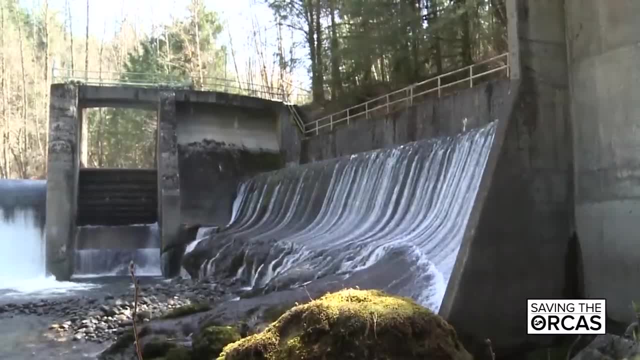 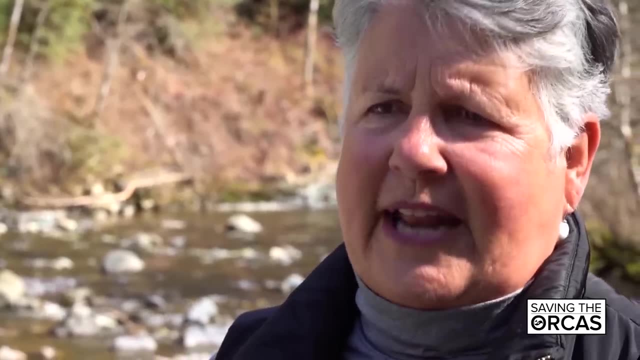 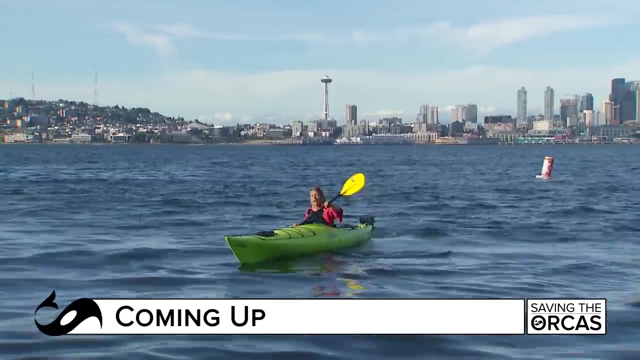 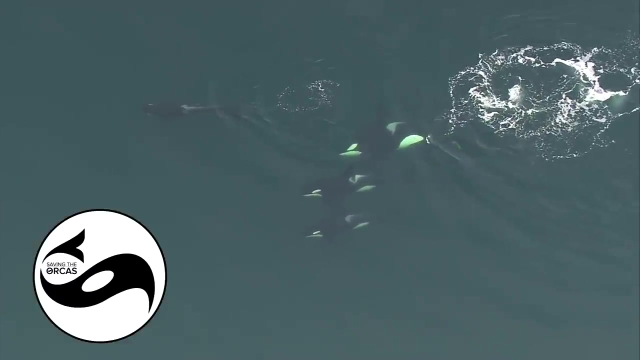 It's a great opportunity to not let generations of children think that every river should be dammed Up. next we'll show you how helping the southern resident orcas may start right in your own backyard. The problems facing the southern resident killer whales can feel overwhelming. 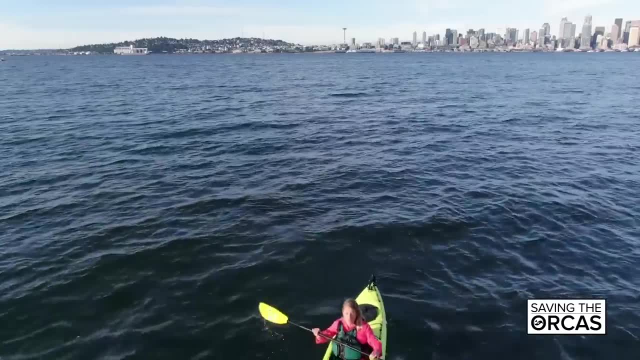 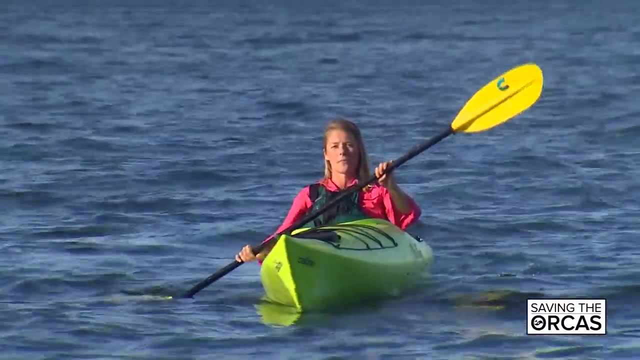 And it can be hard to imagine that regular people just like you and me can make a difference. But that's exactly what we're about to show you, And we'll start right here in West Seattle. You just look, for you know, like a fluttering tail in the water. 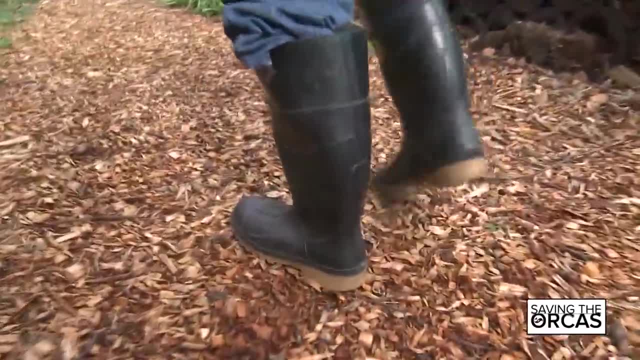 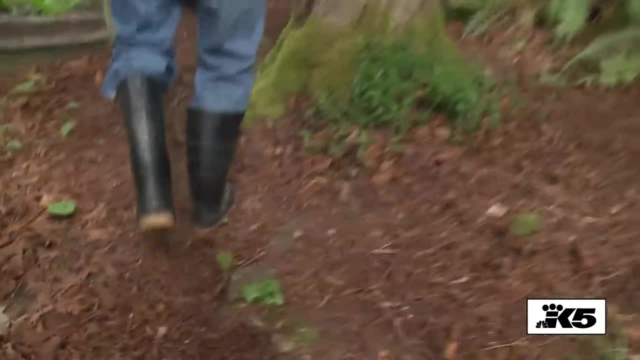 Or a lot of times they see you first and they'll dart around so you can just watch the water. Years of fishing have prepared volunteer Dennis Hinton for his daily checks of Fauntleroy Creek. I feel very childlike. I mean, I've been fishing for a long time. 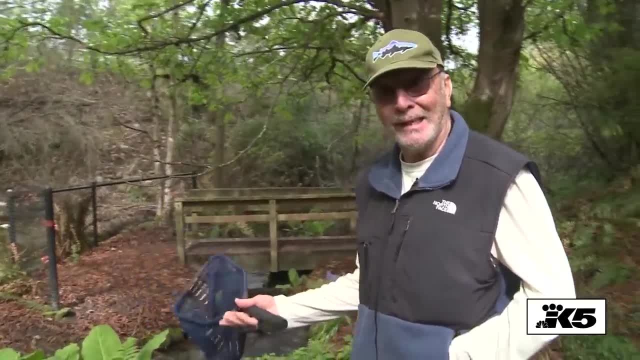 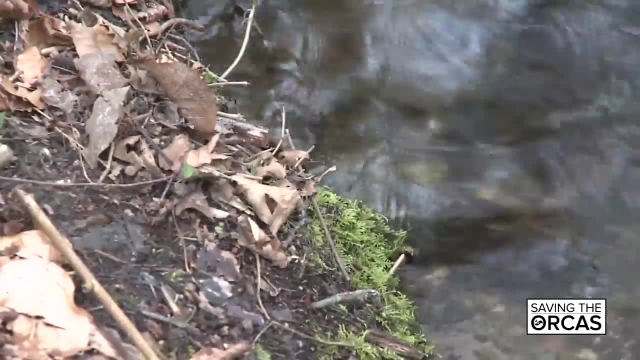 I've been fishing for a long time- I mean I mean really like a kid in a candy store. For decades the creek was essentially dead. It served as a drainage ditch with dirty water that fish couldn't even swim up. It went the way of many urban streams and became a dumping ground. 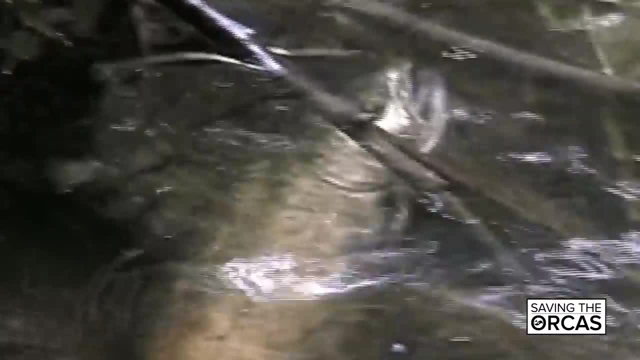 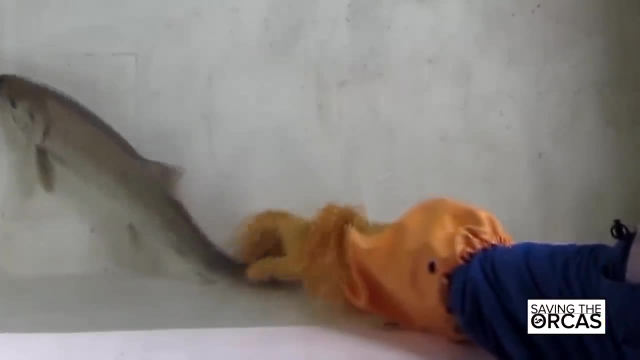 Urban storm water is lethal to coho salmon. This video shows what happens when coho are put in the toxic mix of runoff: They gasp for breath and eventually die. What happens in the ocean happens in the ocean. We can't do anything about it. 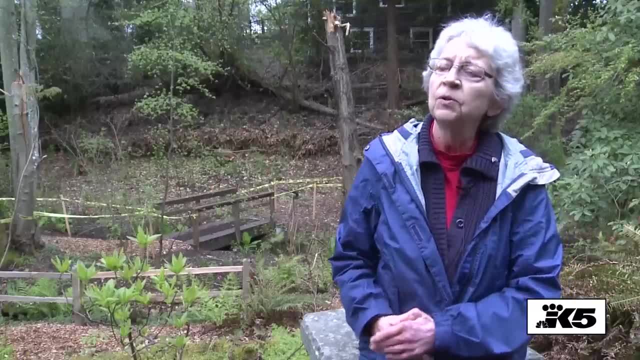 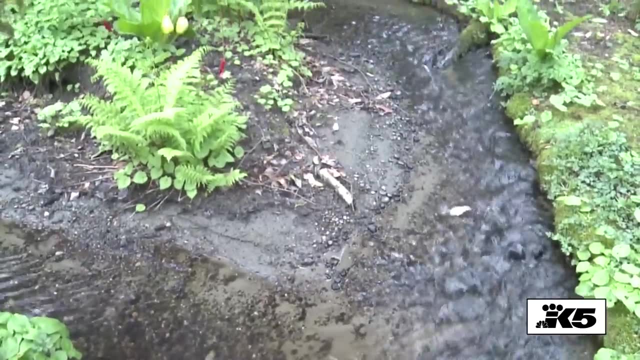 We cannot control it, But what we can control is the health of the habitat for juveniles. Judy Pickens bought the property several decades ago but admits she didn't initially want to get into salmon habitat restoration. Thanks to her willingness and a lot of volunteers. 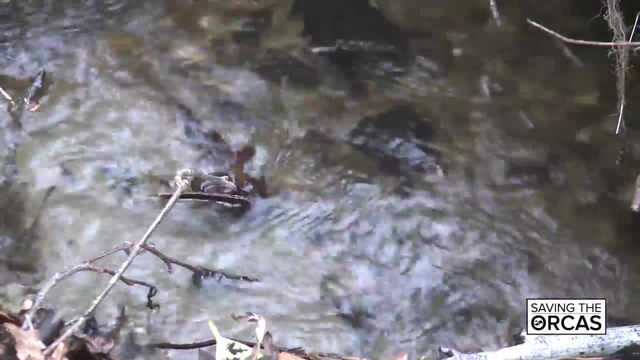 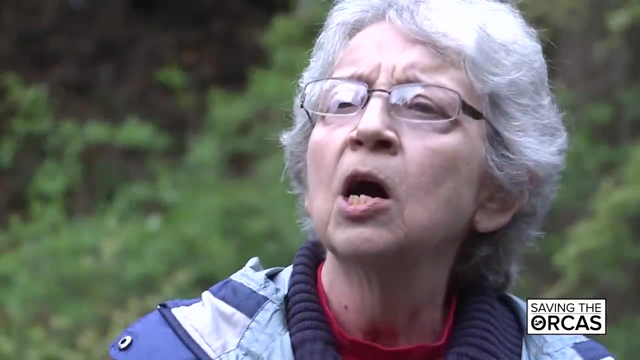 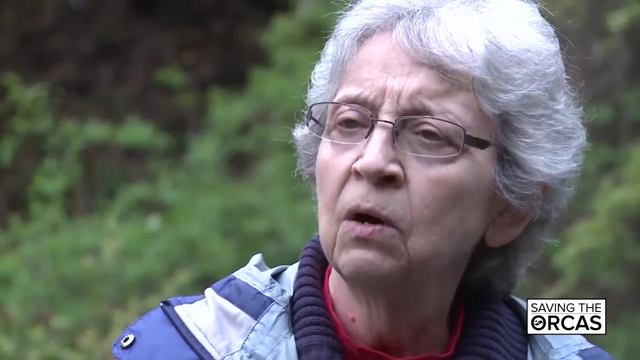 new vegetation, a fish ladder and other improvements have turned the once dirty drainage ditch into a creek that welcomes dozens, and sometimes hundreds of coho every year. They are great advertisement for the major, the major environmental work that is going on and needs to go on outside of the city. 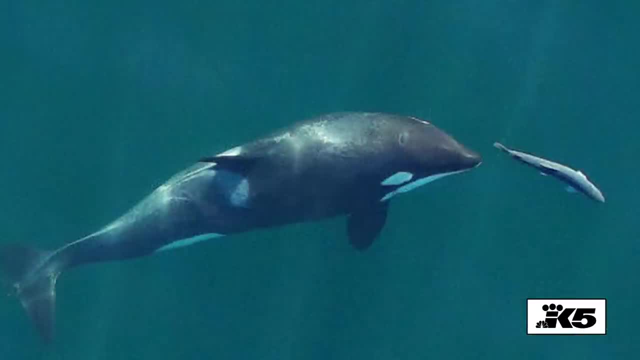 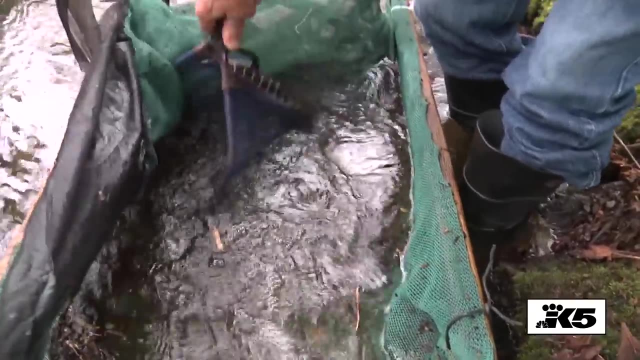 Though this creek is home to coho, it's chinook salmon that make up the main prey for the southern resident killer whales, But coho are often seen as an indicator for salmon health, which is why Pickens looks at the creek in her backyard as an important messenger for all salmon. 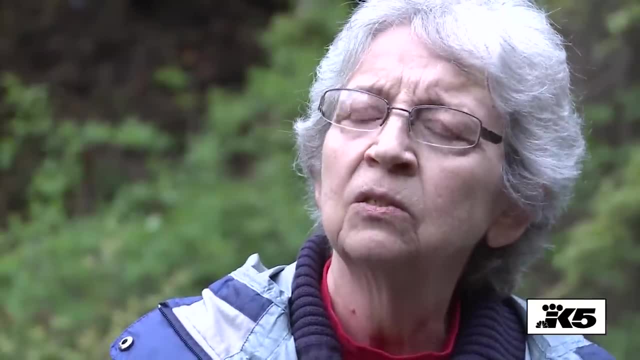 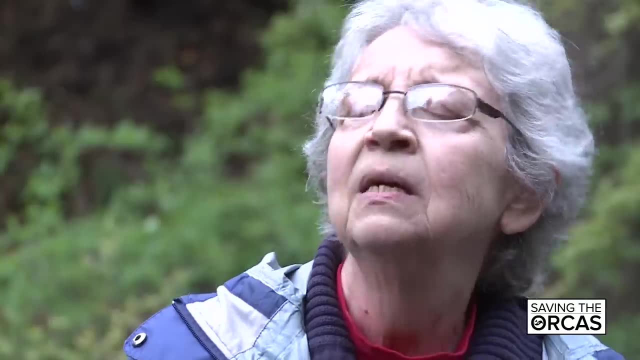 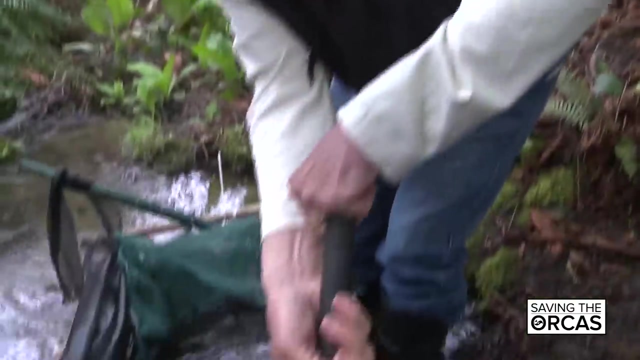 They will recognize that salmon are critical to orcas. whether those salmon are chinook or chum, It doesn't really matter, They're salmon. It's a simple message: Salmon are important. So how do we keep them here? So I'll do a couple of scoops here and see what we come up with. 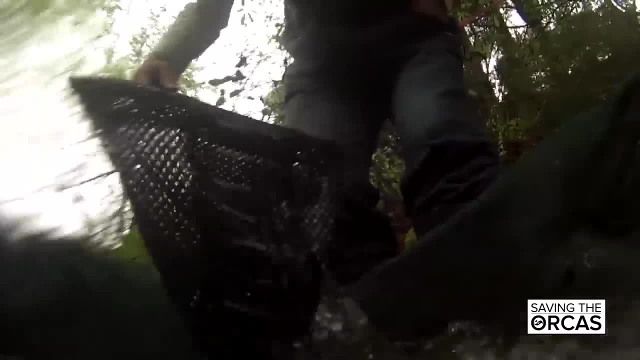 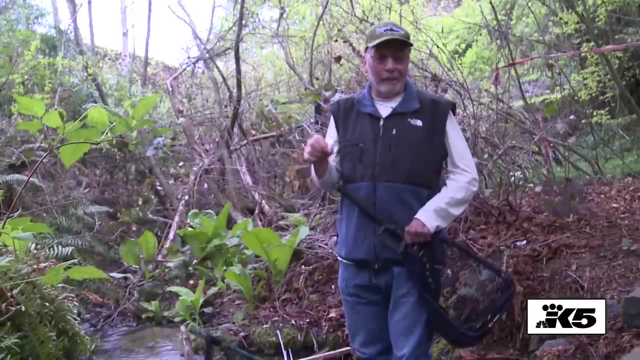 We didn't find any fish on our search, but Hinton will be back tomorrow, just like he is every day. This is not the Columbia River, obviously, But it's a little something that we can do, you know, and feel real good about and feel close to nature. 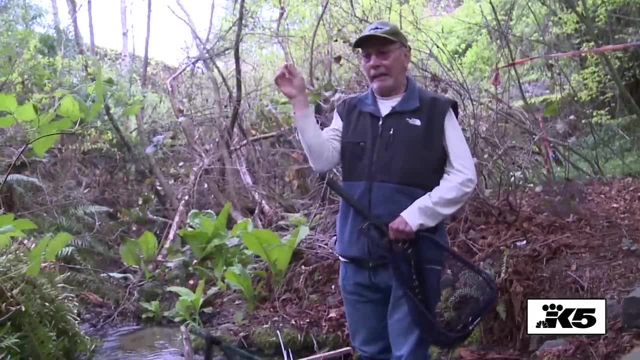 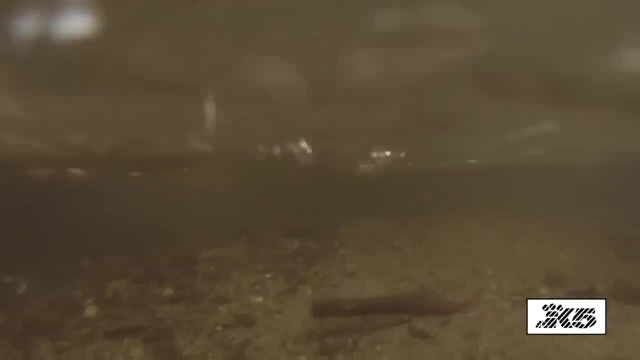 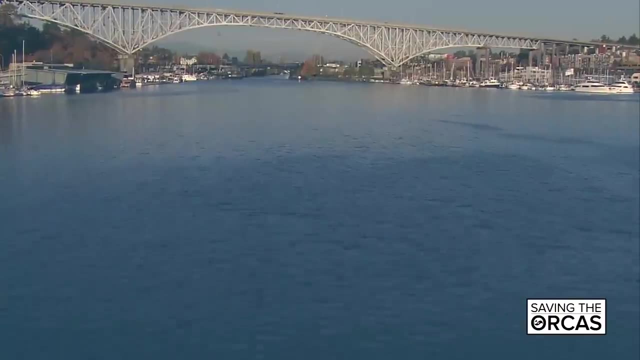 And in our own miniscule way, saving the world. you know, one fish at a time. Fauntleroy Creek here in West Seattle is a small urban waterway, but the ship canal that runs under the Aurora Bridge is huge. 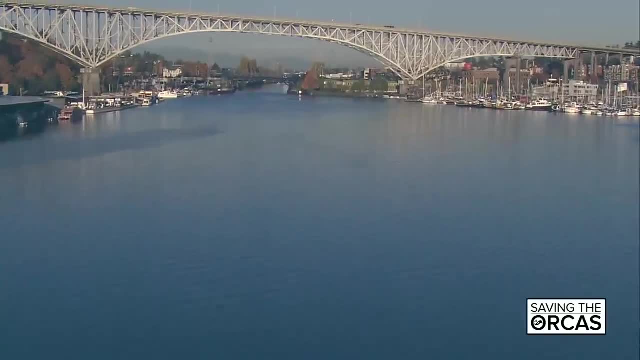 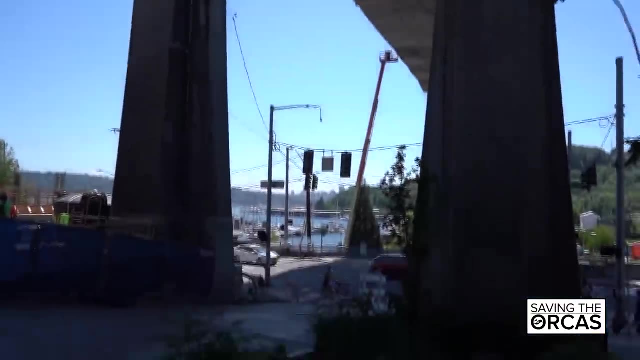 and the roadway above it is a real problem. The stormwater running off of it when it rains looks like coffee and it's toxic for marine life. But the area under the bridge is now getting wet. It's getting a makeover with rain gardens that trap and filter stormwater. 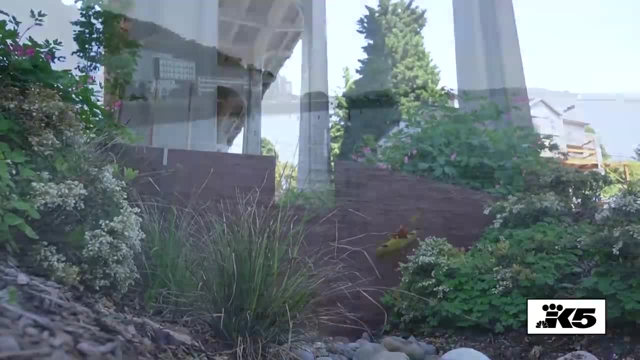 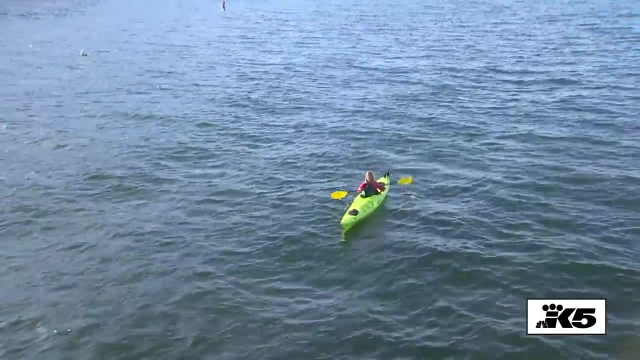 so that it is much cleaner when it finally flows into Puget Sound. Rain gardens are one of the main ways scientists say we can clean up stormwater runoff and reduce the amount of pollution in Puget Sound. that's hurting the orcas, And we're never too young to get started. 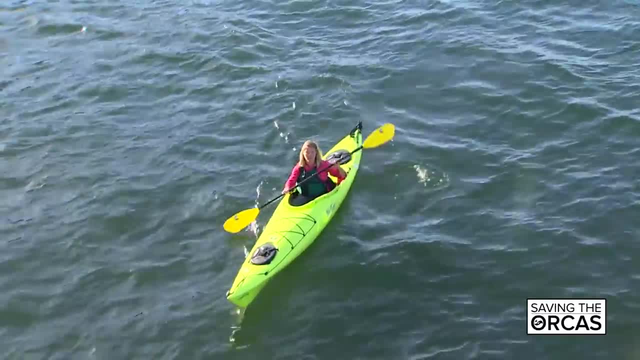 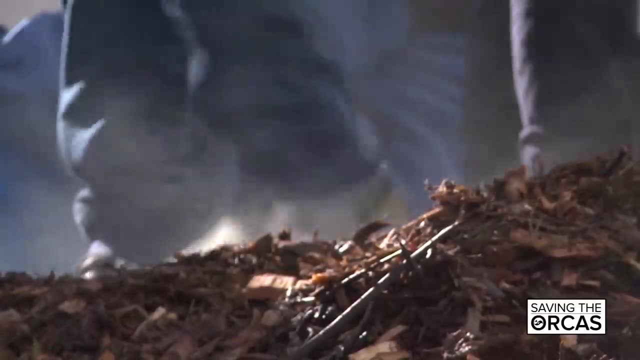 as one group of elementary school students in Tacoma recently learned: Careful, careful. It may look All right, good job guys, And even feel like recess. Kids like to play in the dirt. Kind of true, It's true. 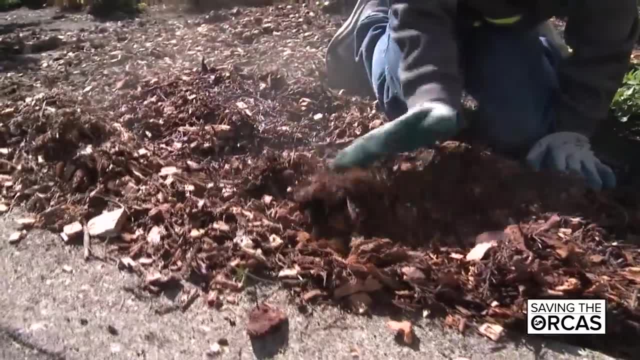 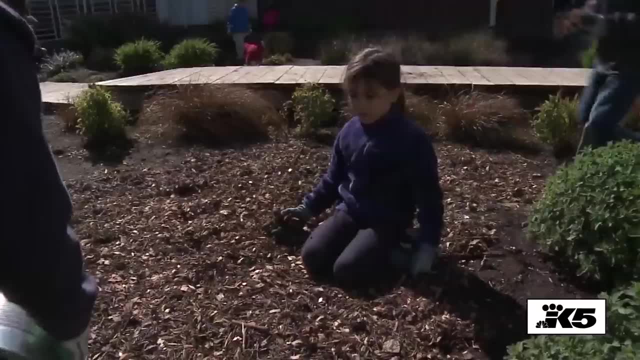 But this group of students at Sherman Elementary School in Tacoma is working on a class project. We shred it like this: They're building a rain garden with the help of a couple adults. Mulch is an important thing to keep the weeds from growing. 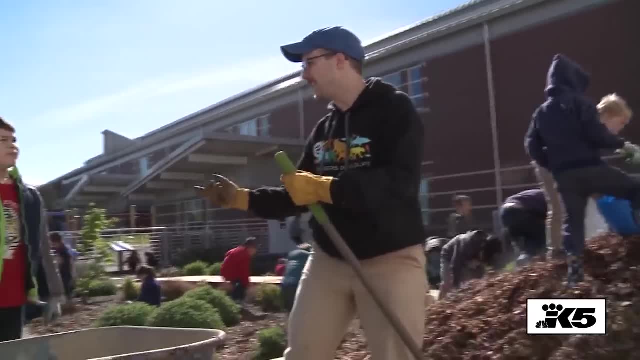 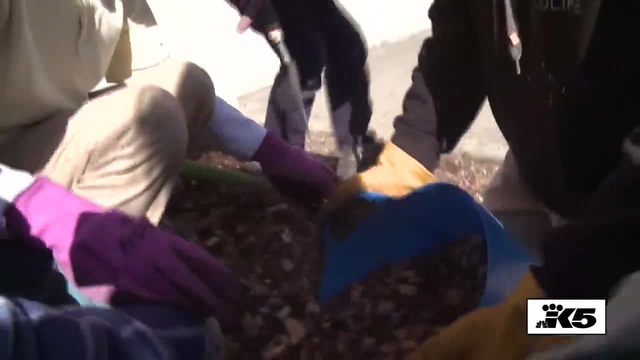 It keeps moisture around the plants. And why do we like rain gardens? Because they help orcas. Because they help orcas. Yeah, Rob Crable is with Defenders of Wildlife, and this frenzy of digging in dirt is part of a program called 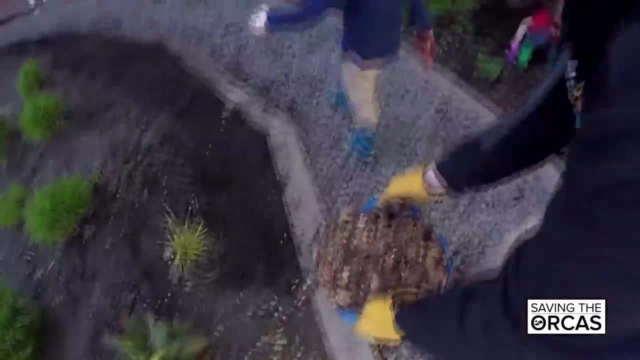 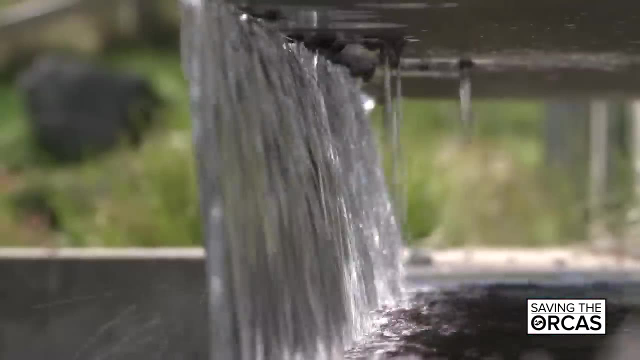 Orcas Love Rain Garden Right here. Okay, It'll filter stormwater runoff from their school's roof and keep it from flowing down drains and into Puget Sound, Just like this rain garden, the largest of its kind in the world right now. 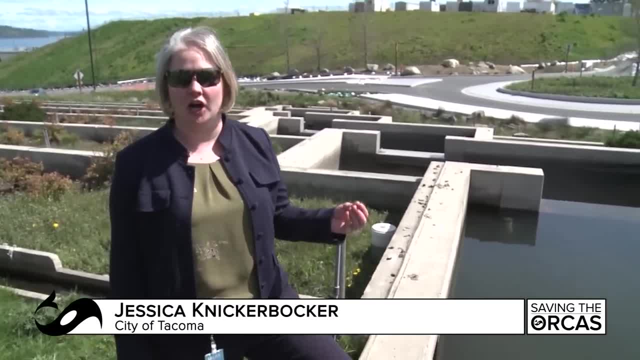 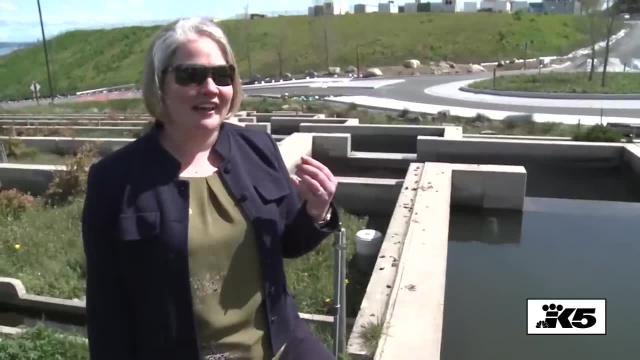 When it's raining, this fills up and it's black like tar, And if you were to touch it it's sticky at times, to the point of one day I might have done that and had to wash my hands three or four times to get the stickiness off of it. 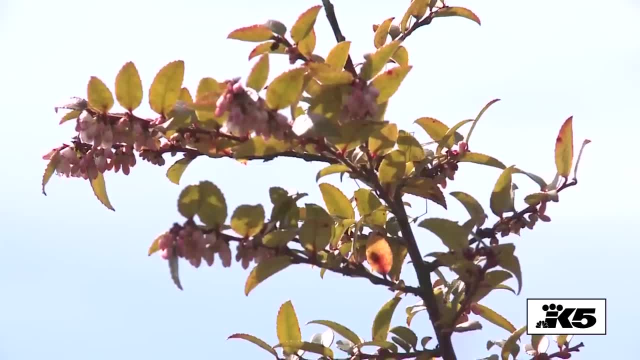 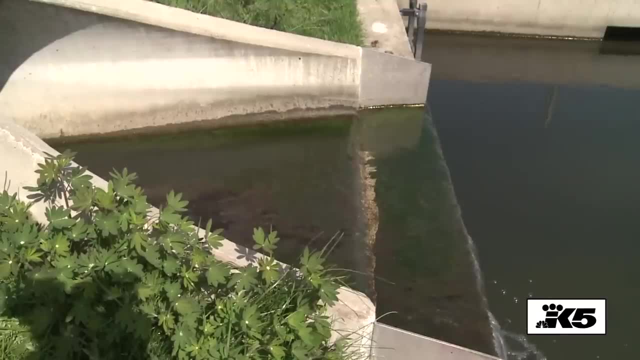 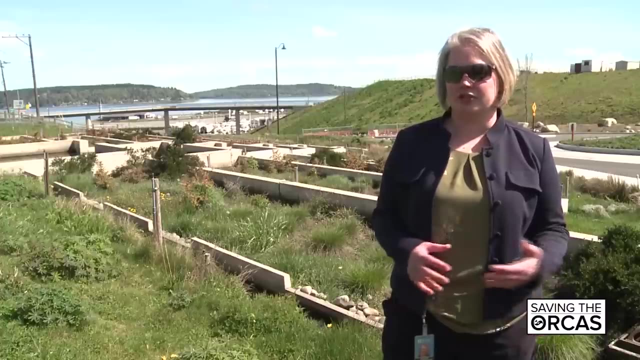 Jessica Knickerbocker spearheaded the construction of the Point Defiance urban rain garden, which filters stormwater from 750 surrounding acres. On an average rainy day, that adds up to 8 million gallons of filtered stormwater. Most of the city of Tacoma doesn't provide water quality treatment. 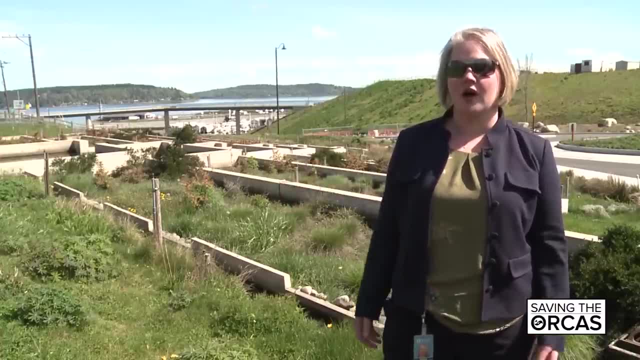 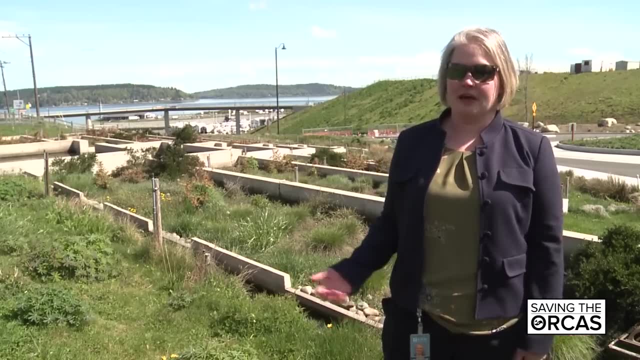 of its stormwater sewer before it goes into Puget Sound. So all of the dirty contaminants from our roads and cars and homes goes basically in our pipes and out to Puget Sound untreated. The rain garden at Sherman Elementary is smaller but no less important. 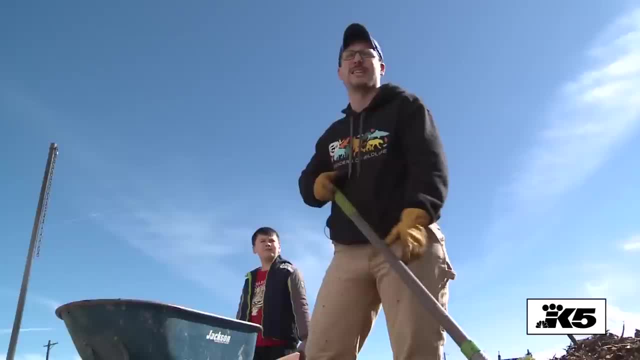 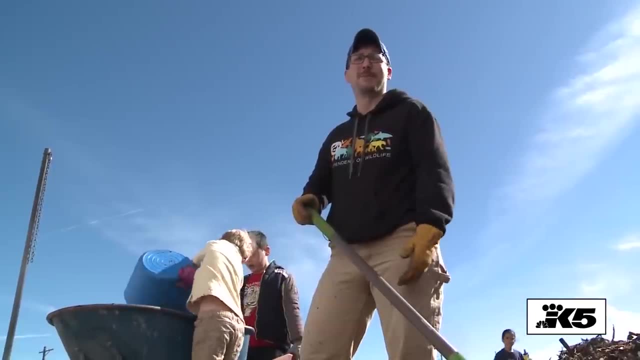 All of these students are going to become the next generation of leaders in Tacoma and Washington, And green stormwater infrastructure is a low cost and, in my opinion, common sense thing to do to reduce our impact on Puget Sound salmon and orcas. 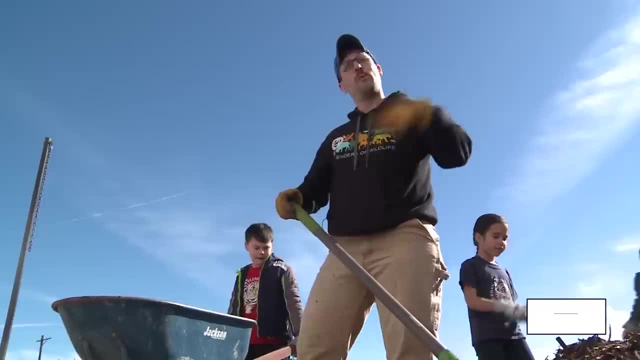 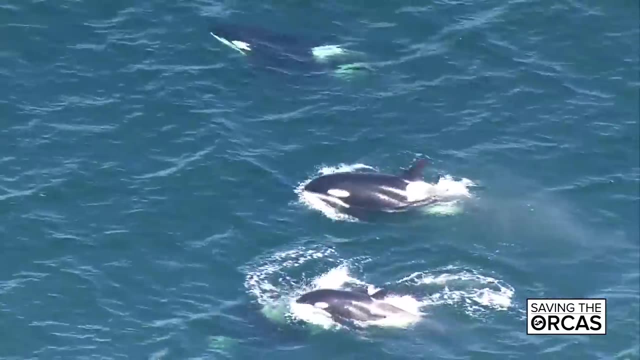 So it's important to get these kids to start thinking about how what we do up here on land is connected to what happens in the ocean as soon as possible. Protecting orcas and their habitat may seem like a lot of work, but they seem daunting, like an insurmountable challenge. 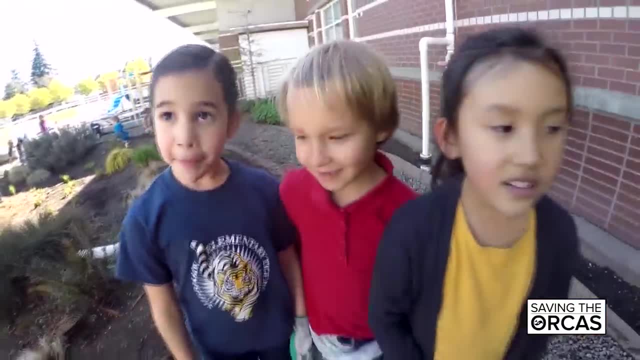 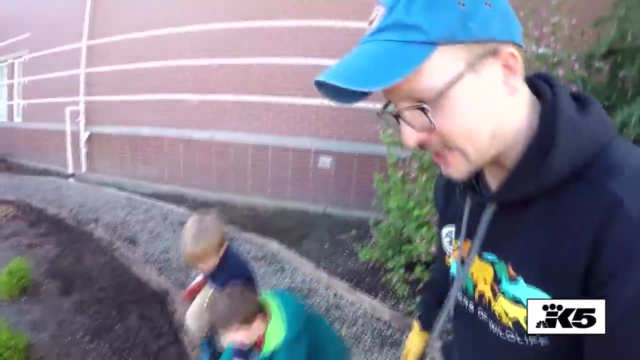 Would it make you sad if they disappear? Yeah, Because orcas look so smooth and pretty. But if we can learn anything from these students, Alright, you guys, spread that out, make it look good. It's that working together is the best way to start.